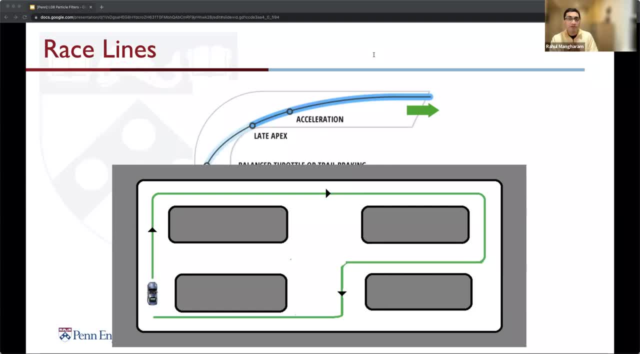 the car should be aware of the paths before and after the turn to choose the optimal path and manipulate its speed accordingly. In several cases, it's not just of all optimizing the turn the car can have in the present view. the decision should be smart enough. 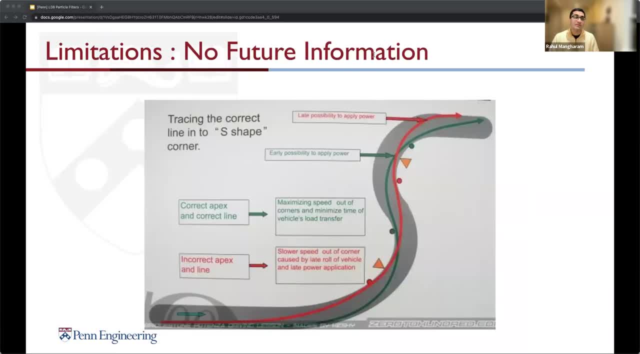 to choose the race lines depending on the next turn as well. as shown in the image here, you have two possible paths: the red and the green part. both follow the optimal path at the first turn. the green part is the most efficient one in order to optimize the second turn as well. 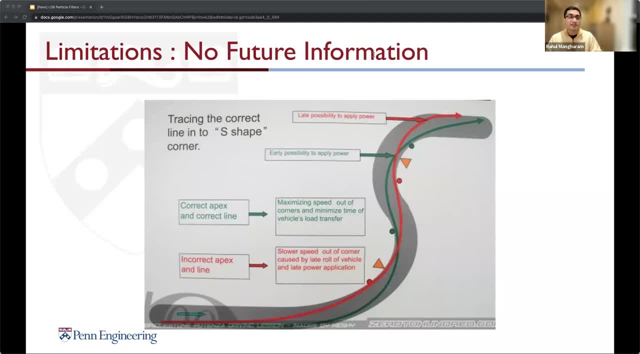 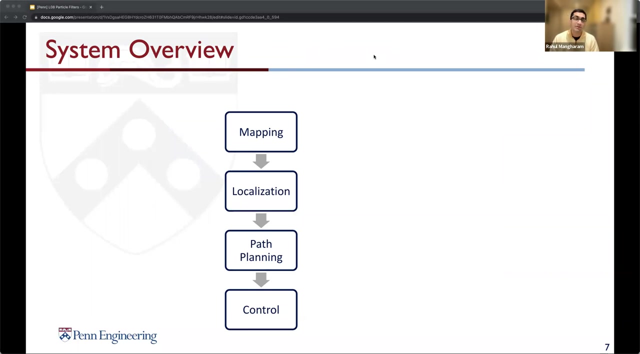 the path selection is heavily influenced by the remaining track. under such scenarios, all of this can be easily achieved if the cars have future track information while making path decisions. well, even the formula one drivers are aware of the track before they start the race. over the next few lectures we will talk about how we go about mapping the racetrack. make the car 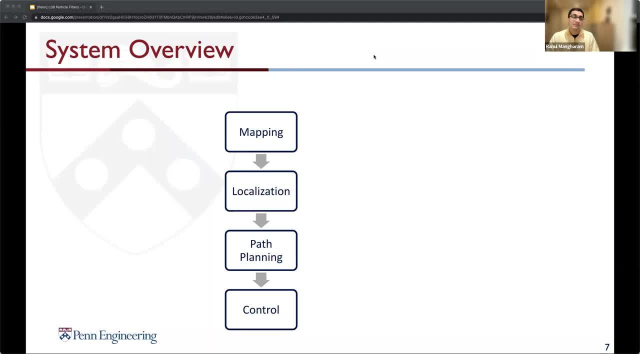 smart enough to perceive the surroundings and localize the track in the right way, as within this track. we will then talk about how to combine both mapping and localization to generate trajectories and then follow them to compete in the next race. to begin with, let's go through the concept of simultaneous localization and mapping. 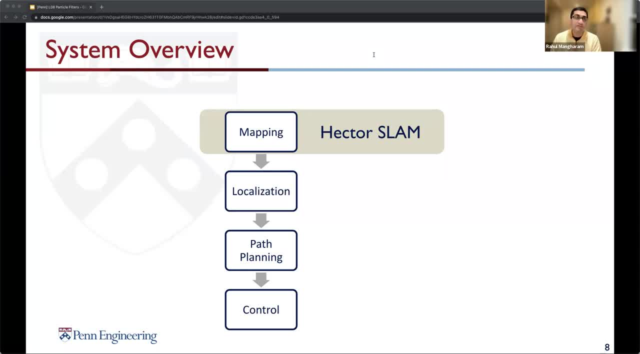 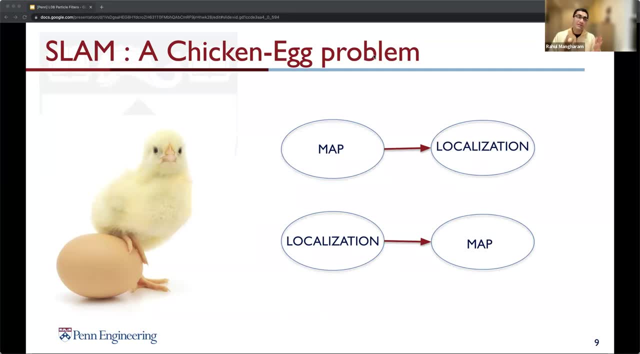 also known as slam, and we'll use a particular flavor of slam over here called hector slam. slam is often considered a chicken egg problem. you need a map of the environment to determine the robot location, but you need the robot's location first to build the map itself. 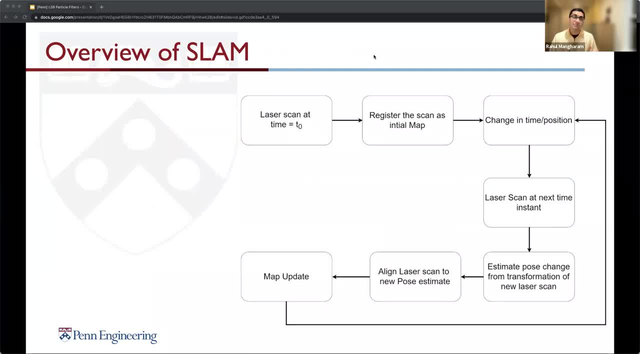 the way slam works is you register your initial map from the first scan and the initial pose estimate. the car then moves by a minor amount in a small time interval. now we have a new laser scan measurement and an estimate of the car's motion. the current laser scans are then correlated with 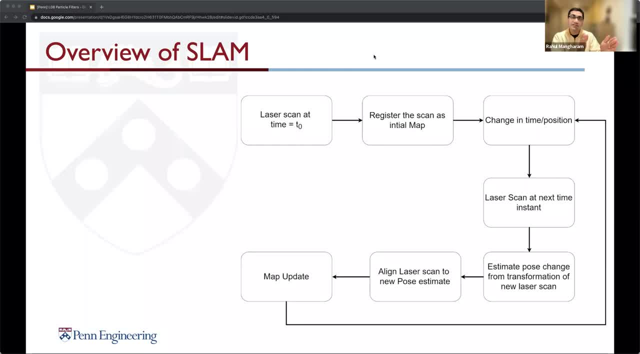 the map observed till this stage to estimate the change in the position. this way, at each stage you get a new pose estimate with which we update the map. this process continues several times over several time samples, updating the map at each step and this gives us an entire map. we won't go into the loop closure aspects today, but this just. 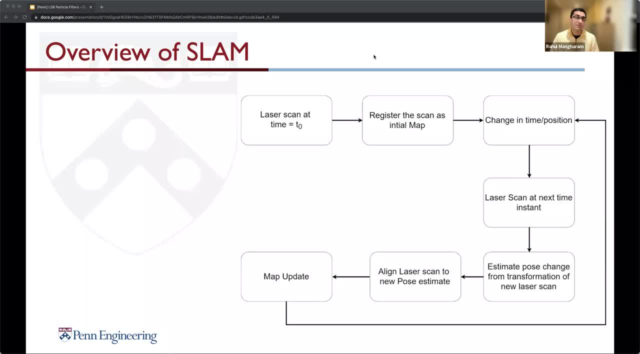 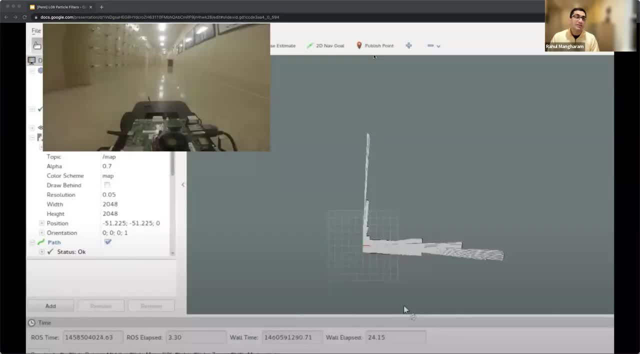 shows you a step-by-step manner in doing both the map map observation and the localization. so let's see the mapping generated by the car. this looks pretty simple, right? so let's delve into it further and analyze it. at the implementation level, there are a number of ways in which we could have. 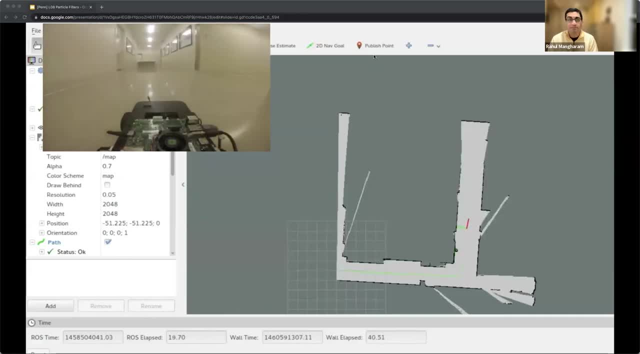 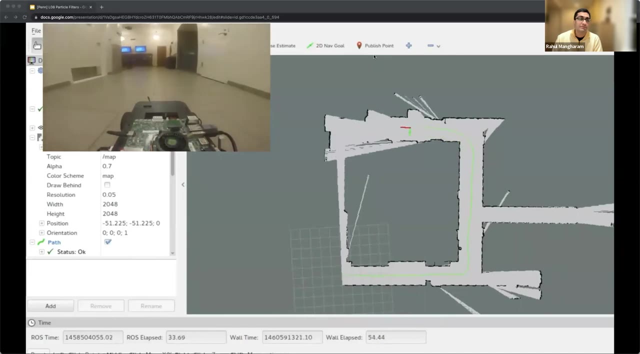 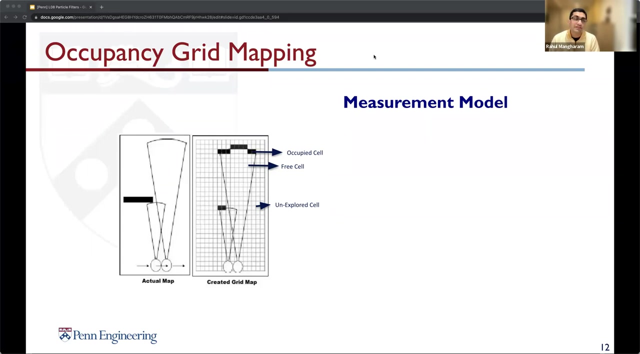 approached this problem and there are loads of research articles comparing them. we will talk about an approach centered around the ross package called hector slam, and you will be using this on your platform. the map we build here is an occupancy grid. as you see in the image, the occupancy grid is nothing but. 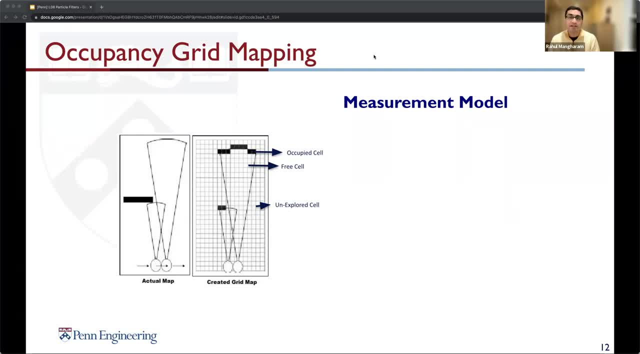 a standard grid where values of each cell indicates if it's occupied, if it's a free cell or an unexplored cell. the cells where we get confirmed lidar hits over several iterations are considered occupied cells and they build the walls or the occlusions from the map. the map is a. 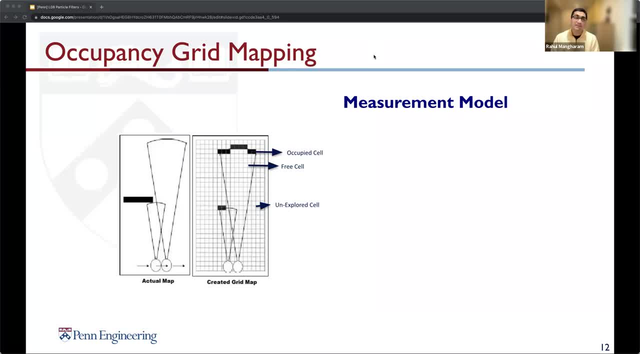 free cell. the cells considered as free cells are the ones where the lidar scans had a chance to pass through but did not get blocked or bounced off any obstacles. and the third type obviously corresponds to the cells where the lidar scans have never been able to explore anything. now. 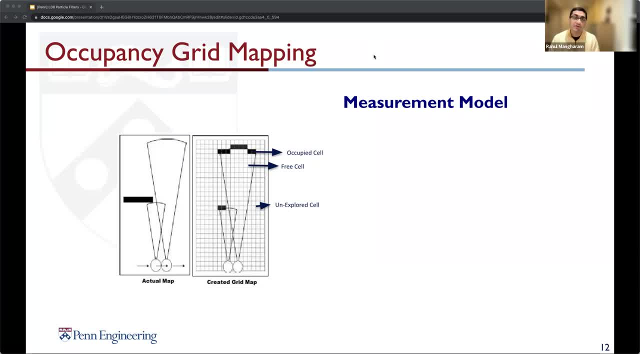 when we place the car into this occupancy grid. the lidar hits need to be ported to cell values. we maintain a separate database of laser measurements corresponding to each cell value. so the cells that are being occupied in the cell state can't be deployed in the cell state. 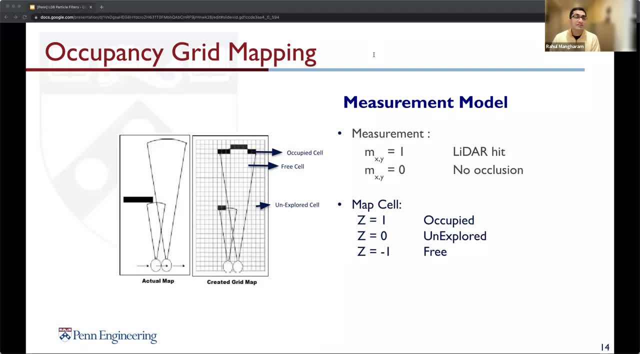 we consider these measurements as one for a coordinate where we have a lidar array, endpoint zero. for coordinates between the endpoints of the car and the car, the cells in this occupancy grid correspond to one minus one or zero, depending upon the cell state, whether it's occupied. 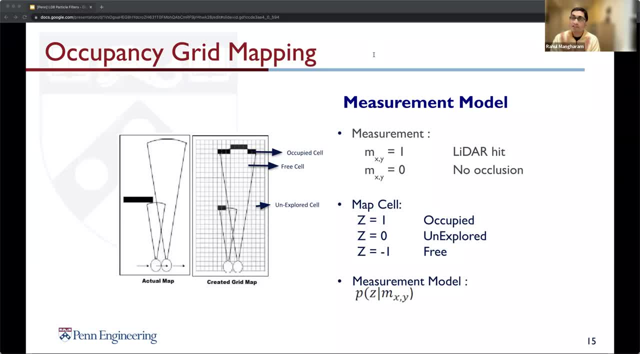 free or unexplored being 1 or 0, which indicates the estimated uncertainty in the LIDAR data. LIDAR measurements can be pretty accurate. However, you might not want to trust them completely, as you may have people moving around while we are mapping. 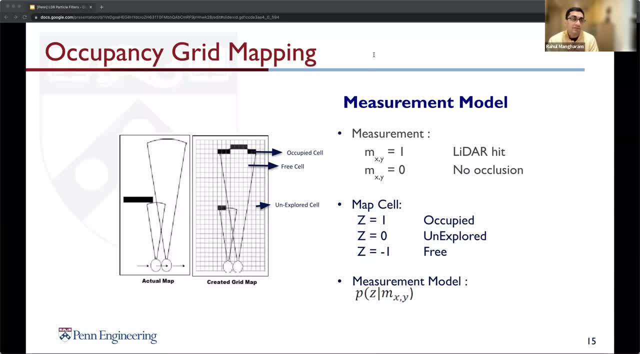 the environment. Now, for each given laser scan, the probability values for each cell the LIDAR scan passes through will be less than 1. And hence the accumulated probability would jump quickly to almost 0 and make no sense. To avoid this underflow, we deal with the log probability. 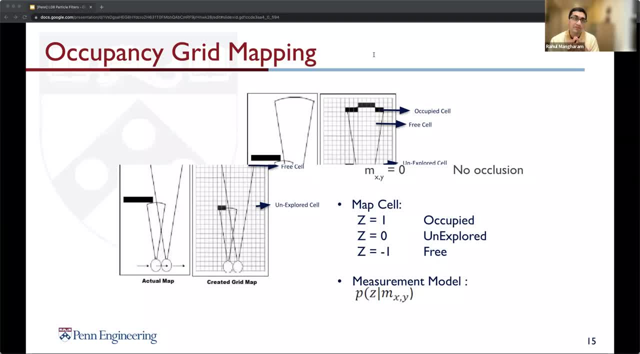 You see two equations over here. One corresponds to the log odd probability of occupied cells and the other one for free cells. During each time step we update the robot pose and map these constants to the particular mapped cells. This tells us the odds of a particular 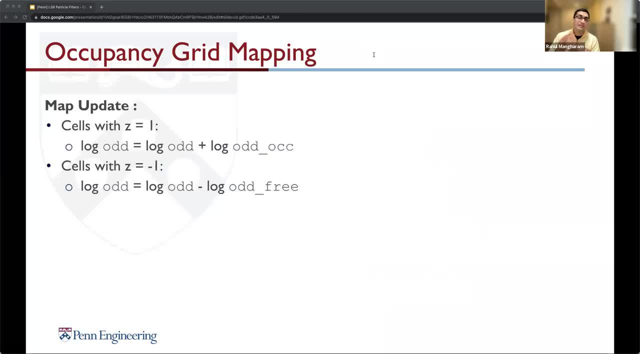 cell being occupied or free. We keep adding these constants for each cell over iterations after scan, after scan of the same region, to determine the confidence level of each cell. In robotics it's a general rule that you deal with unexpected noise sources And hence you should never be completely 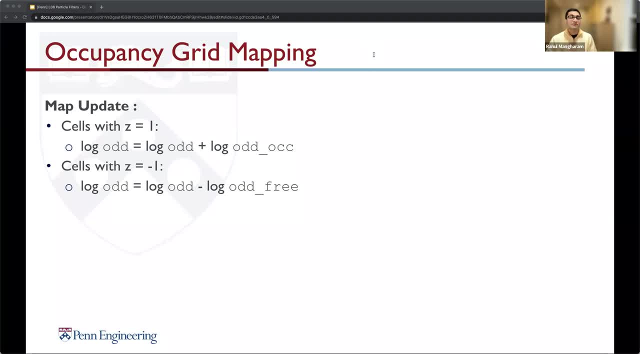 certain of your observation. There is always an element of uncertainty And therefore we have a very probabilistic view of estimation. Now, as we mentioned, we keep adding the constants to the cells to accumulate the confidence level if the cells are free or occupied. 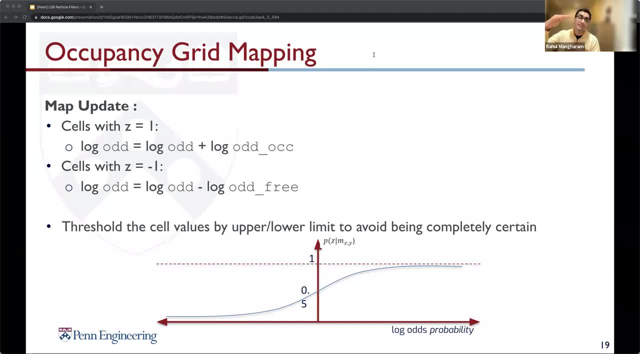 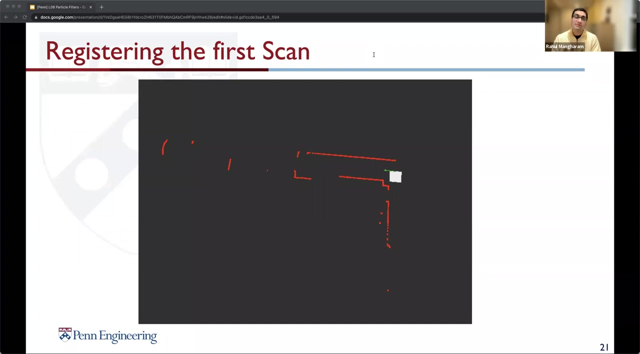 To avoid being completely certain, we saturate the cells with an upper and lower limit So that, if updated due to noise or unexpected moving surrounding features, the future measurements can bring it back to the corrected state. Now, when you start building the map, 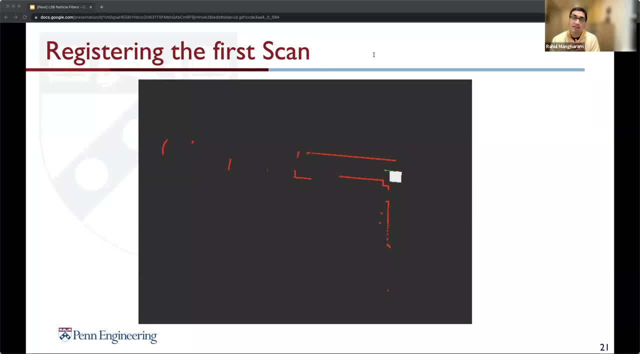 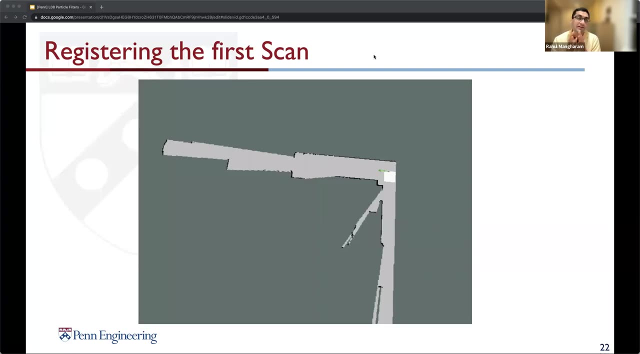 you take the initial pose of the robot as 0, 0 and update the map cells, taking in the first laser scan. For example, if this image is a scan at the initial stage, this is how the map registration will look like. This is our very first scan in this location. 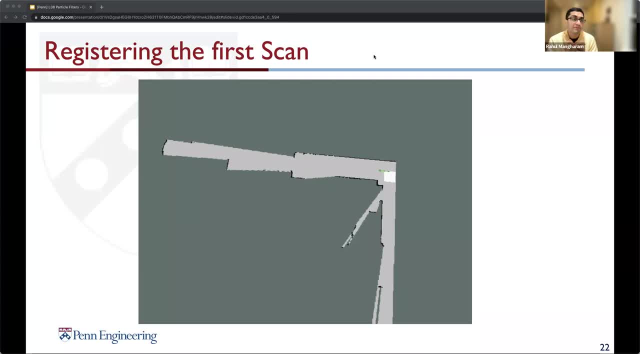 The initial map is directly updated by using the log probabilities for occupied and free cells a bit further. our goal is to find the pose change with respect to the previous measurement. We do this by finding the transformation between the new laser scan and the previously registered map. 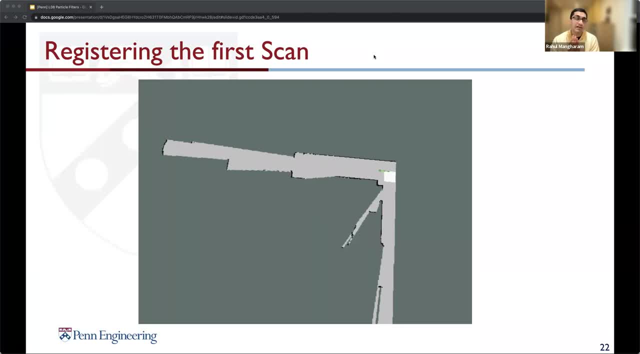 We cover scan matching in the previous lecture and will review it briefly in the context of map making over here. As you can see here we have a scan at time: instant t equals t1. The robot moves a small amount and makes a left turn. 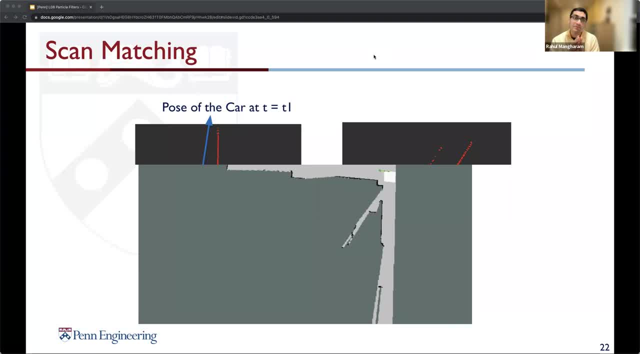 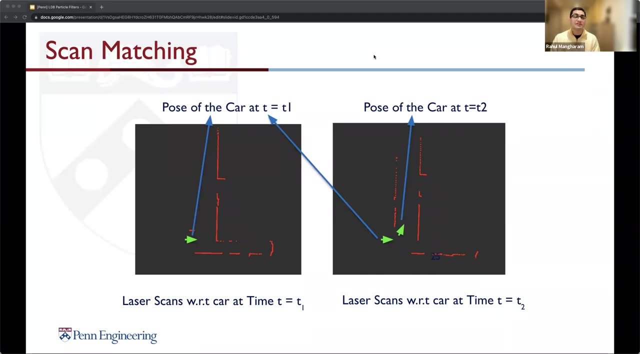 The laser scans as viewed from the robot frame at time t2 look like the second image on the right. Scan matching will allow us to find the pose change between these two timestamps and align the scan at the second time instance with the first scan. The change in pose measured with this approach is used to maintain the robot pose while updating the map simultaneously. 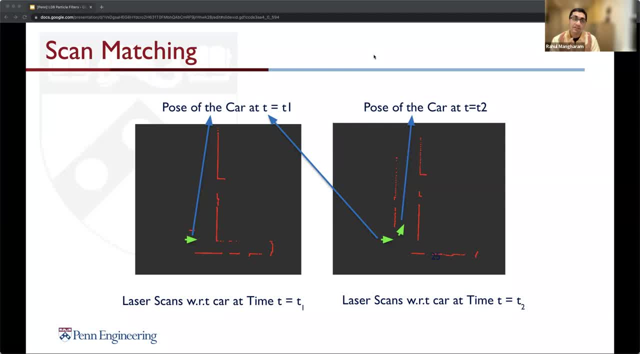 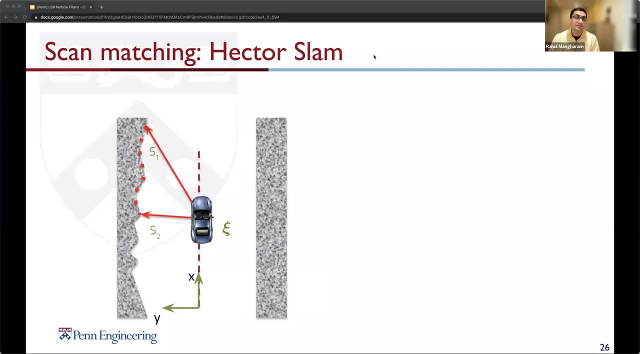 The laser scans we get are point clouds which give us information about the 2D map of the current environment around the robot and within its scanning range. Let's see the approach taken by Hector Slam to find the transform between two consecutive scans. Here the symbol psi i represents the pose of the robot. 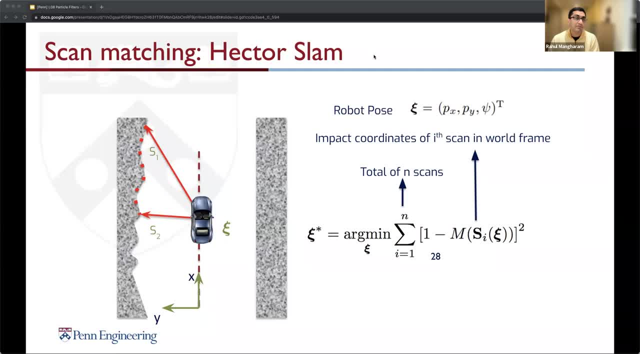 The function si, psi, i represents the end coordinates of the item And the function m gives the value of the map cell at the particular scan coordinate. As we noted earlier, the map cells correspond to 1, minus 1, and 0.. 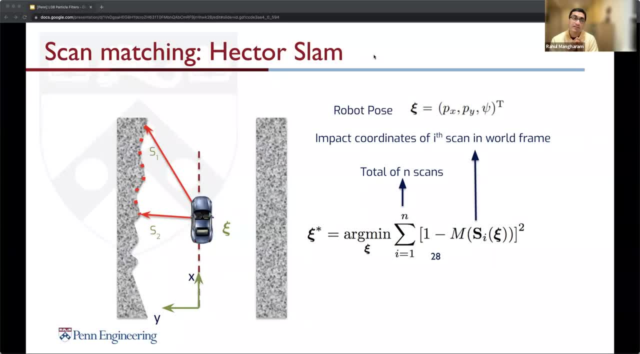 Because this correlation is done over occupied cells, we can mask the negative values to 0. The equation here suggests that the term within the brackets is 0 for a point i where the map cell value is 0. Thus when we scan each point, it corresponds to the cell having a value of 1.. 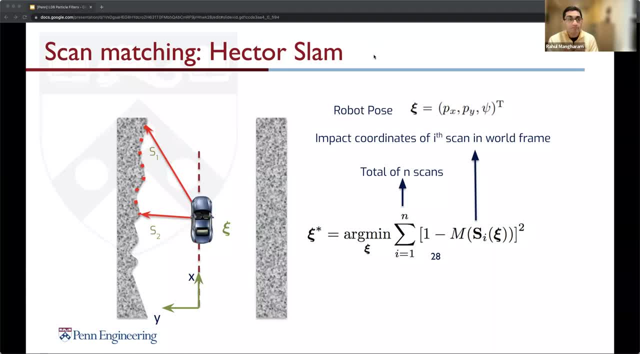 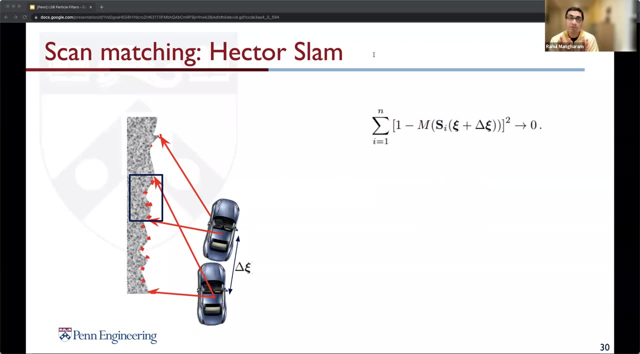 The summation will result in a 0 value. For a normal case, where we do have certain uncertainties and minor errors, our goal is to minimize this summation. The pose function, psi i, can also be written as a summation of previous pose and the change in the pose in the small time interval. 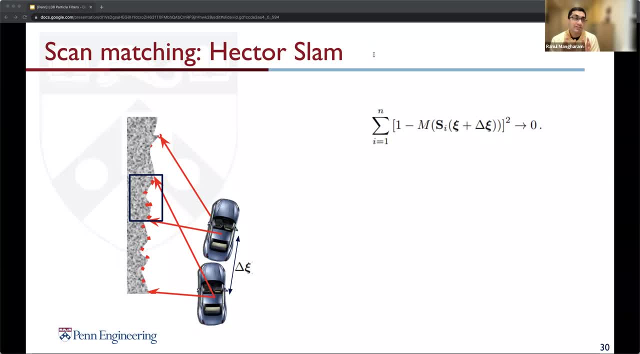 This now changes the minimization function to a function over change in pose. We expand the equation using the Taylor expansion for function m. Solving it for delta psi. i gives us the Gauss-Newton equation for delta psi i, evaluation of which gives us a step change in the pose with respect to the previous timestamp. 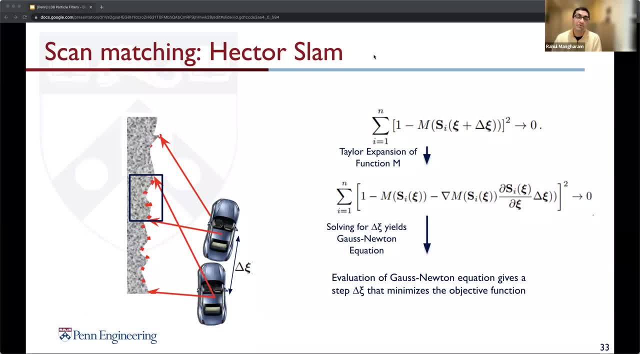 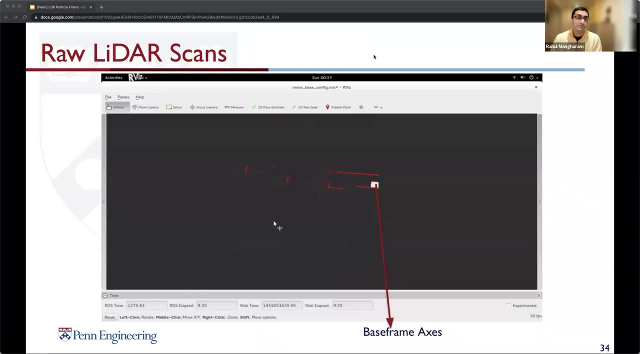 Now this operation will give you the change in the pose. at each time step. We update the pose with the calculated pose change. transform the current laser scans to the new pose. The map is then updated using the transformed laser scans. The video here depicts the way in which you get the LiDAR data in the car's view of the world. 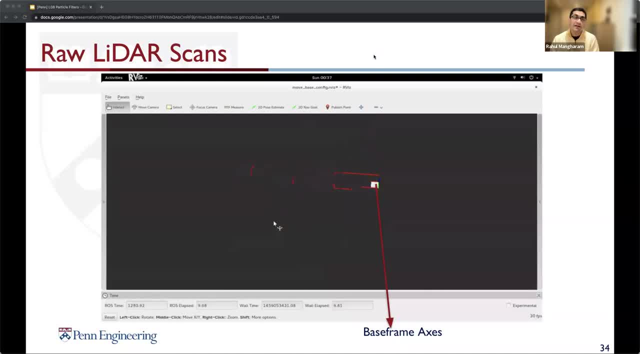 The Hector scan matcher will take this data, match the scans between the two timestamps while registering the map, and then update the car pose at each stage. Now the video here shows the LiDAR scan when it's viewed from the map frame. 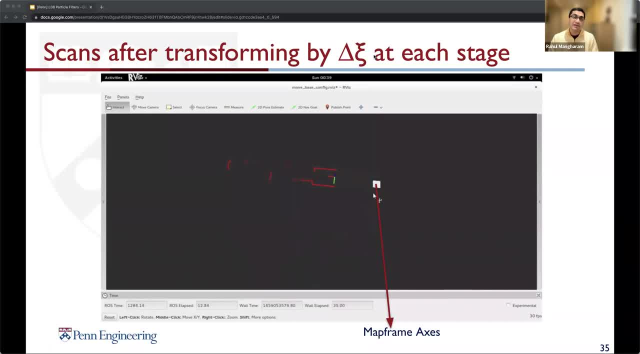 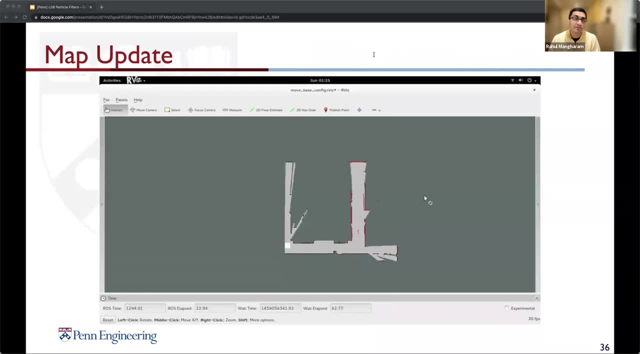 The change in pose estimated is evaluated at each stage to calculate the new pose, and scans are being aligned to the new pose. The map registered in this video that we just saw would look like this: We observe that once we have the change in pose estimated. 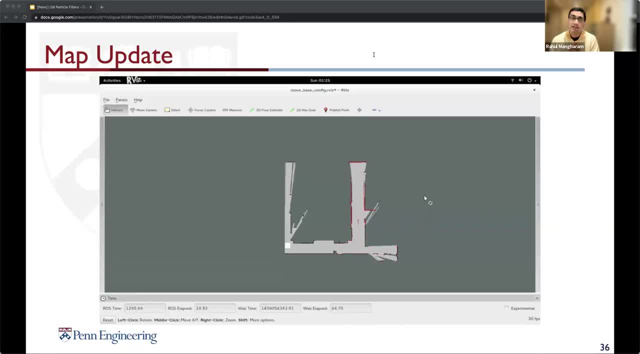 we transform the scan to the global frame and then update the global map with these scans. However, the occupancy grid doesn't assign a wall or a free space directly by observing in a single scan, as it might introduce a lot of noise. Observe this video carefully. 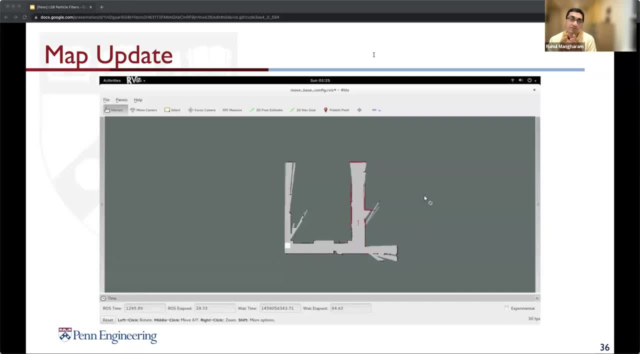 Apart from the binary occupancy grid visible to us, the algorithm also maintains a value for each cell. This value is a function of the number of times a cell is encountered during the scan. The number of times a cell is encountered during the scan is determined by the scan as free or occupied. 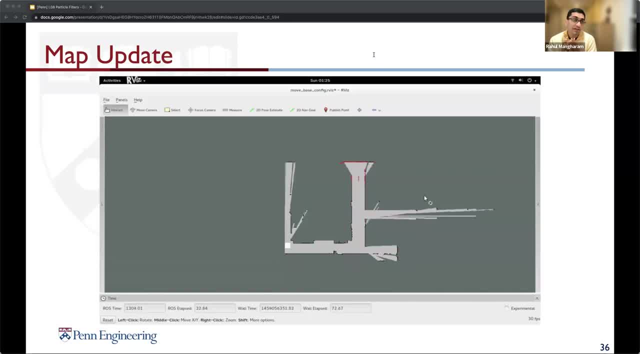 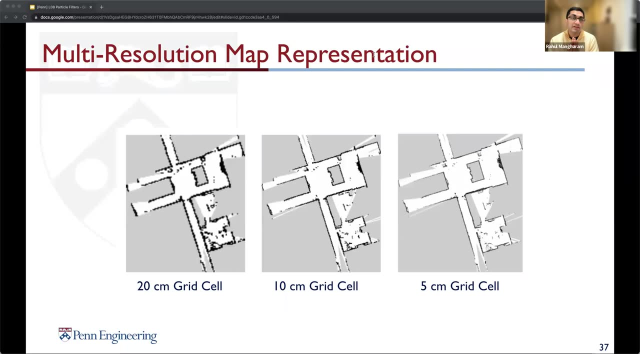 and the probability of scan measurement being correct. Thus, after every few laser scans, when the map is confident of a particular chunk of cells being free or occupied, it gets published as the occupancy map. Now, in this kind of optimization functions there's a high possibility of getting stuck in local minima. 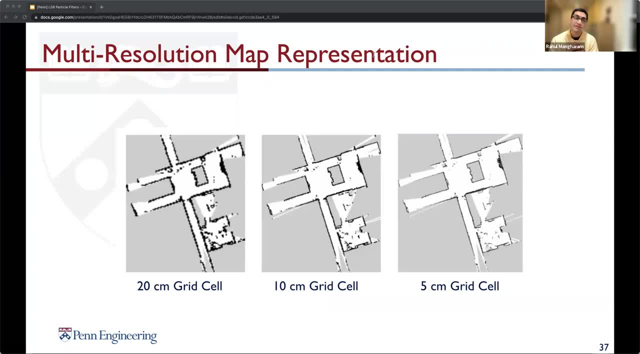 In order to avoid this, rather than using a single occupancy grid, the equation is optimized first over coarser maps to find a pose estimate. The estimate is then used as an input to the optimization function over higher-resolution maps, If we provide the resolution of 5 cm as the input to Hector's SLAM. 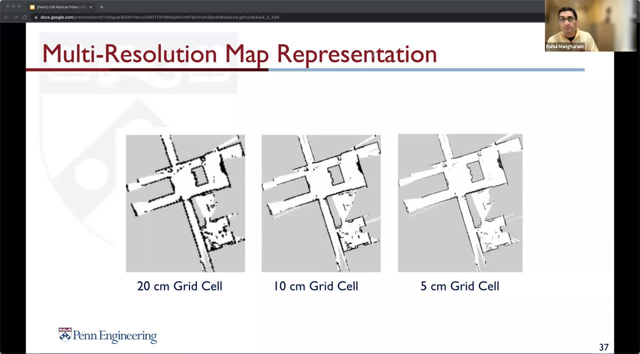 and we have decided on using three multi-resolution grids. the algorithm will iterate over the grids of resolution: 20 cm, 10 cm and 5 cm. The pose update from the 20 cm grid will be and input to the process over the 10 cm grid, and so on. 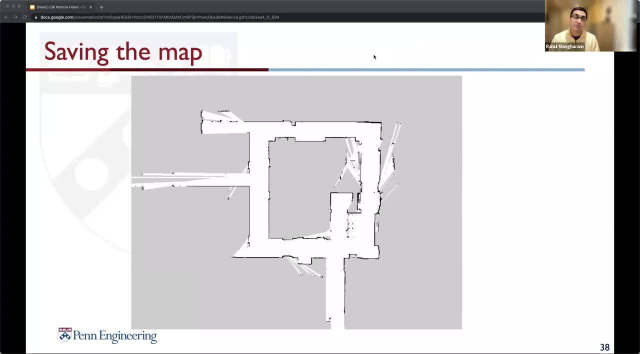 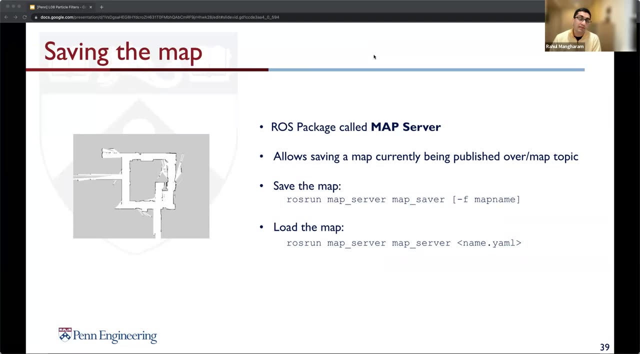 The map generated here is now a base for further algorithms of localization and planning. It is essential to save this map and be capable of loading it later. The ROS package called MapServer provides this functionality: to save the map and then to load the map using just this ROS, run MapServer and save the map. 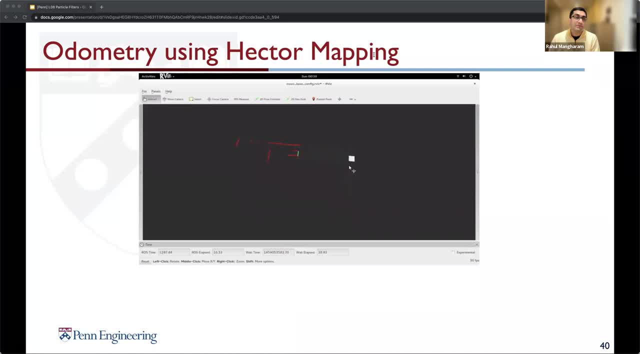 So, coming back to pose updates, during Hector's SLAM we get a change in pose during analysis of the laser scan at each timestamp and thus a source of odometry Ignoring the map being generated. we can actually use the Hector's SLAM package. 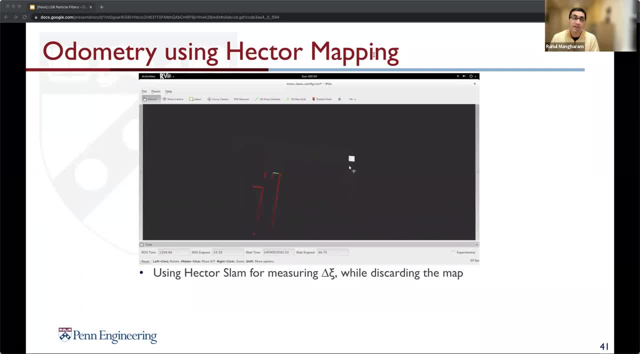 to get a source of odometry information obtained via scan matching. You can also consider using the canonical scan matcher package for the same task. Both these approaches give odometry information. The main difference is Hector's SLAM calculates the change in the pose by matching the current LiDAR scan with the map generated during the previous timestamp. 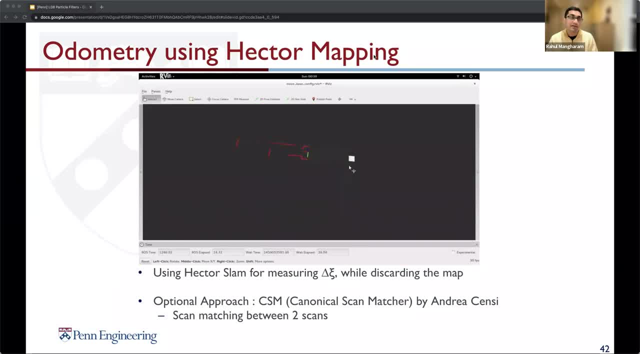 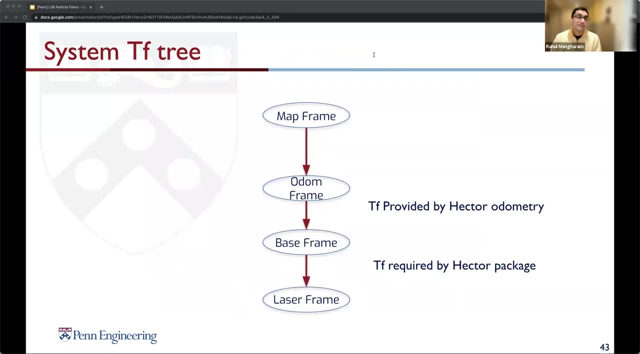 whereas the CSM package or the canonical scan matcher package, as we studied in the previous lecture, that's developed by Andrea Sensi, does this by correlating the current scan with the previous scan and not the map. You've seen the TF tree diagram in previous lectures, haven't you? 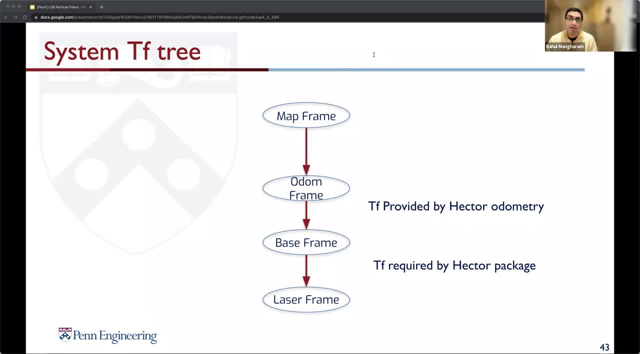 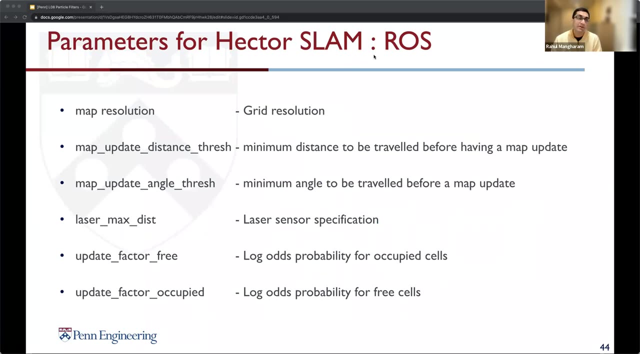 This is the transform tree for our system. once the localization algorithm is implemented, The Hector odometry provides a transform between the odometry frame and the base frame. Now you will use this package in ROS and you will come across several parameters. You can go through the website on Hector mapping a package- to read about them in further detail. 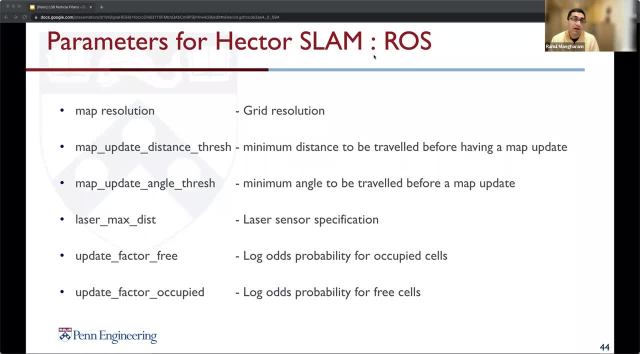 The map resolution parameter allows you to specify how fine you want your map to be. The next two allow you to specify the distance or the angle threshold by which the robot should move between consecutive map updates. The default map laser scan set in this package is 30 meters. 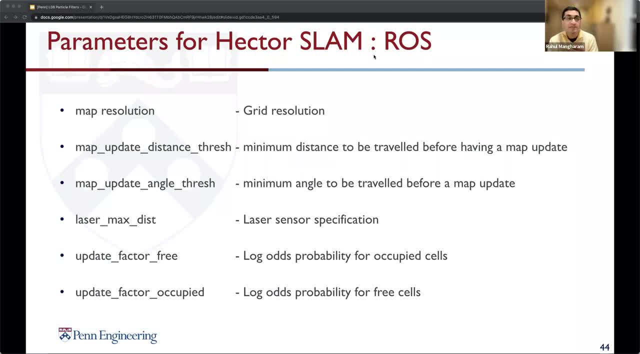 but the LiDAR you'll be using has a range of 10 meters. The last two parameters are the log-odd constants of the occupied and the free cells we talked about during the map update stage. In the SLAM tutorial. we will walk you through installing the package. 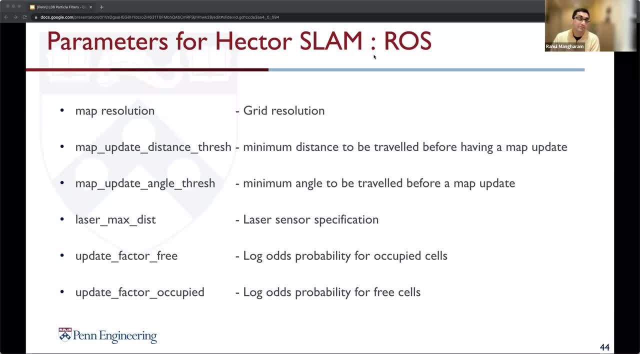 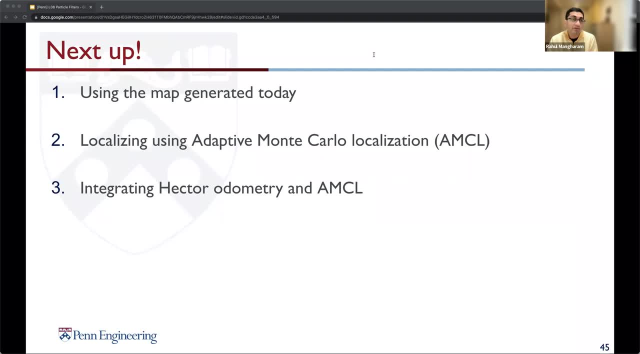 and using the basic launch file for your application. In the next section, we will go over the concepts and implementation details of the adaptive Monte Carlo localization and show you how to integrate the map and odometry we generated today for the localization package. In the previous section, you saw how to build a map of the surroundings using Hector SLAM. 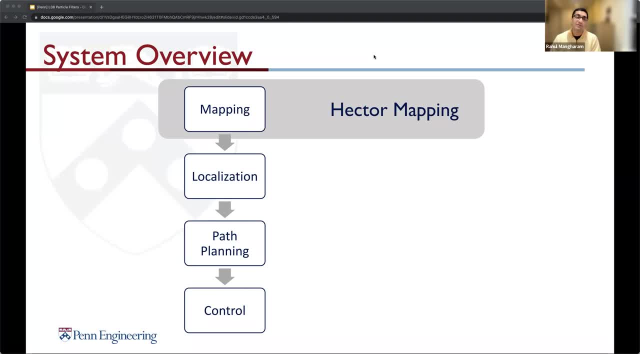 and also how to use Hector SLAM to build a map of the surroundings using Hector SLAM, and also how to use Hector SLAM to build a map of the surroundings using Hector SLAM, as well as how to use Hector SLAM to build a map of the surroundings using Hector SLAM. 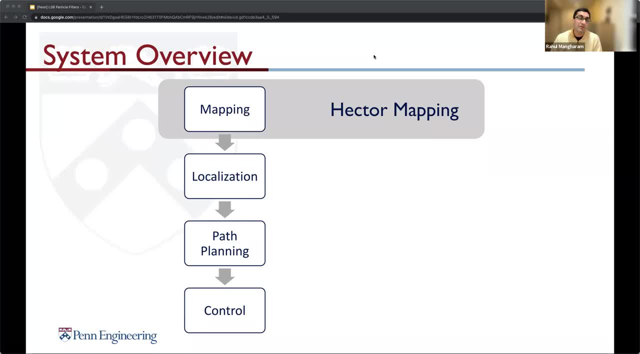 Now that we have built the map, we'll go to the next task, which is to know where we are in the map accurately. It's crucial to know where we are to decide where we need to go. This helps us plan the trajectory that we should take. 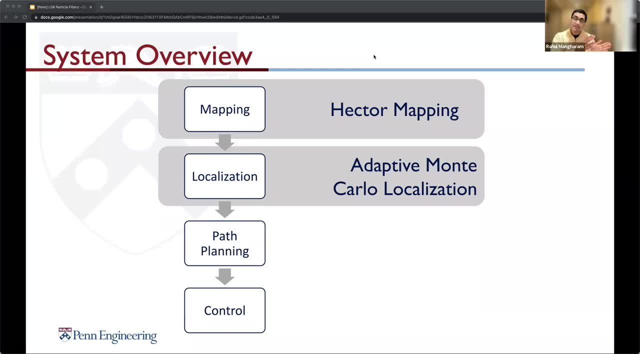 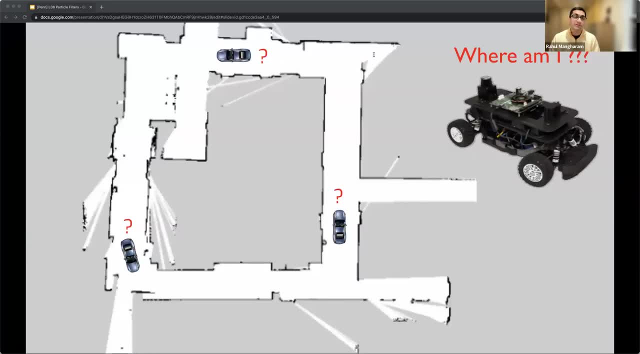 based on the upcoming corners, and also make precise control decisions on the speed and race lines. That way, we can decide at what speed we need to approach the corner, based on how sharp the turn is and how far we are from the race line. Another piece of crucial information that we need to know is our orientation. 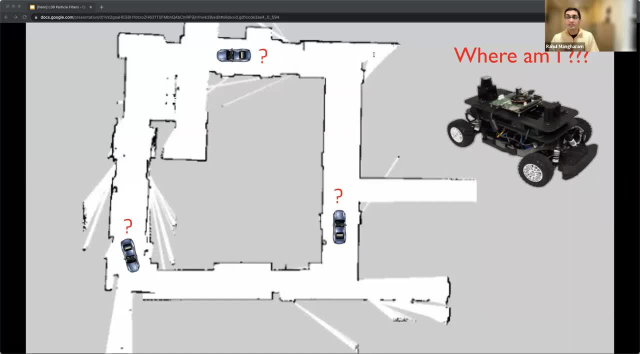 or heading in the map, so that we can decide on the correction to be applied to the steering to take evasive actions against collisions with the wall or obstacles In general. knowing where you are helps us decide what we need to do next. Hence we need our car at all times to precisely. 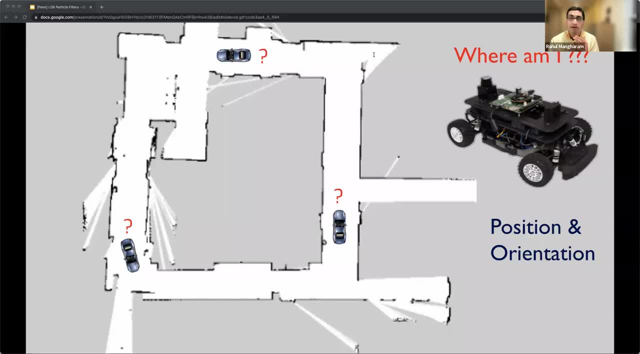 locate its position and orientation in this map, with or without knowing the original initial position. Localization involves estimating the position and orientation of the vehicle, collectively called as a pose, as it moves and senses through the environment. One way of knowing the position of the car is by tracking, from its initial position, the amount. 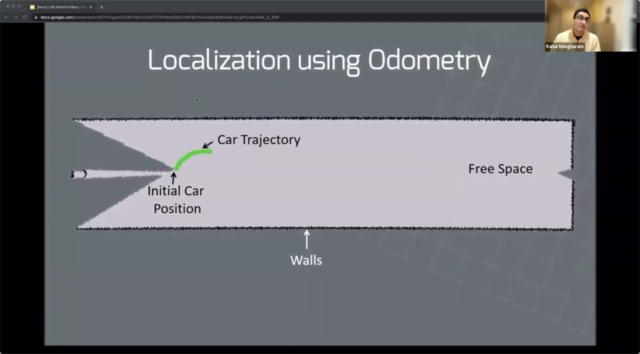 of distance it has traveled By measuring the number of rotations of the left and the right wheels. using wheel odometry that we saw in the previous lectures, we can calculate the distance traveled from an initial position and predict with some certainty about the car's pose on the map. 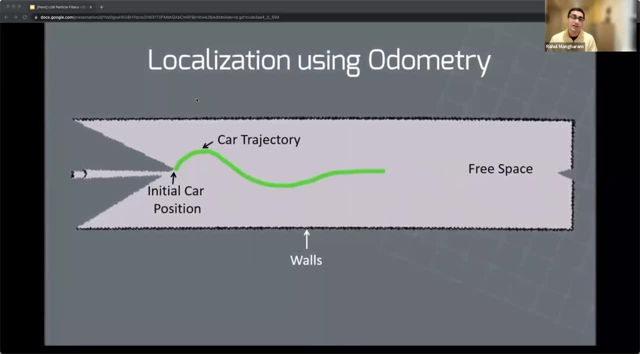 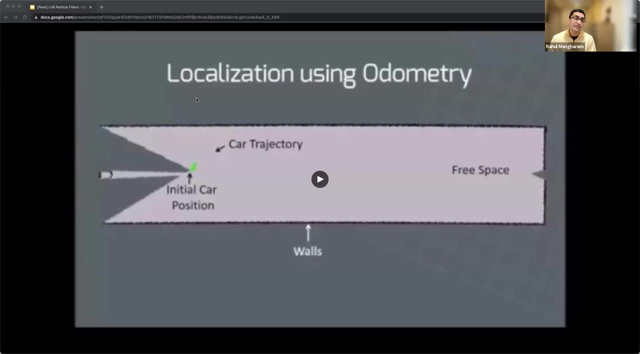 Here, the green dot is the initial position of the car in the corridor As it begins to move. the green path is the trajectory followed by the car as tracked by the wheel odometry. Similarly, even the odometry information from Hector's slant can be used for. 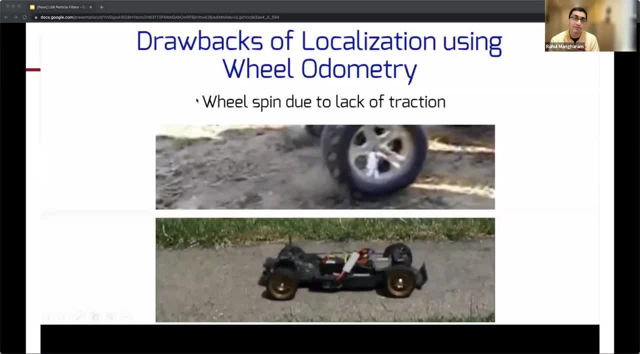 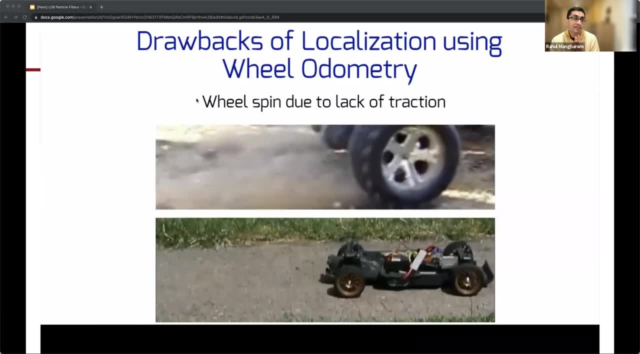 tracking. However, both these sources are not accurate sources of pose due to various reasons. First, the method of measurement itself is not accurate. Additionally, as it integrates distance over time, the error keeps accumulating. This causes odometry drift over time, So the longer 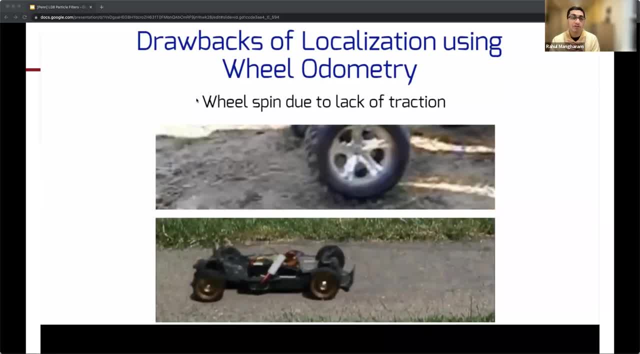 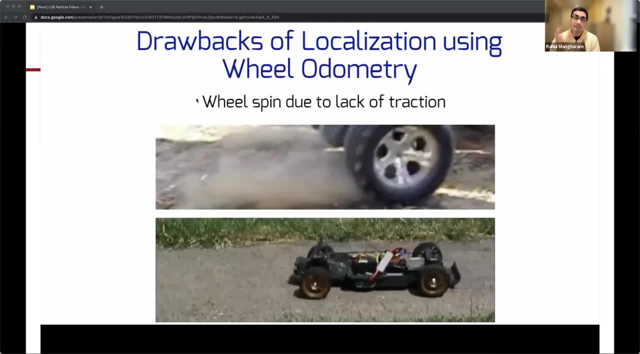 you run the odometry, the more accurate the odometry is. So the longer you run the odometry, the more inaccurate your position or your pose estimate is. Another problem with wheel encoder-based odometry is that it does not account for wheel slippage, as you can see in the video here. 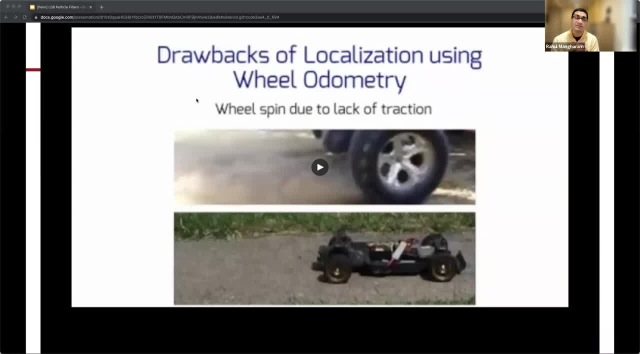 which is very common for high-speed platforms as this one. Due to the high torque of the motor, the wheels spin at the same location before the car starts to move, The odometry believes the car has moved a certain distance, even though the wheel is spinning at the same location. 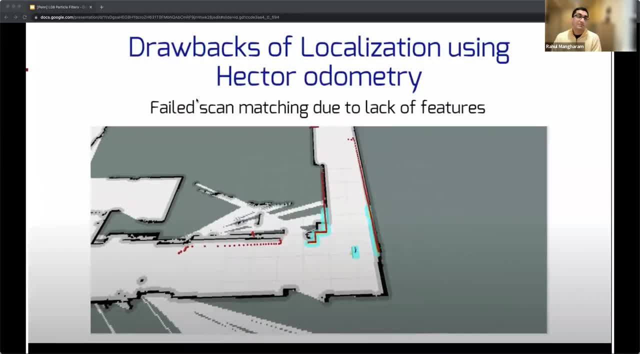 That is why it is very often soccer- could fall into collision focus mode. So from the performance gradient adjusting the odometry second location yields an incorrect pose. Similarly, when even odometry using Hector's slant, it suffers some drawbacks. The scan 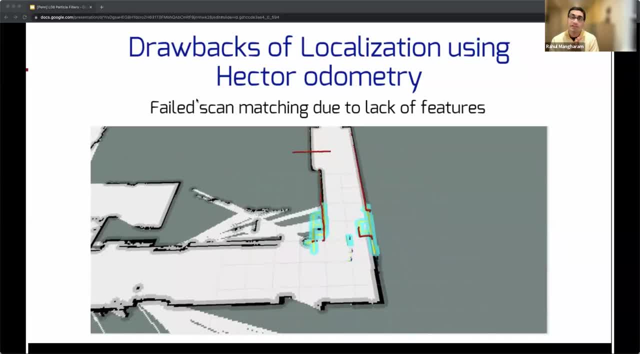 matching-based odometry fails when the corridor is very similar, as we have seen previously: Such a corridor with smooth, featureless parallel walls over short distances. in this video, you can see that, even though the car is actually moving and recording new scans. 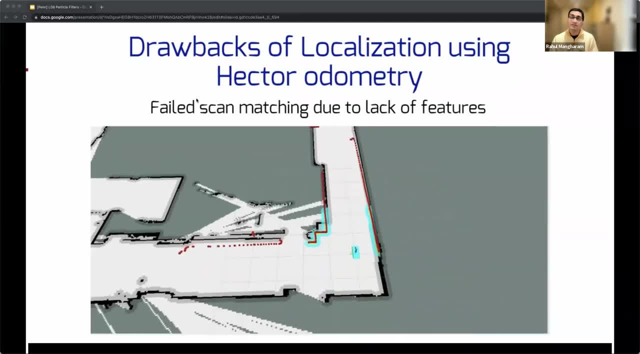 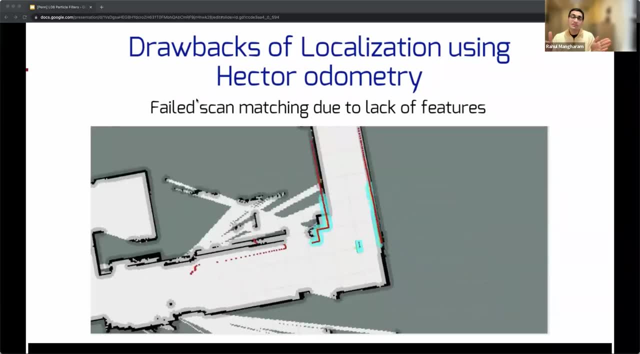 which are shown in red. the scan matching based odometry fails to record it because it scans with it, because the scans are very similar, and finally, it realizes only when there is a prominently different scan at the end, at the turn of the corridor. Hence we need a solution that can 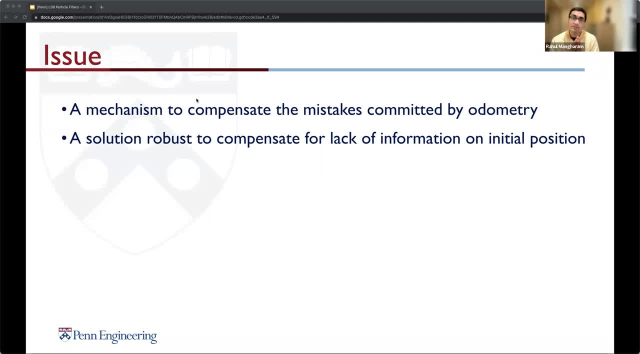 compensate for the accumulated odometry error, including those errors due to the measurement wheel slippage and failure of scan matching. Additionally, we must also be able to localize without providing an accurate initial position. In other words, we must be able to handle inaccuracies in defining the initial pose. One solution is to use Monte Carlo localization. 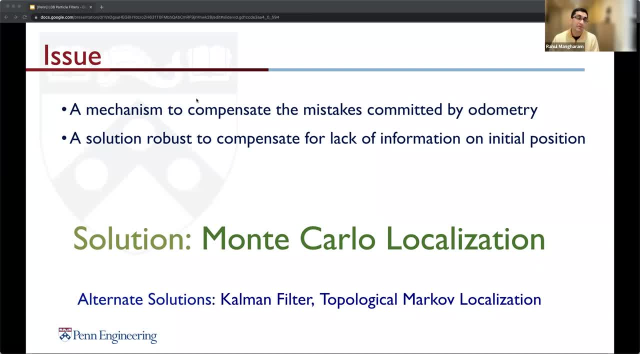 which uses particle filters. Other options to localize are Kalman filters, which use Gaussians to keep track of the position, and Markov localizations, which use histograms. We'll focus on the MCL based localization and also further understand how particle filters make this work. To understand about Monte Carlo localization: 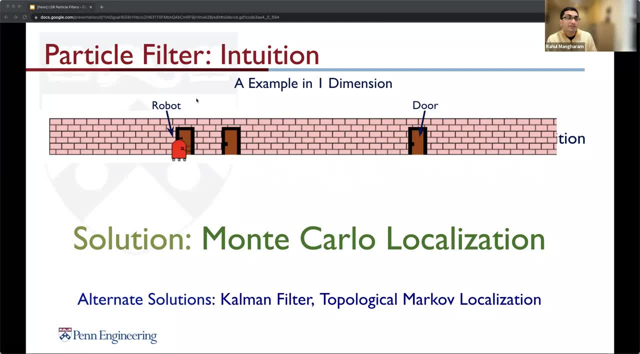 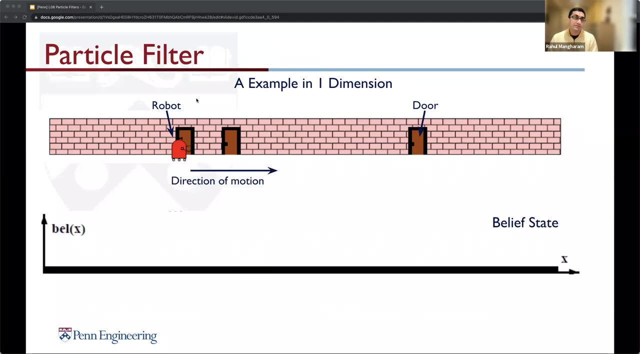 we first need to see how particle filters work right. So let's use an example of a robot where we can move. in one dimension, The robot just moves, you know, from left to right, or it can move the other direction too. The environment is the corridor with a few doors, The robot can move. 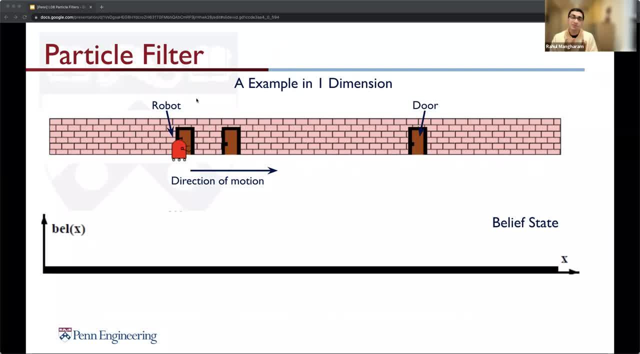 up and down the corridor. The robot also carries sensors to sense only the doors, And so it has this magical sensor that knows, okay, if it's next to a door- here is a door- And has a source of odometry that tells how far it has moved. Initially, the robot has no. 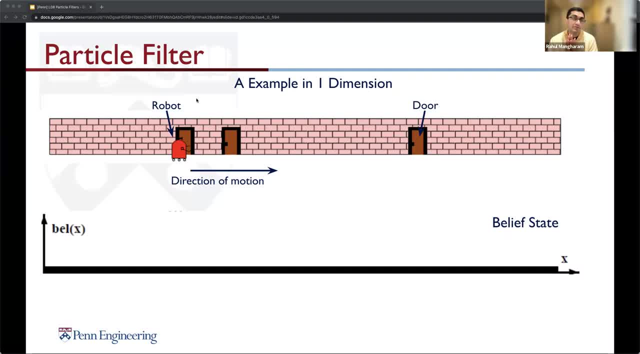 information on where it is in the map. The graph of the position on the x-axis versus the probability on the y-axis of being there is zero. We call this graph the belief state. It defines the probability of the robot being in that particular position, So we can model the robot's current belief about. 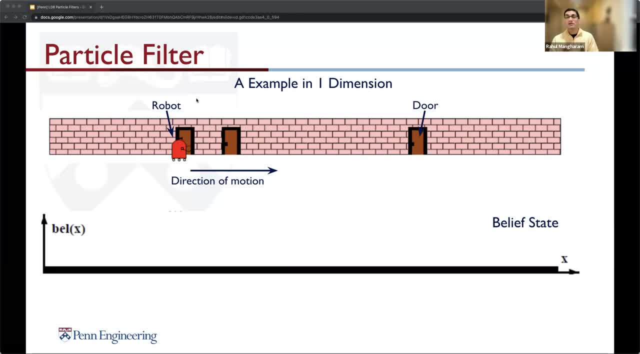 where it might be by its confusion. This is captured by a uniform function that assigns equal weight to every possible place in this world. This is a state of maximum confusion. at this point in time, At the first time step, the robot senses a door, So the probability of 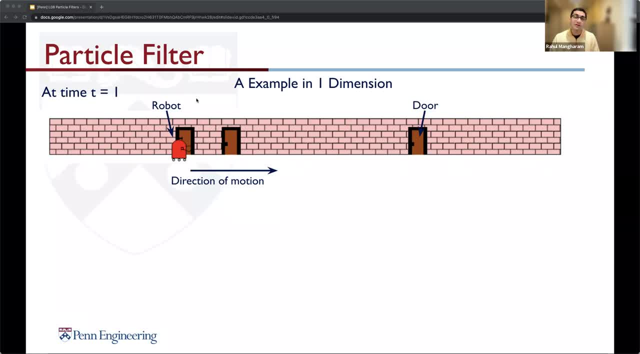 receiving this sensor measurement in the corridor is given by a probability p of z, given x, Where z is the sensor measurement, in this case if it's a door or not, and x is a position. We call this our measurement model, which denotes the sensor reading against position. 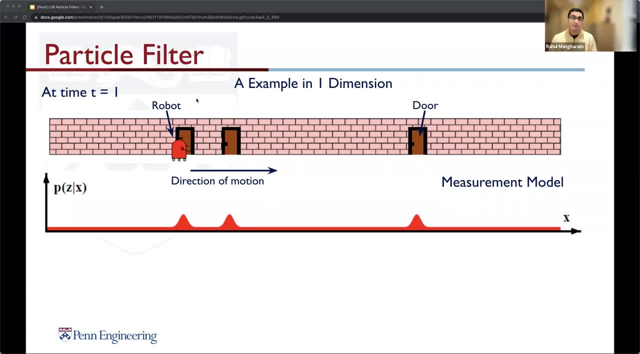 So all it knows now is that it is located likely next to a door. How would this affect our belief? Well, our belief state is where our robot is in the map and it has a particular, has a similar definition of belief. So it has a particular, has a similar definition of belief. 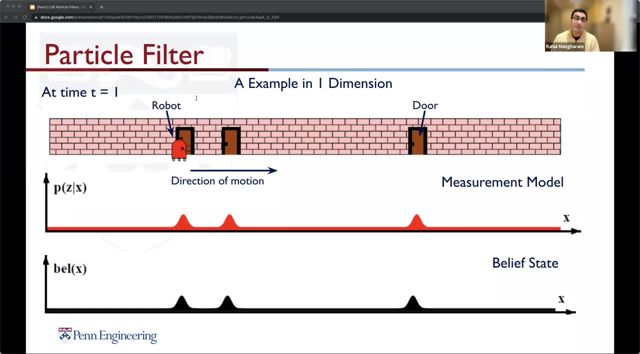 And by observing this belief distribution, the measurement of a door transforms the believing function defined over possible locations to a new function that looks pretty much like this: For the three locations adjacent to doors, we now have an increased belief of being there, whereas all the other locations have a decreased belief. 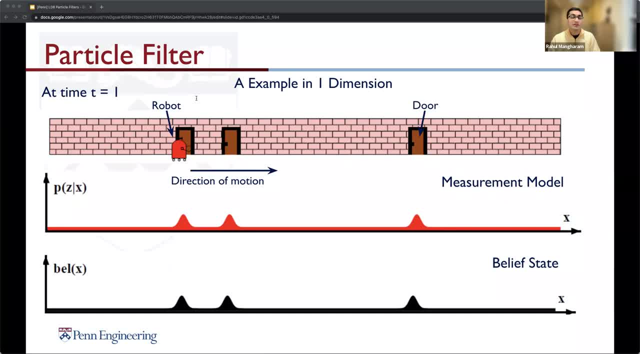 This is a probability distribution that assigns higher probability for being near a door and it is called a posterior belief of being next to a door and it's called the posterior belief by the world. Posterior means it's it's after the measurement has been taken. 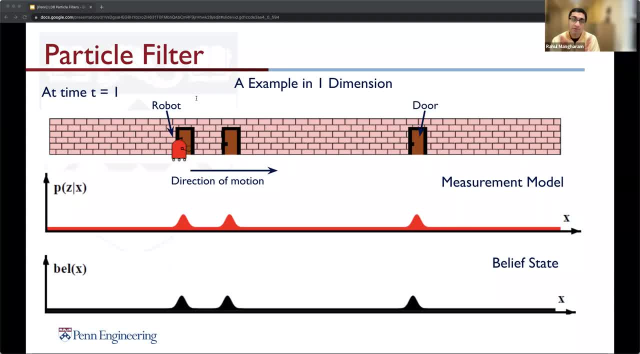 Now, the key aspect of this belief is that we still don't know where exactly we are And there are three possible door locations, And, in fact, it might be that the sensors were erroneous and we accidentally saw a door where there is none. 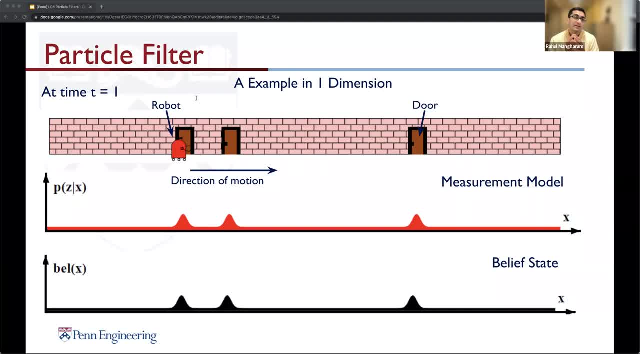 So there's still some doubt also about that. So there is still some residual probability of being in these places between the bumps, but the three bumps together really express our current best belief of where we are. This representation is absolutely core to probability and to mobile robot localization. 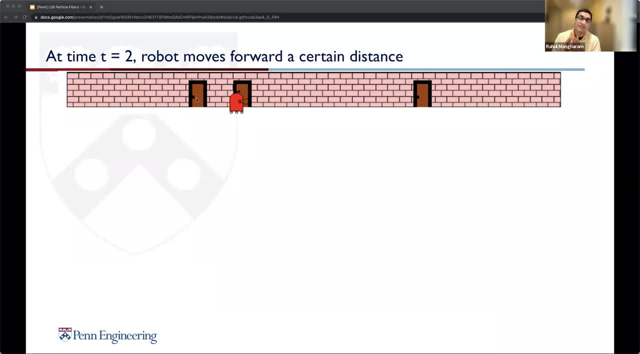 At the next time step. the odometry from the robot says it has moved a certain distance forward. So now we update our belief state by moving forward the same distance with some added noise to account for the error in odometry. This is called our motion update of the belief state. 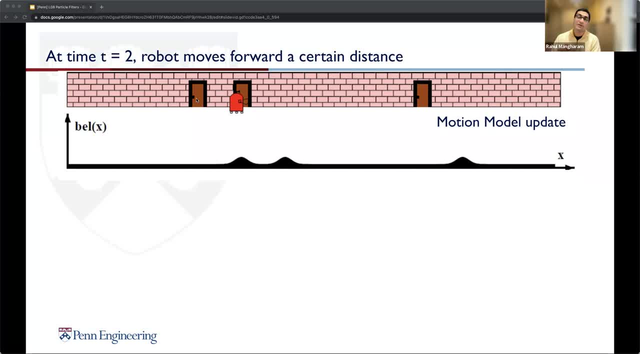 This is nothing but our previous belief state that has been updated with odometry information less shifted. Now the robot motion is somewhat uncertain And we can never be certain as to where the robot moved. So these things are a little bit flatter than the guys. 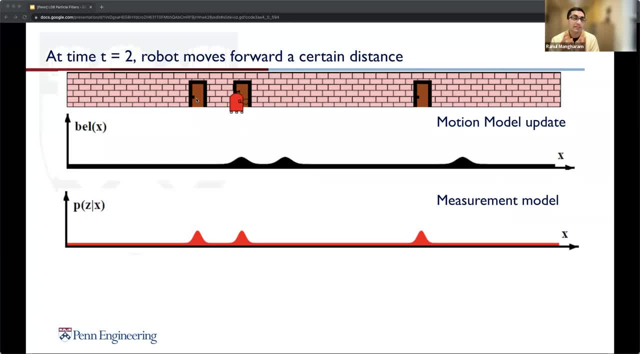 over there And we perform a measurement update by reading the data from the sensors. Again, we sensor door, Hence our probability of receiving the sensor measurement in the corridor is the same. So this is for the second door. So we get our new belief state. 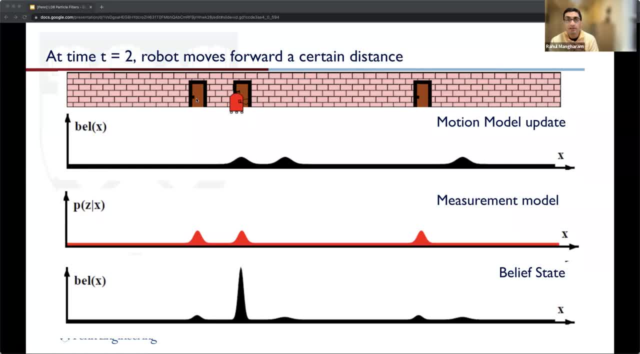 which has a high probability of being near door two. We end up multiplying our belief, which is now prior to the second measurement with the red function in the middle. That is a second measurement after the motion update. The outcome has a peak at each door. 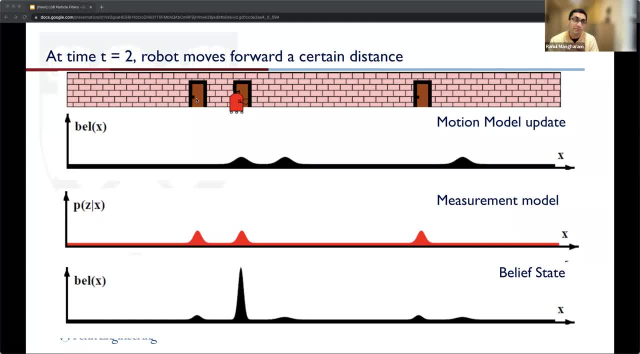 and outcomes: belief looking at the second door. So we get our new belief state, which is a higher probability of being near door two, And when young people are misunderstood, they collect that enough data from them thatity runs along the path of building the door. 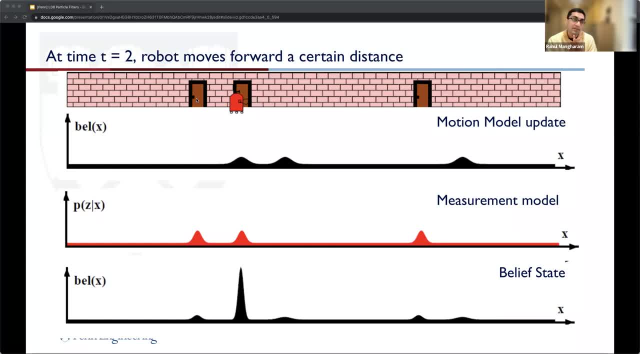 and that data is stored as part of the construction for the computer, Because two open doors sending us an action to change the direction of the physiology of a computer roof. it also reproduces the data to the operator or gentelector. Finally, it opens to any tweets of a notebook. 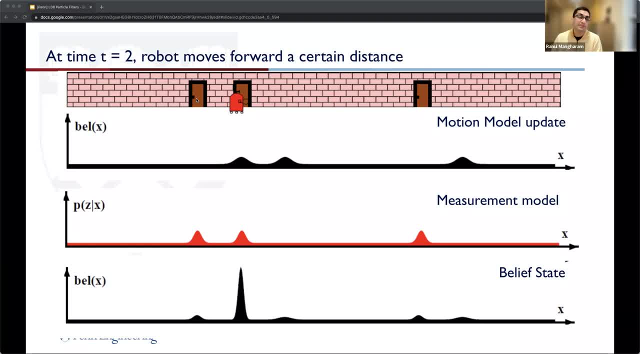 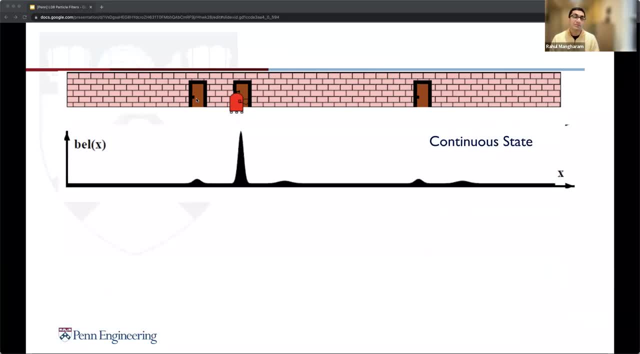 Have no more errors. Bye, bye, Bye. and using this convolution helped us localize ourselves. The location where the probability is high is the place where we actually are. This function is really interesting. It's a distribution that focuses most of its weight onto the correct hypothesis of the robot. 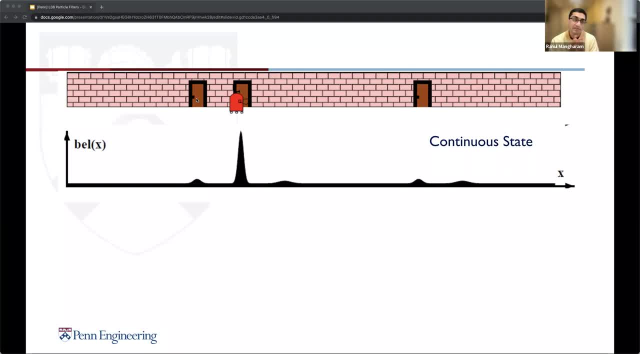 being near the second door. However, practically this belief state is not used as a continuous function, as that makes it computationally very expensive. It is instead sampled to produce discrete points or positions. Each of these sample positions is called a particle, Hence we can represent our entire belief state. 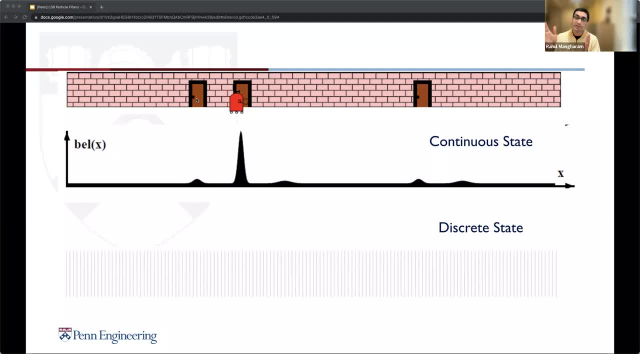 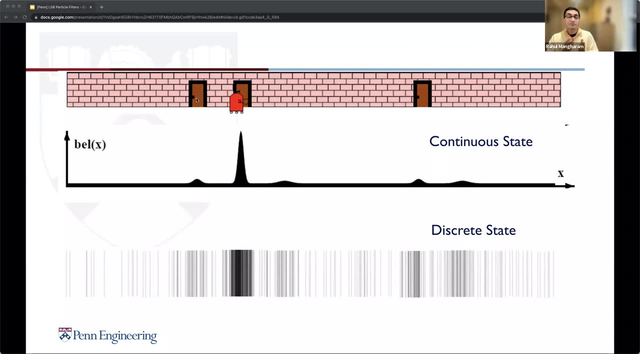 as a discrete set of particle positions of the corridor, each associated with the probability of the robot located at that position. Also, instead of using uniform sampling, where samples or particles are drawn from equal distance apart, we draw particles wherever the probability of the belief state is high. 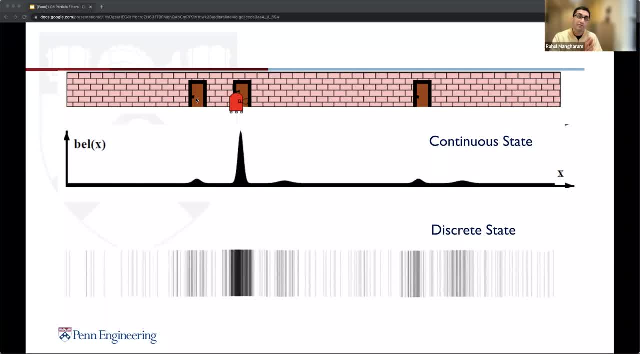 So here, since we have more probability of being near the middle door, the particles are more densely drawn from here compared to other positions where the probability is low. Each of the drawn particles are associated with a weight which is equal to the probability of the belief state. 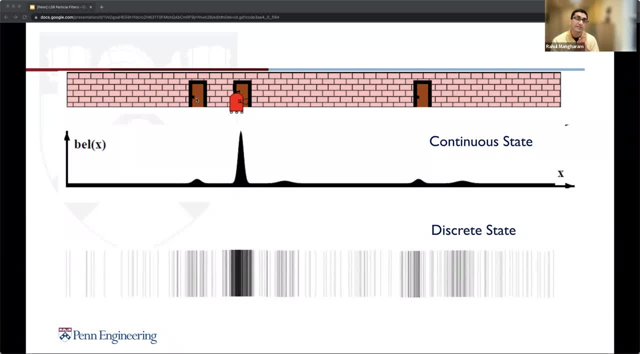 at that location of where the particle is drawn. That is, the particle near the middle door has a high weight, where particles near the other doors have a medium weight and the particles at other- all other positions- have a low weight. We will look at sampling and how these particles are drawn. 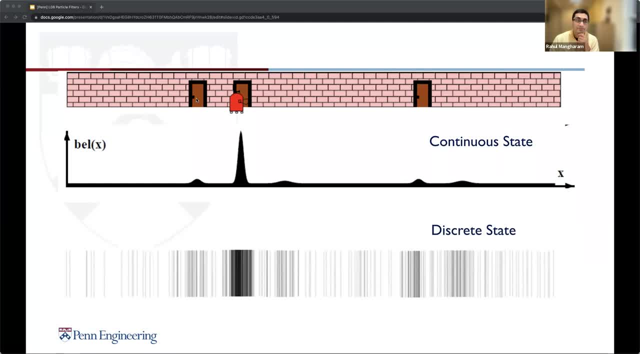 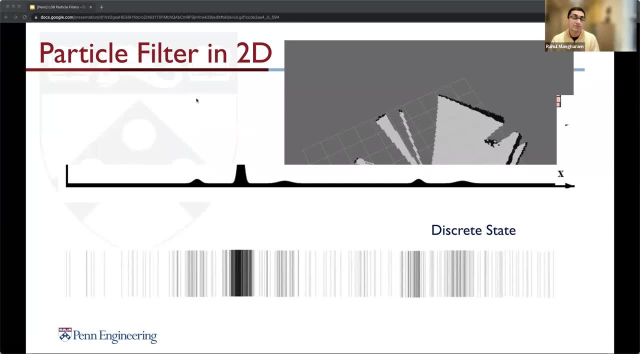 and how they propagate in more detail as we go further. Now let's look at particles in the two dimensions and the process of using them with our race car. Here we will see a map previously generated using Hector mapping. The black pixels of the map denote the walls. 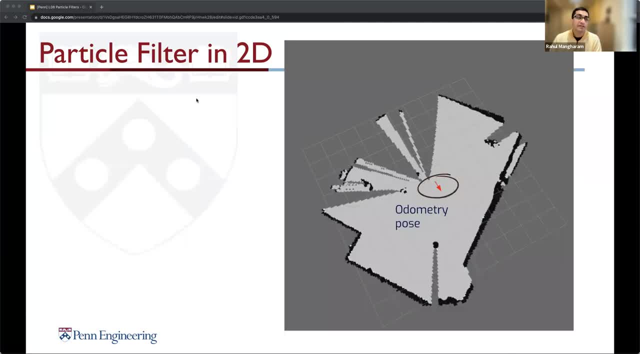 and the gray pixels denote all the free space, The red arrow indicates the distance and the yellow indicates our pose, obtained from odometry, which is not accurate. Let's use particle filters to minimize the error and localize more accurately on the map. First, we generate a set of hypothesis of our positions. 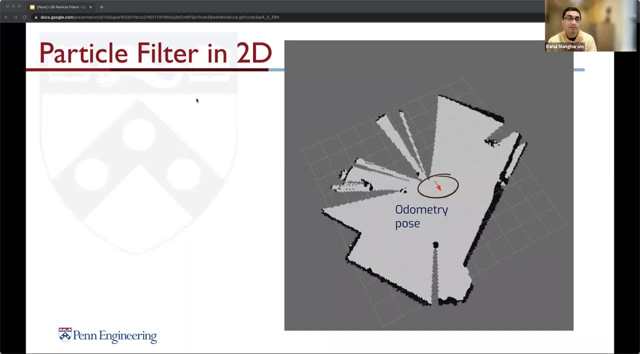 These are the discrete particles drawn from a Gaussian distribution of being, our odometry pose, with some covariance that defines the size of the region around which we draw the particles from. We end up with a set of poses that are obtained by adding noise to our odometry pose. 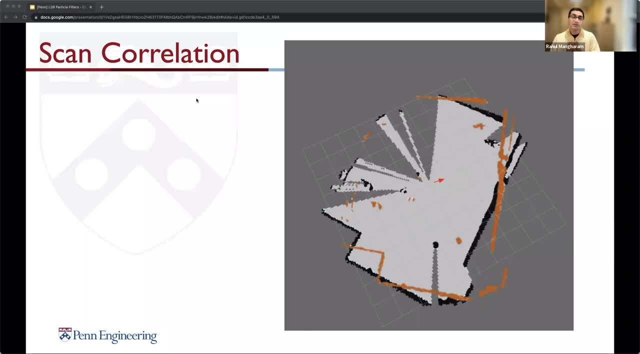 Then, for each particle, we orient the laser scan shown in orange with respect to the particle pose and compute the correlation score. The correlation score S is calculated by using this formula, where A is our map and B is our scan. A bar and B bar are the mean values for all the pixel values. 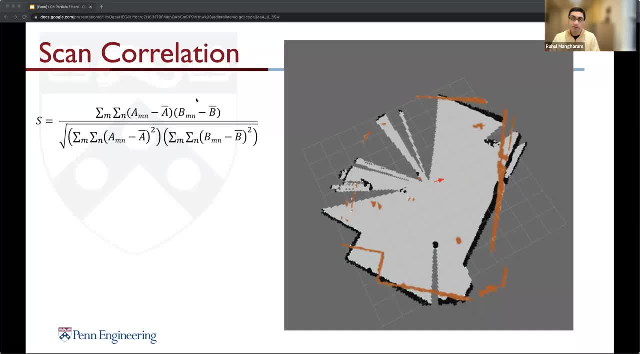 of the respective maps. The F and D bar are the mean values for all the pixels in the map, where walls have a value of one and free space, as we know, has a value of zero. M and N are the X and Y coordinates of the pixels. 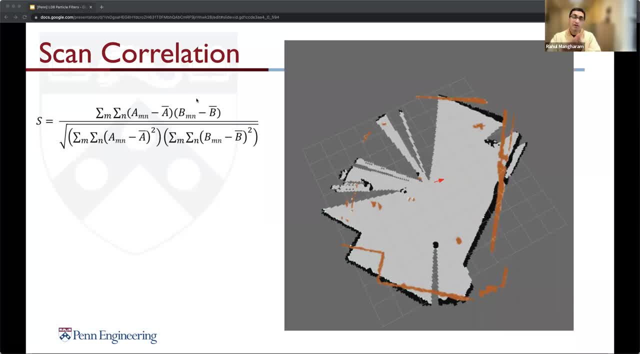 This equation basically counts the number of black and orange pixels- That's, our wall pixels- that are overlapping. We repeat this for each particle and then record the correlation score for each. The particle that aligns well with the map has a high correlation score. 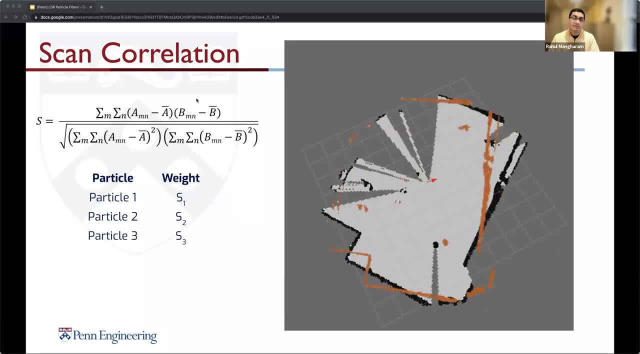 So we can walk through particle one, the two, and we see that each particle is a guess, with a different orientation and a different position, and finally we see that particle six- that's pretty good over there, right, and this particle with the maximum weight is chosen as the pose of the robot at the current state. 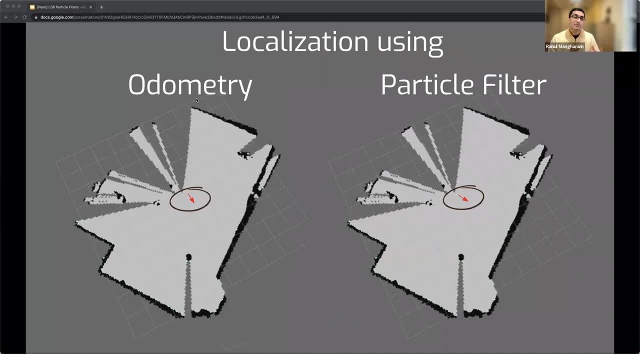 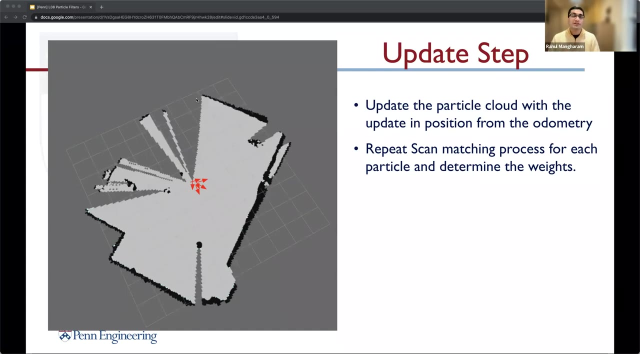 notice that drift in the pose of the odometry seen in the image to the left is corrected by the particle filter in the image on the right. this might seem minor now but as we keep driving the drift will get larger. we repeat this procedure of correlation for each sensor update. 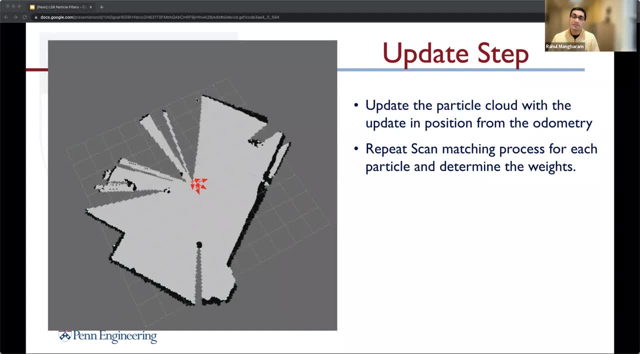 first we propagate each of the particles we generated based on the distance and direction defined by odometry. then we perform the correlation of each particle as described previously and then record the correlation scores. the weights of the particles are kept track of the correlation scores and then we repeat this procedure of correlation for each sensor. 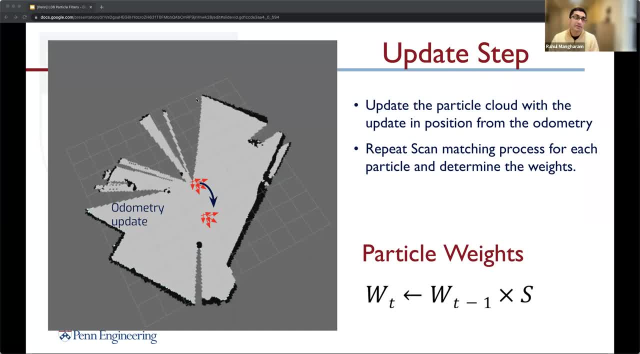 track off by normalizing and multiplying over time steps. the scores at time step t is first normalized by dividing the largest score at time step t and then multiplied the previous weight of the particles at time set t minus one. in this way we can keep track of how well each particle 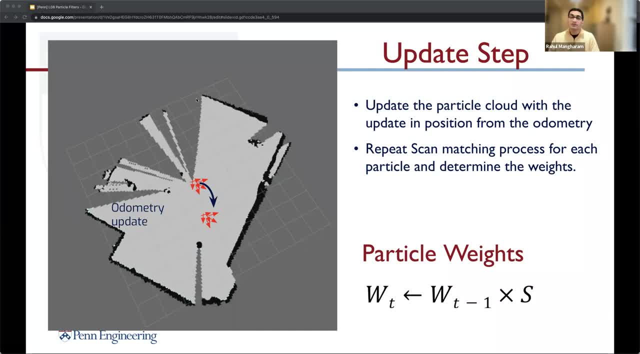 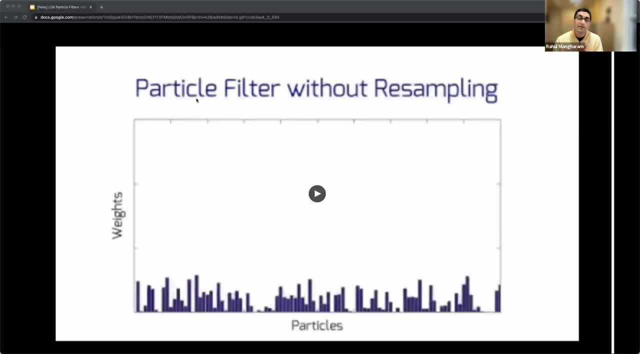 performs and draw more particles from the neighborhood in from that neighborhood. you know when it's needed. as we are multiplying the weights over iterations, the particles with small weights reduce to a very small weight and then we can keep track of how well each particle performs, and then we can keep track of how well each particle performs. and then we can keep track of how well each particle performs. 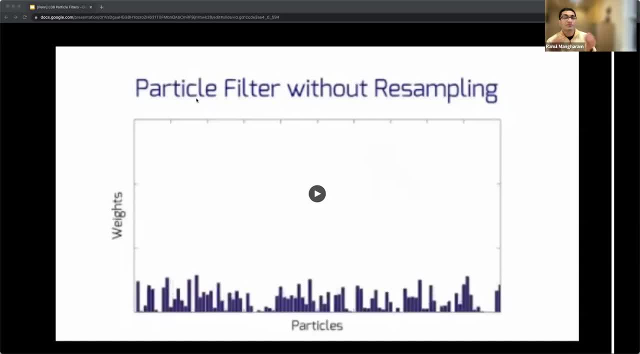 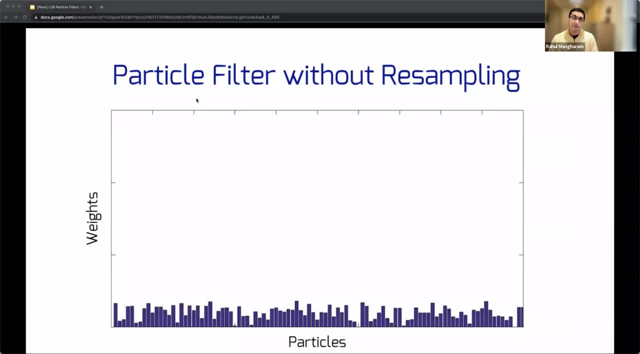 value over time and the particle filter has effectively very few particles to produce good results. this graph shows the particle number along the x-axis and the weights along the y-axis. we can see over iterations, only very few particles become prominent. to avoid this, we resample the 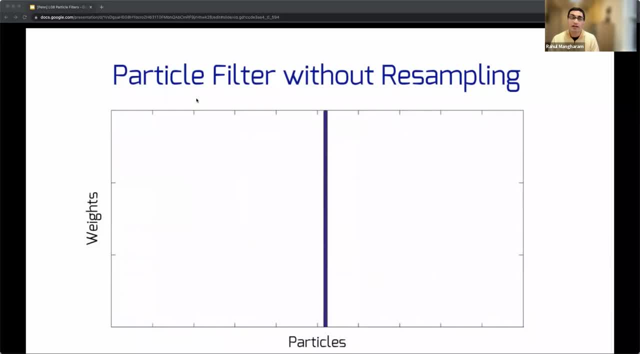 particles, when the effective particles become too few and reset all of the weights. so we don't want to get into this local minima, because that could be you know a set of values that we can use to get into this local minima, because that could be you know a set of values that we can use to 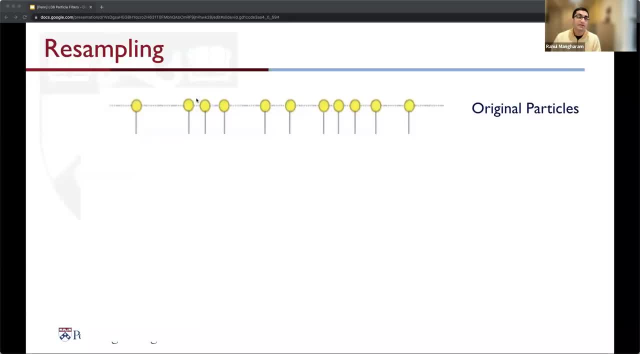 wrong guesses that has led us there and get stuck. then consider these yellow circles as the initial set of particles that we drew from the distribution. as they propagate over time, their weights change and few particles become very prominent over the others. the size of the blue particles denote their 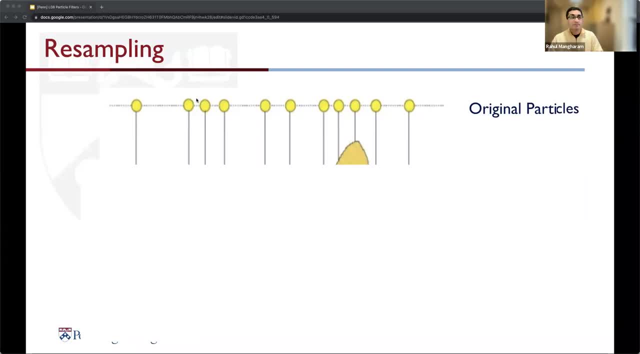 weight. the larger the size, the larger is the weight. when the size of the blue particles becomes very large, the particles have to be resampled. the resampling is done by drawing more particles close to the particles having the higher weight than those that have a smaller weight. thus, a new set of yellow particles drawn have a higher 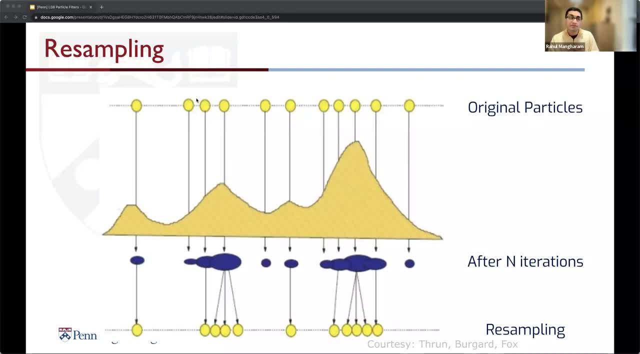 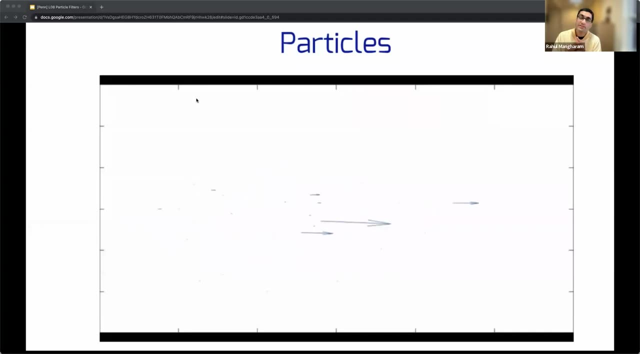 density near the position where the particles with the larger weight existed. all the new particles drawn have the same weight and the particle filter begins from scratch. the graph is a plot of x and y position of each particle. each arrow represents a particle that has the same weight and is, of course. 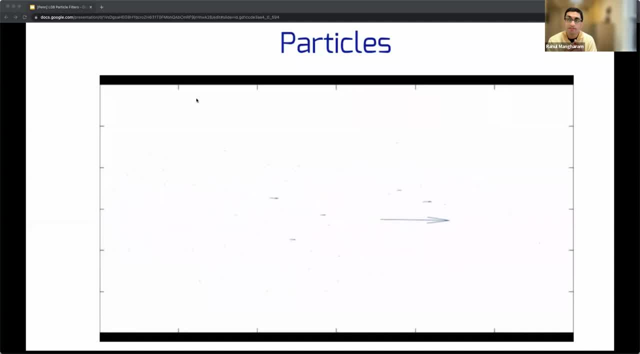 different, at which point the star is closer to the state of the particle and thus higher, and therefore and its orientation as an arrowhead. The size of the arrowhead is proportional to its weight. The larger the weight becomes, the larger the arrow. So over iterations, as we can see here, 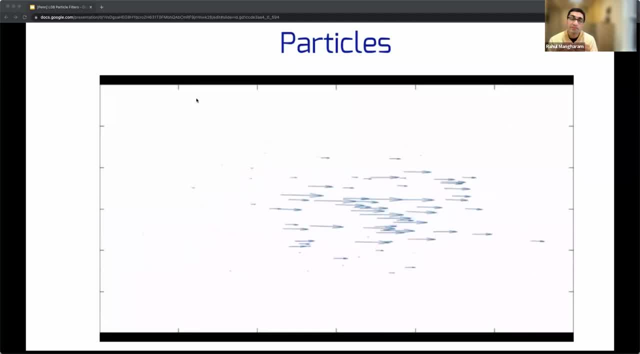 few particles become large compared to the others. When this happens, the particles are resampled. We can see that the particles that have more weight are resampled into many small particles very close to it, And very few particles are present. far away from that. 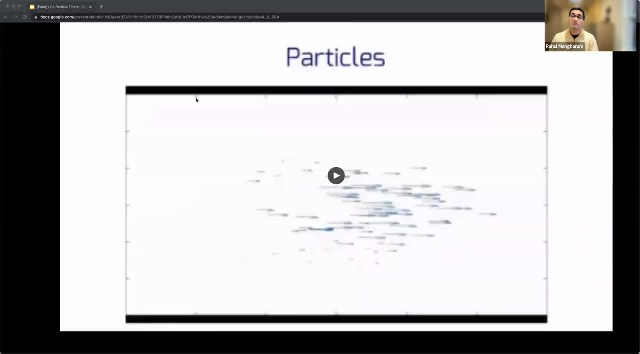 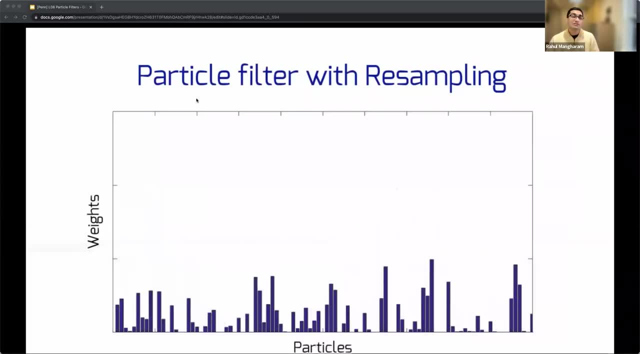 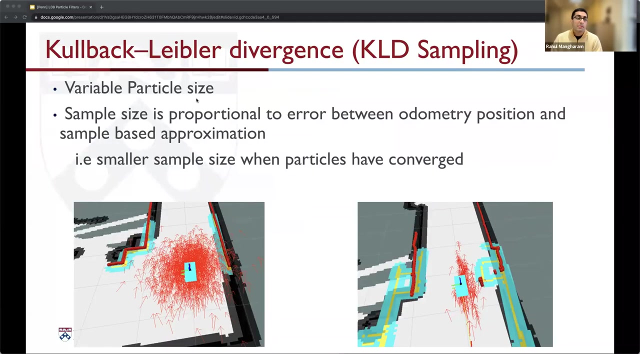 With this procedure it is made sure that no particle dominates the distribution and all have a fair chance. Hence now our particle versus weight graph resamples whenever the particles become very few and starts off with equal weights again. This form of localization is computationally expensive. 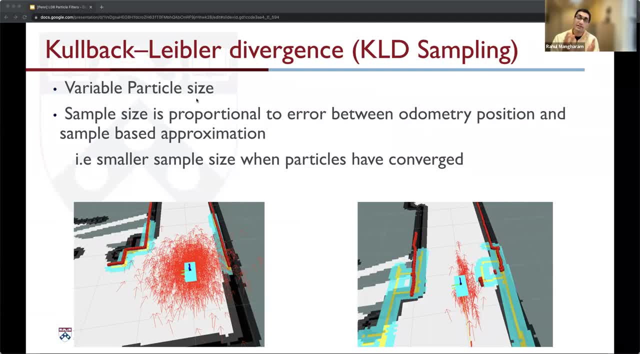 because the need to iteratively calculate the correlation of each particle is costly. So larger the number of particles, more time is taken to localize. In order to optimize this, we use a sampling method called KLD sampling. This technique controls the number of particles. 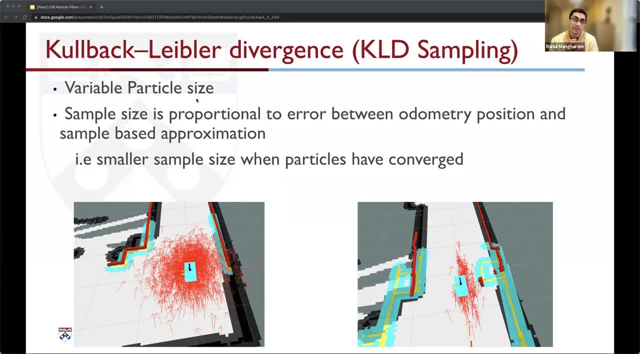 based on the difference in odometry and particle-based localization. Initially, when the position is unknown, the particle cloud is low, And when the position is unknown, the particle cloud is low, And when the position is unknown, the particle cloud is large, as we can see in the first figure. 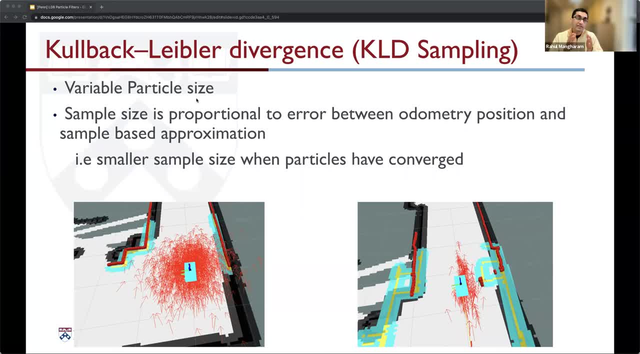 on the left due to the uncertainty in the position, But as the car moves, the particles converge and the particle cloud then reduces. Thus KLD sampling, culls redundant particles and improves performance. Now that we saw how the particle filter can, 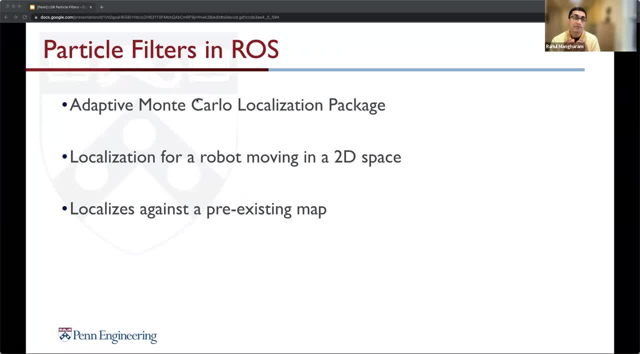 be used for localization. let's see how it is implemented in ROS. This is called adaptive Monte Carlo localization, commonly known as the AMCL package. The word adaptive refers to the KLD sampling. This package can be used for localizing with laser scans. 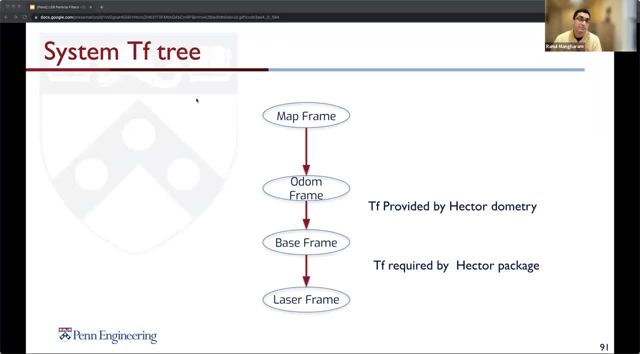 against a pre-existing laser map in two dimensions. The Hector odometry provides a transform between the odometry frame and the base frame. The AMCL package provides an other transform to correct for the drift in the Hector odometry to localize accurately in the map. 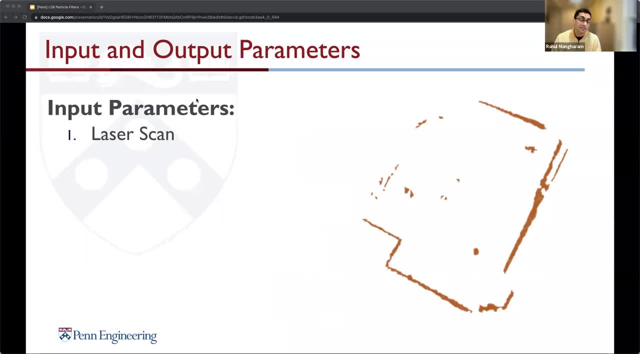 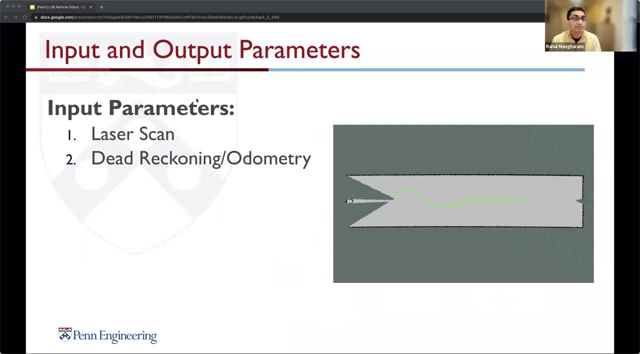 The input parameter is the Hector odometer. The parameters are the sensor- That's basically our laser scan- An odometry source- In this case that's our Hector odometry- And a pre-built map. that are all the three inputs of this package. 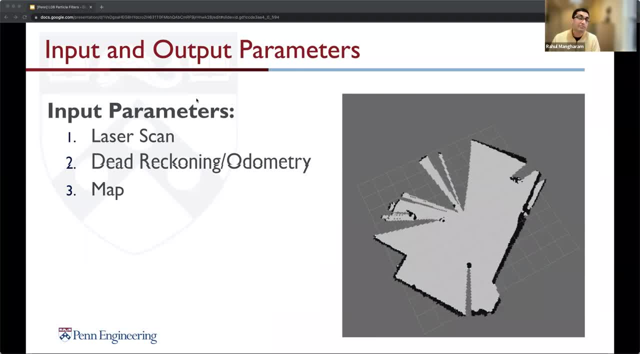 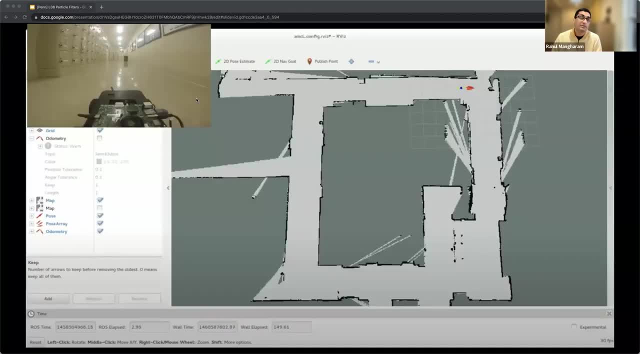 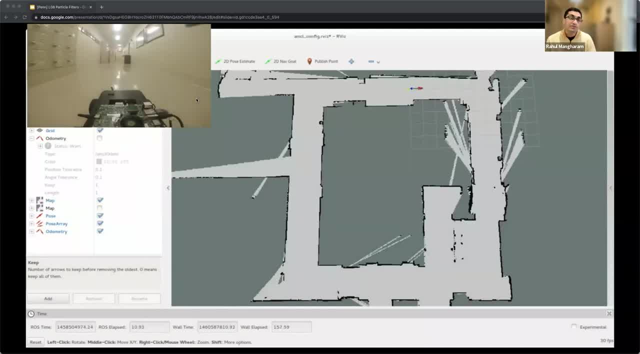 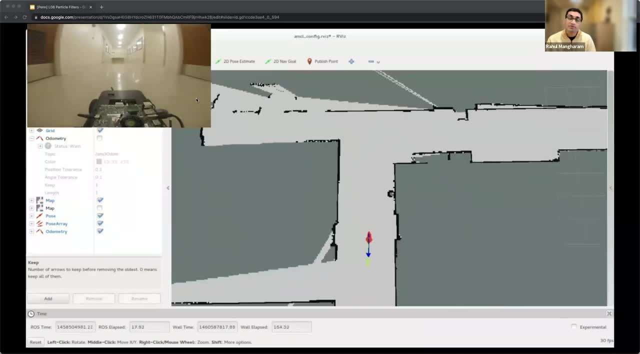 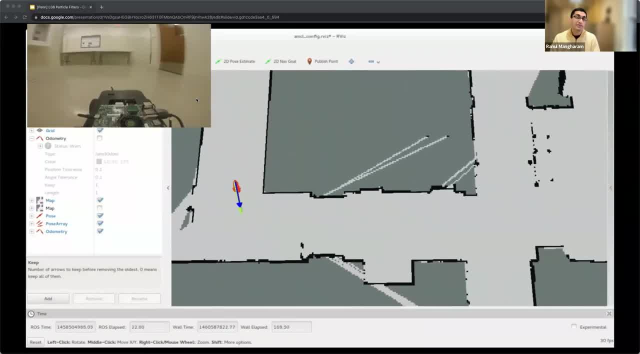 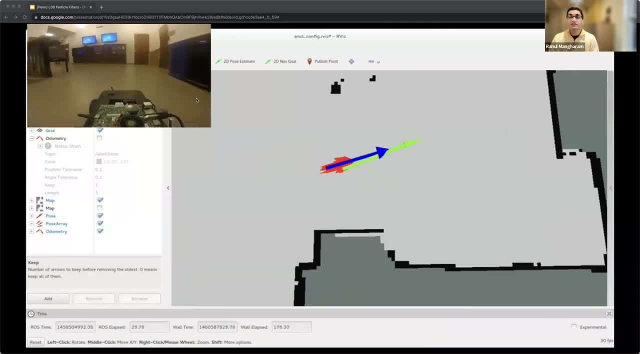 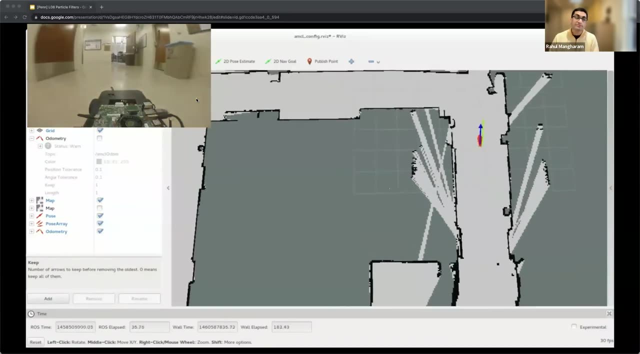 The particles are represented by many small red arrows. The difference between the position of the green and the blue arrows depicts the pose correction performed by AMCL. After traveling a certain distance, the error in the odometry becomes visibly evident from the gap between the green and the blue arrows. 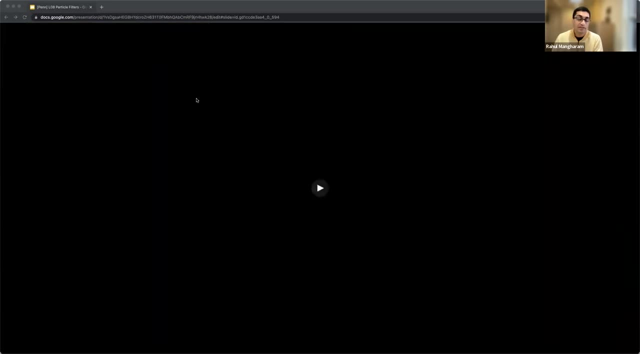 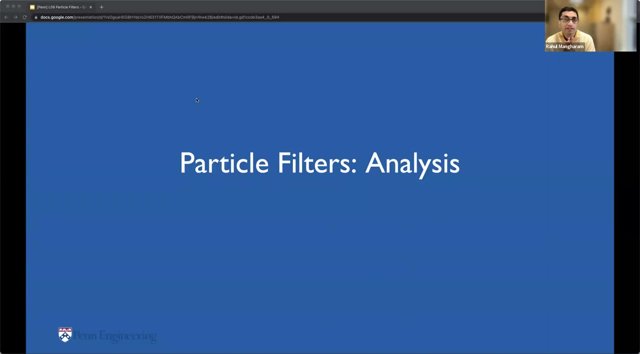 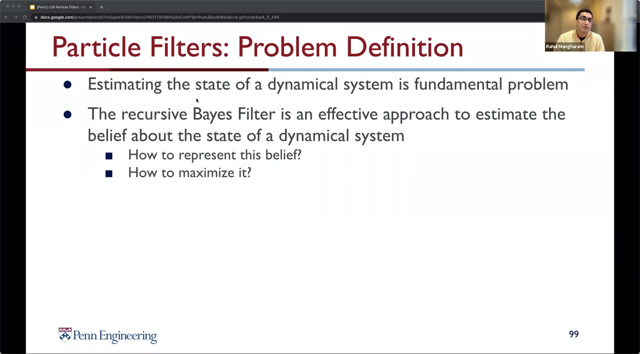 And this is the car basically racing around the corridor, and that's what you will do in your next labs. Now that we have got the intuition behind particle filters, let's analyze the math and the algorithms further. Our problem is to estimate the state. 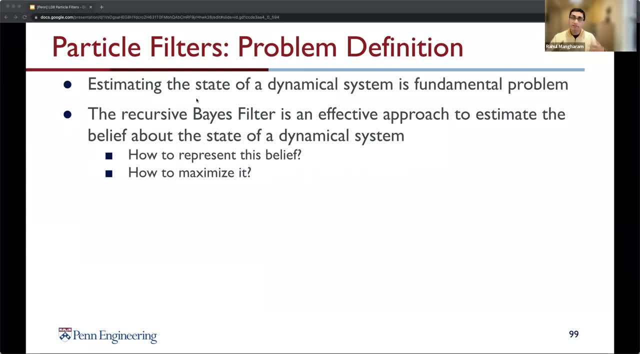 of the dynamical system, and that's the state of the vehicle itself within its environment. In principle, the math and the algorithms behind the particle filter are very similar. It's essentially the same as a recursive Bayes filter. However, there's a particular trick. 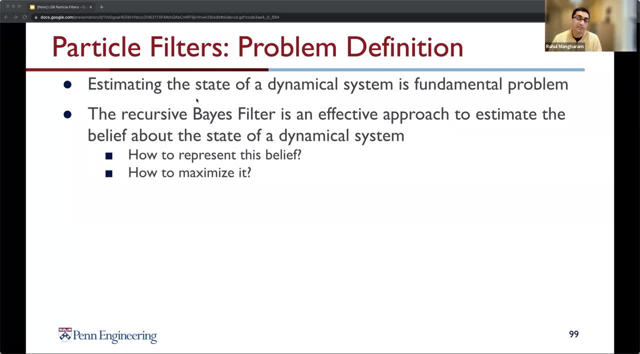 that we use here. that makes the estimation in higher dimensional space more feasible. We're going to address the question of how to actually represent the belief of our state in a probabilistic way. Typically, we also want to know how to maximize it, although we won't address that in the lecture today. 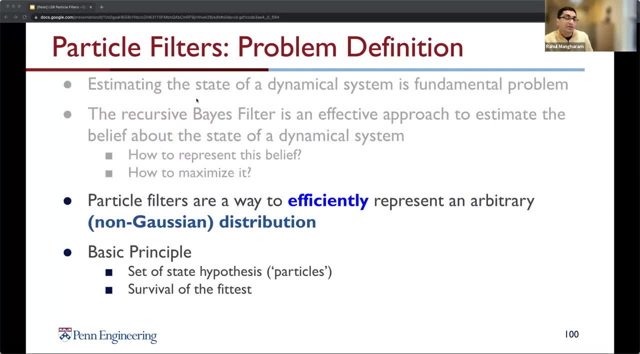 We will look into how particle filters are an efficient way of representing such a problem. So let's start with a probabilistic belief, In particular in situations where this belief doesn't look like a bell-shaped curve and it's not a Gaussian distribution. 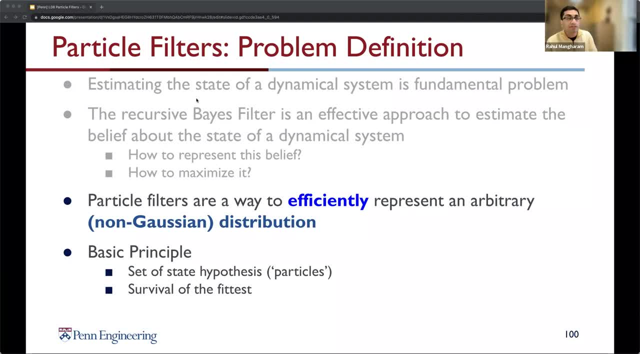 so we cannot use a closed form analytical solutions like we use in the Kalman filter. The key principle is to use sampling to estimate such arbitrary distributions, to capture discrete approximations of the belief by a so-called set of hypotheses or guesses, or particles. What we use is called a survival of a Fittest scheme. 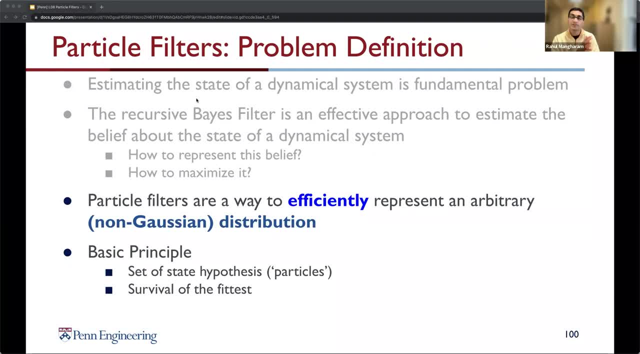 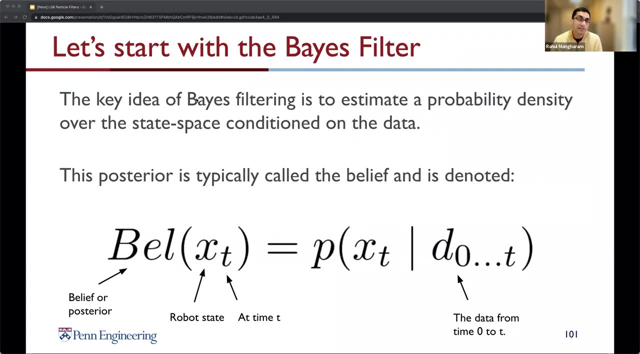 to concentrate our finite particles to better sample an arbitrary distribution of the belief. This is similar to genetic algorithms or evolutionary strategies, where we iteratively use particles to resample based on a cost function. Now Monte Carlo localization uses a recursive Bayes filter that estimates the posterior distribution of robot poses. 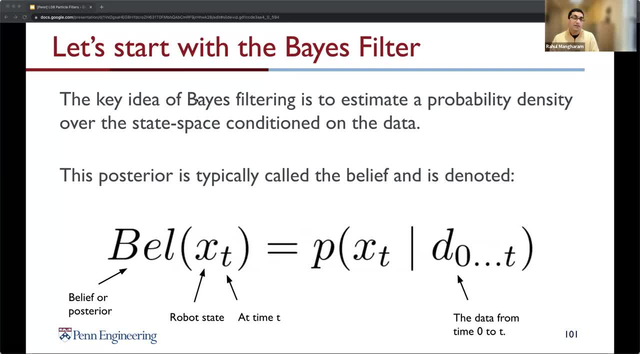 conditioned on sensitivity. The Bayes filter is designed to measure the behavior of a robot in a state X, which is a state of motion, and a state of motion Bayes filters address the problem of estimating a state X of a dynamical system from data or from sensor measurements. 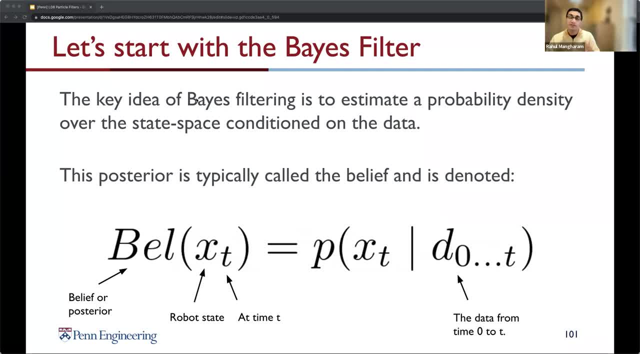 For example, in mobile robot localization, the dynamical system is a mobile robot in its environment, The state is the robot pose. The data term includes sensor measurements. Bayes filter assumes that the environment is Markov, which means that the past and future data are conditionally. 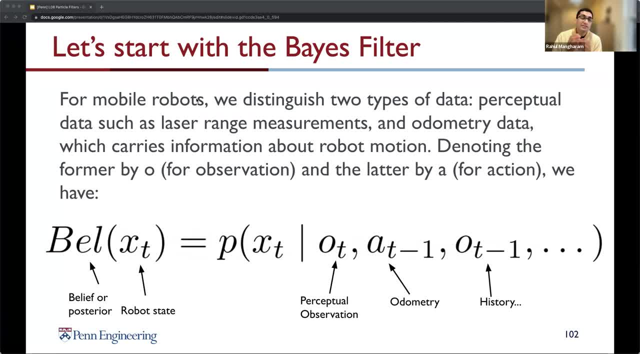 different from the current state. So we are interested in the belief about the state of our dynamical system. right, This is the posterior distribution of the state, given all the actions of the system has carried out and all the observations it has made. So OT are the observations and AT are the actions. 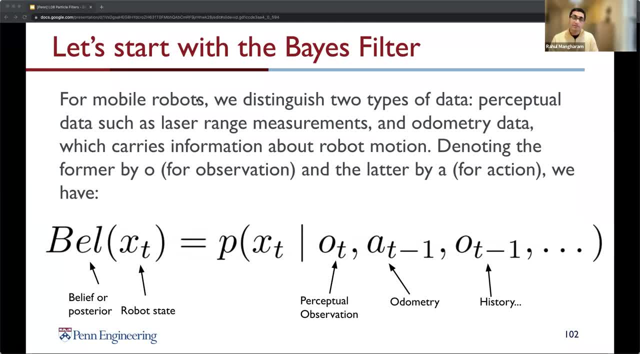 The observations could be camera images, distance recorded by LIDARs or ultrasound sensors, basically inputs from whatever sensors you have. The motions of the mobile robot are the motions captured by the odometer, which convert real movements into angles per second, And from that we can actually calculate. 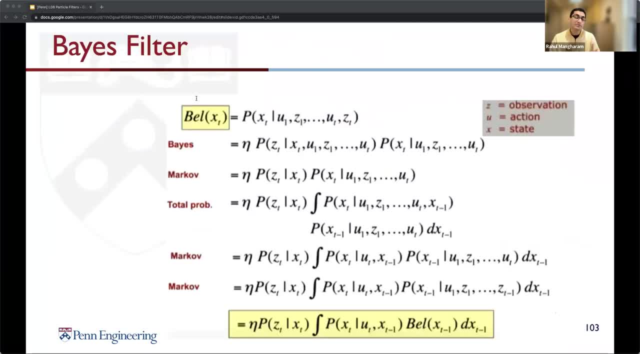 what action the robot might have carried out Now using a couple of mathematical derivations. we won't go into the details here, but I just want to get you to the point of how we can. what is the exact equation that we are working with? 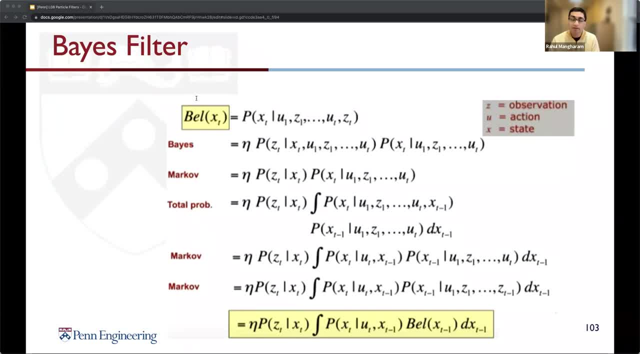 So now, using applying Bayes theory, independent assumptions, law of total probability and another two Markov assumptions, we basically end up with this equation at the bottom in yellow, And this is the nice aspect of this equation is that it's actually a recursive. 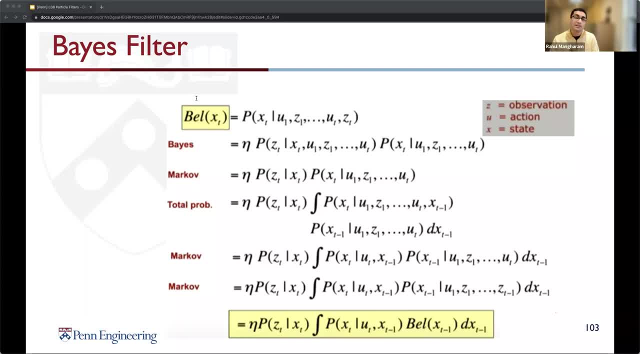 So the belief of the robot state at time t depends on the belief at time t minus 1.. At the bottom there are two components right. The first one is the integral and the second one is a multiplication. on the left-hand side, 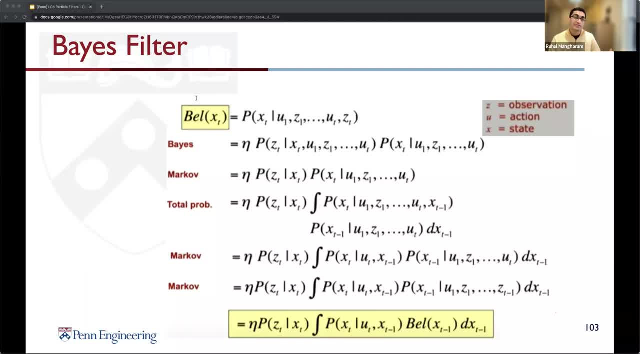 We call this the boshier on the left hand side, the transitional model, where the probability is that you end up in a state xt, given you execute some action u at time t and were at a state xt minus one before. So let's. 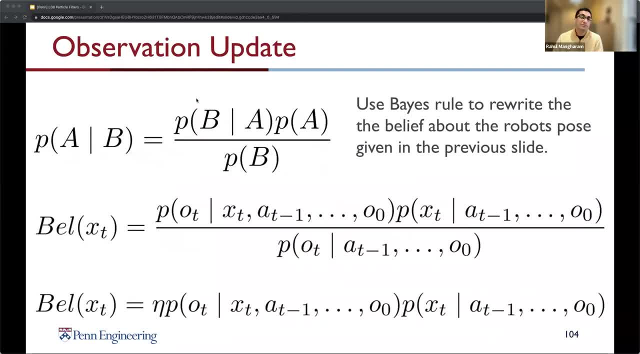 dive into this further. One simplification step involves Bayes' rule, because we are interested in probabilistic way of representing these actions. So if you carry out an action and I want to actually describe the distribution about where I might end up being, as given I was given in xt. 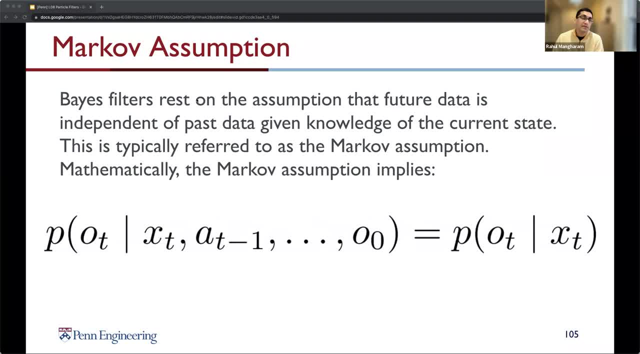 before I executed that action. So the Bayes filter rests on the assumption that the future data is independent of the past data. given the knowledge of the current state, This is typically referred to as a Markov assumption, So we don't have to consider the entire motion history. 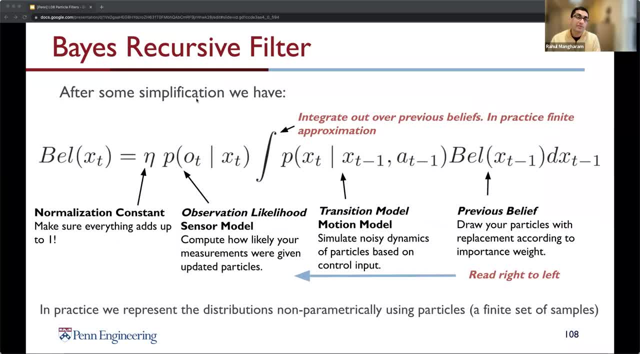 just the current state. So what we have here is the approach to the distribution of the distribution, of the distribution of the current state, To estimate the belief of our current state using the previous belief, the transition model or the motion model, and the observation likelihood or the sensor update model. In this form, 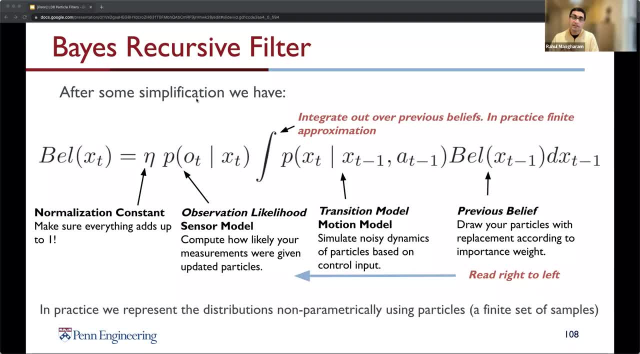 the belief is a continuous function and does not lend itself directly to a computational solution. So how do we use this in practice for our robot localization? What kind of data structure should we use to represent this belief? So one efficient way is to use a finite set of samples of guesses. 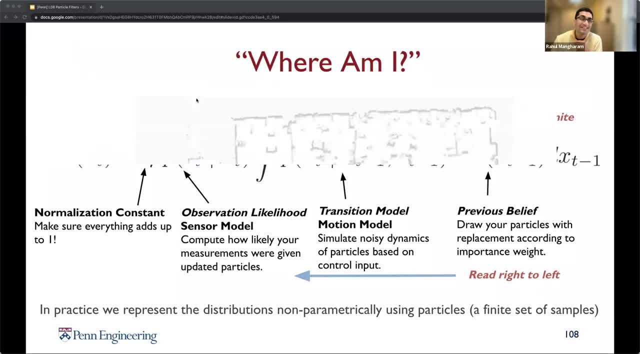 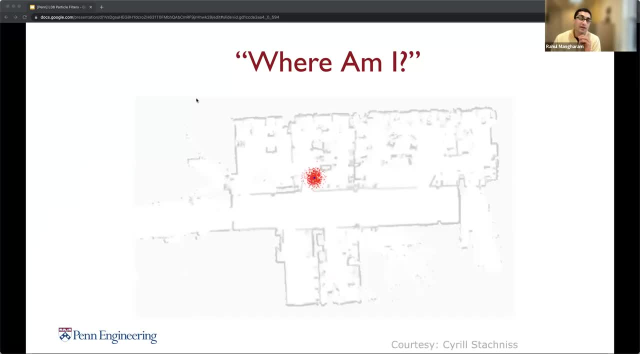 and we call them particles, as you now know. So, given this map, our goal here is to figure out a good estimate of where we are, and I make a bunch of guesses as to what my pose is, and I want to zone in on what my exact pose is. Traditionally, for state estimation, we use Gaussian filters, The Kalman. 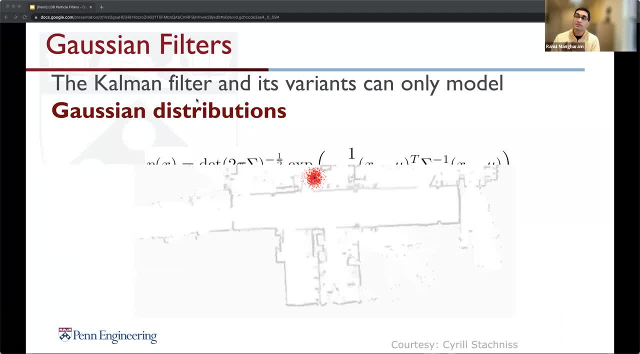 filter is a popular example used to estimate the probability distribution. The underlying assumption is that this probability distribution is to be Gaussian. So if your underlying distribution is Gaussian and if your models are not dramatically non-linear, then the Kalman filter or the EKF is a fine choice. 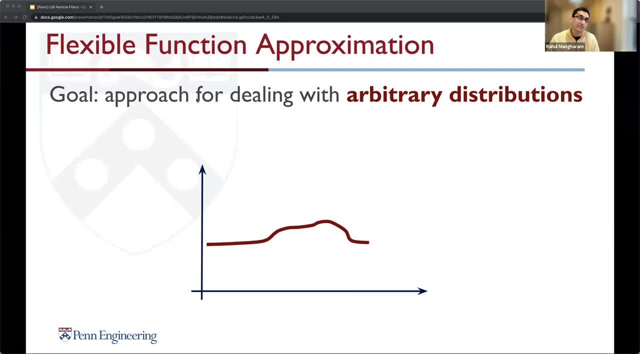 What happens, however, if we have this kind of arbitrary distribution? How can we use a different way of estimating the pose of the robot if we leave the Gaussian world? That's one of the advantages of particle filters as well, that they are very attractive techniques to do. 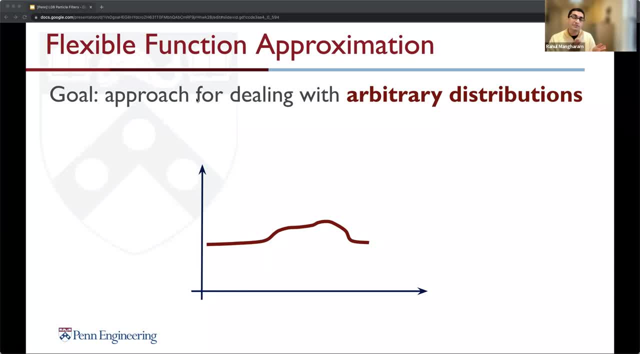 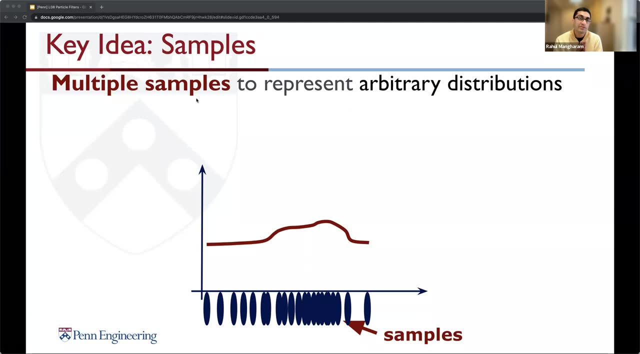 exactly that. So the key idea of the particle filter is not to use a parametric form like a Gaussian, but to use a non-parametric representation of my distribution. here The particle filter uses random samples. So let's say, this is my distribution and I generate a lot of set. 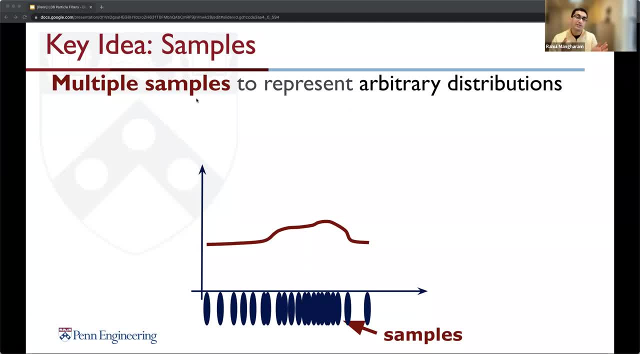 of samples in the beginning I can see the samples as points which live in my x-coordinate, and the more samples I have in a certain area, the higher the probability of that area or the that region. I may also assign a weight to the sample. So bigger the oval here, the higher the 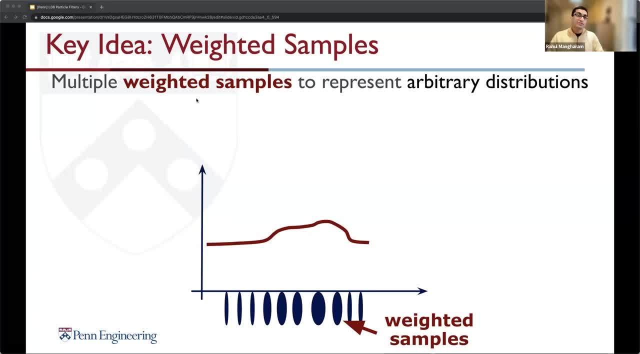 weight and the higher the probability of the corresponding area. So under the peak we have large ovals and the ones at the edges are, you know, where the probability is small. you have small ovals or flatter ones. It's kind of an intuitive way to see the samples. 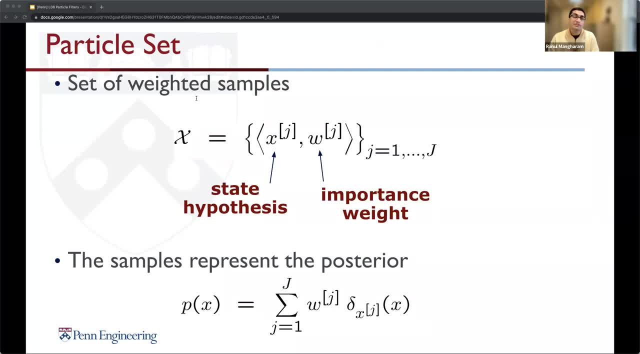 So we represent the posterior by a set of samples and we see every sample as a state hypothesis. So one possible explanation of what the state is, one possible state the system may be in. So I could have thousand samples to represent thousand possible states. the system could be. 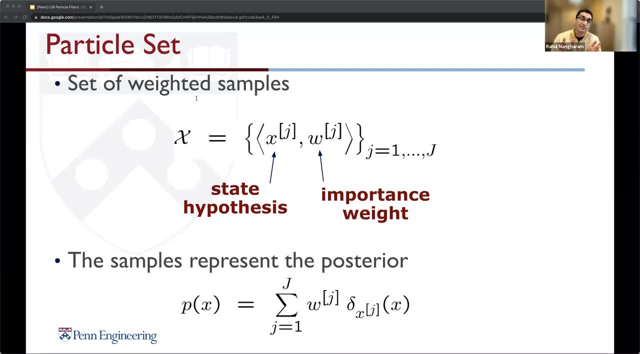 in. That's the key idea. So you have areas of large uncertainty. You may need to have a large number, a huge number of samples, So there's no free lunch. You are more flexible with what we have here, because we can represent, you know, any arbitrary function, But this comes at a 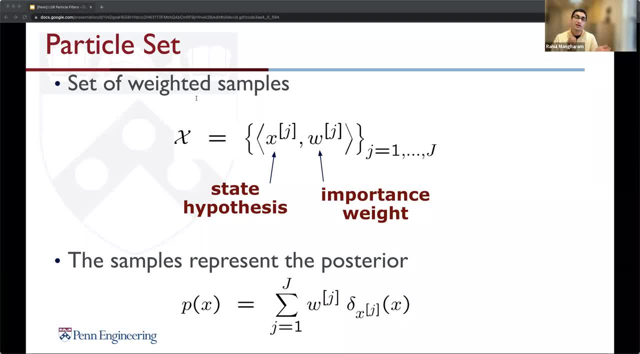 high computational cost. On the other hand, for a Kalman filter it basically needs about the same computational resources for varying degrees of uncertainty. So for the state hypothesis X and I I typically have an importance weight. So the probability distribution we obtained from 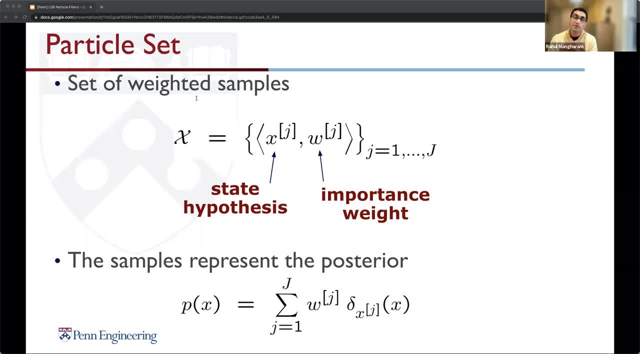 this sample set represents is just a sum over all samples and the weight of the individual samples and the Dirac distribution centered in the state of the sample. Again, the Dirac distribution is zero outside the state and infinite at the state, but the integral is one. 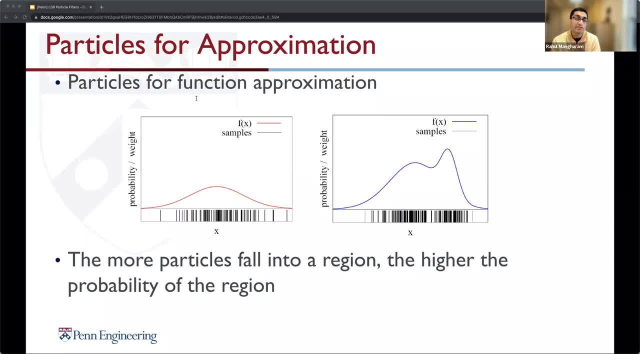 So I can use these particles or samples for function approximation. On the left is a Gaussian distribution and below it is a sample based representation. The more samples I have, the better approximation will be and, as you can see the area you know at the mode of the curve. 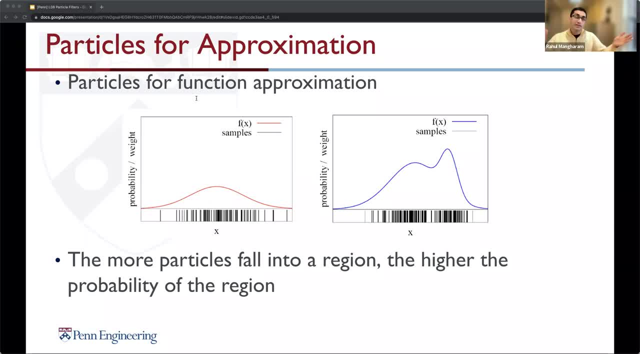 has more samples concentrated and then there are less samples towards the tail of the Gaussian. On the right you have this fancy distribution where the peaks have high concentrations of samples and the smaller concentration at the dips. So more samples, I have better approximation. The question is, how do we obtain these? 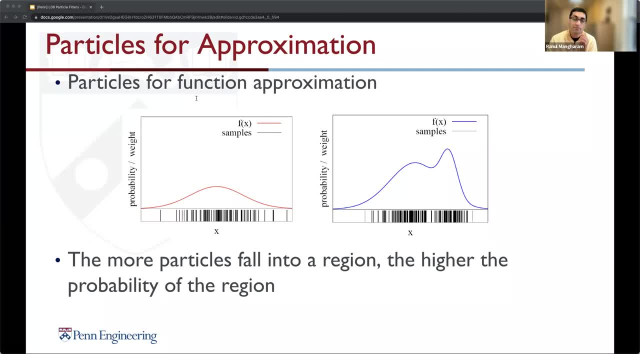 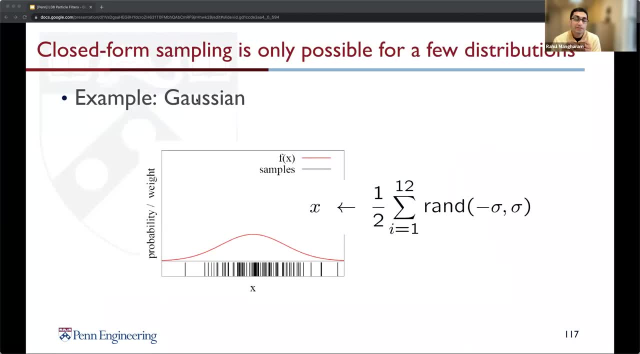 samples and how can we actually generate those samples. and that can be, you know, a little tricky. So if my state estimation is a Gaussian distribution, I can use this closed form. you know, term is to just take 12 random numbers between minus and plus the standard deviation. 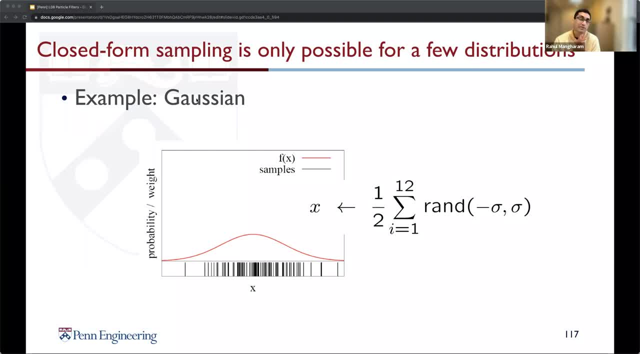 of the Gaussian distribution. sum all of them up and divide by two. This generates samples from a Gaussian distribution that's centered around zero with a standard deviation. So for certain distributions like a Gaussian, I can efficiently generate these samples right. but the question is, what about other distributions that cannot be represented by this kind of? 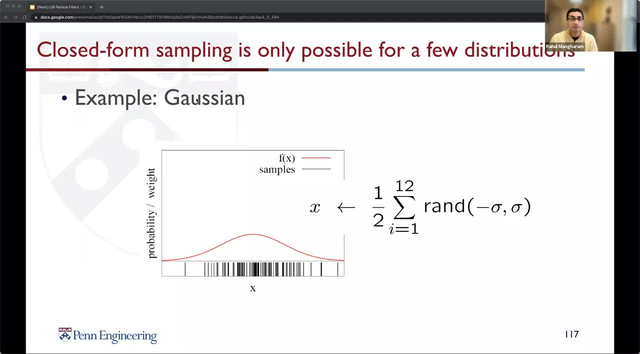 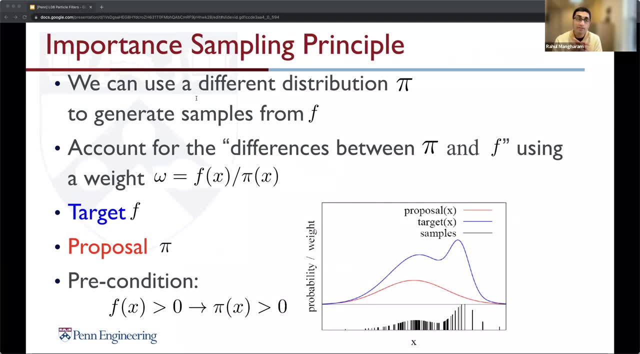 closed form equation. How do we generate samples for those distributions? One technique relies on the importance sampling principle. Let's say we have a function f which is also called the target distribution. right, so that's in blue over here. We want to generate samples from this target distribution. Unfortunately, this distribution has some 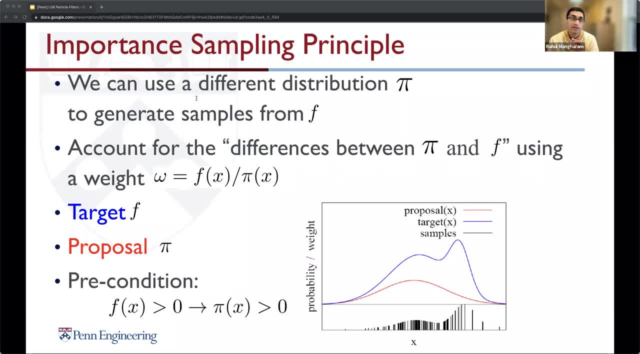 form where we cannot generate samples from in a closed form. The important sampling principle tells us that we can use a different distribution, which is called g or the proposal distribution, or sometimes called pi later on, and we can actually generate samples from this other distribution, from the proposal. Let's say we take a Gaussian as a proposal. 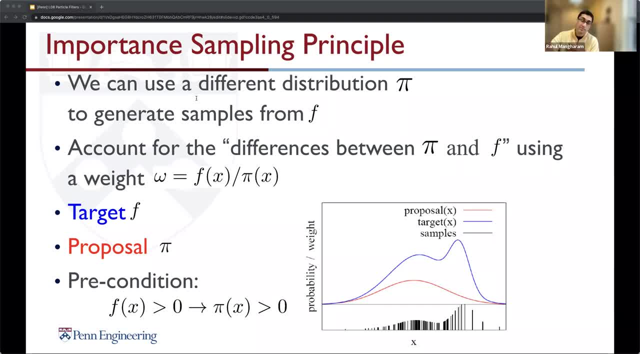 which is different from what the target is. obviously you can see that between you know the Gaussian in red and our target distribution in blue. So we have our proposal in red right and we have selected the Gaussian as our proposal. So we generate samples from this proposal distribution. 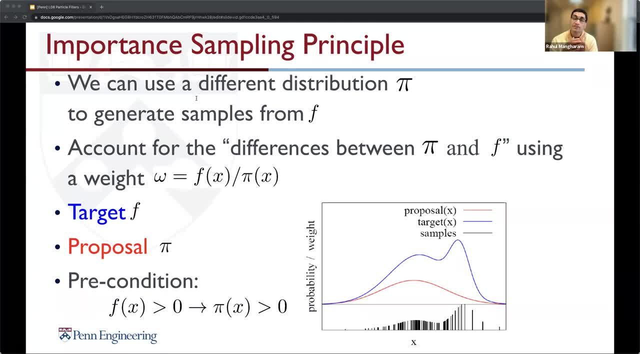 and then we do a correction taking into account the difference between the target distribution and the proposal distribution. This introduces the weights called the local importance weights. So this is given by evaluating the value of the target at the sample location divided by the proposal distribution and that gives me the weight. So if I have my proposal distribution in red and my 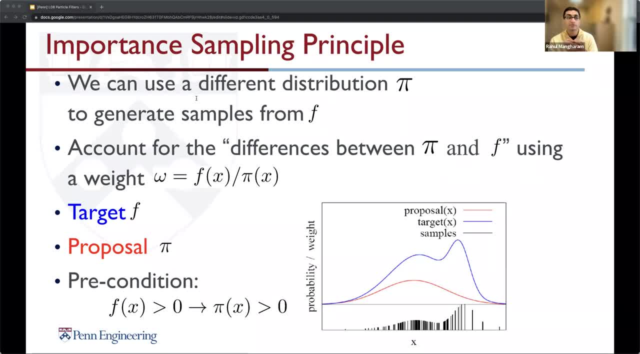 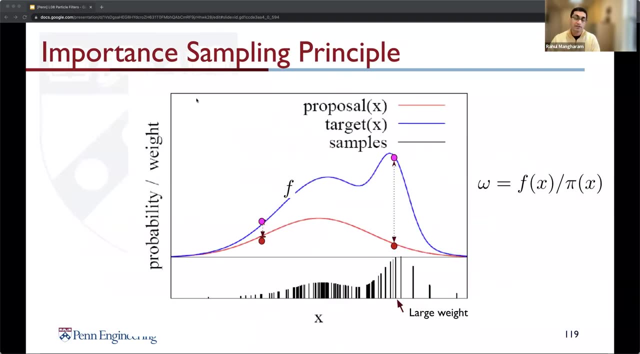 target distribution blue. I generate samples from this Gaussian distribution. So the spacing in x, the location x drawn from the Gaussian distribution, but then the weight of the sample, is the difference between these two distributions. So as we can see here, I think I can have a large weight when the difference is large and a small weight when the 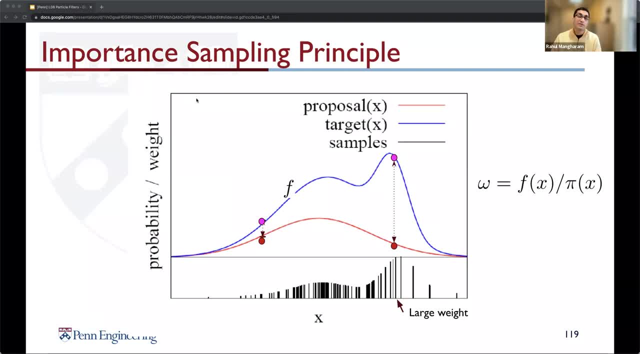 difference is small. So if there's a big difference I get a large weight depending on the ratio, and so a large or small weight in this way corrects the samples, and I obtain samples which follow my target distribution. That's what the importance sampling principle tells us. 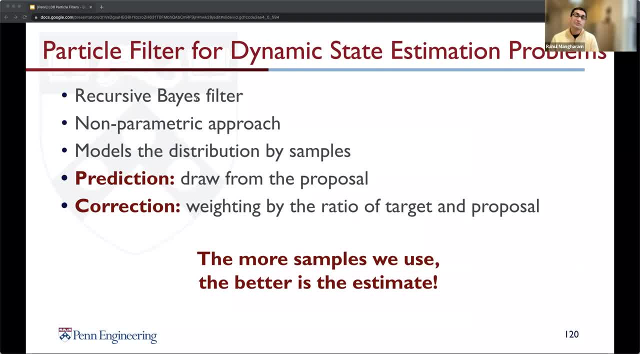 What the particle filter now does is it uses the samples which represent the posterior and uses exactly the importance, this sampling principle, to update the belief. So it's a recursive based filter and specifically a non-parametric recursive based filter. That means we do not maintain a 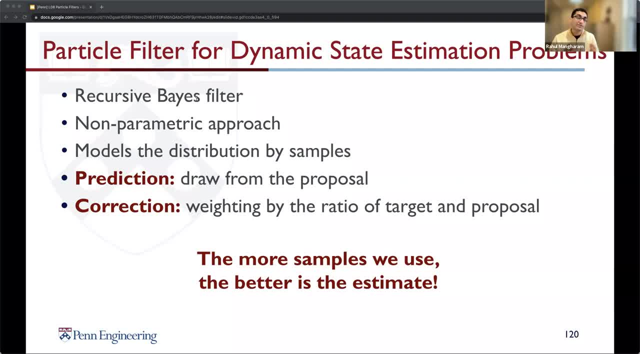 closed form distribution. like a Gaussian for the target distribution. We take those random samples as my representation of the underlying distribution and I update my samples based on the motions that I have and based on the observations that I obtain. It does this in two steps: a prediction step. 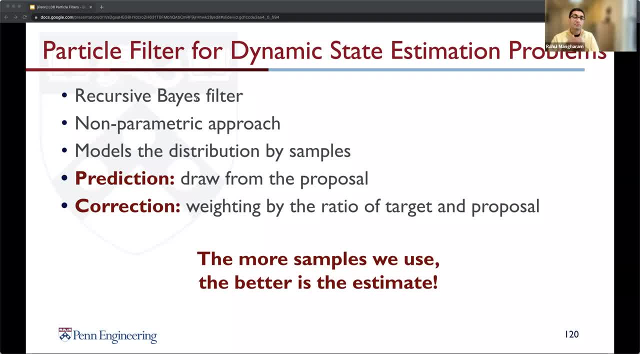 and a correction step. The prediction step draws samples from the proposal distribution. That's a distribution I can easily sample from In terms of localization. I typically use my motion odometry as my proposal to generate new samples, taking into account the motion of the platform. 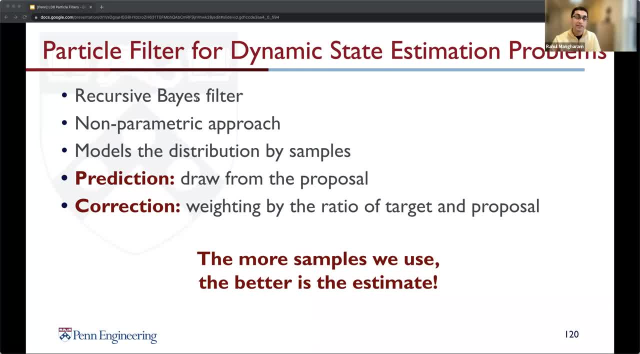 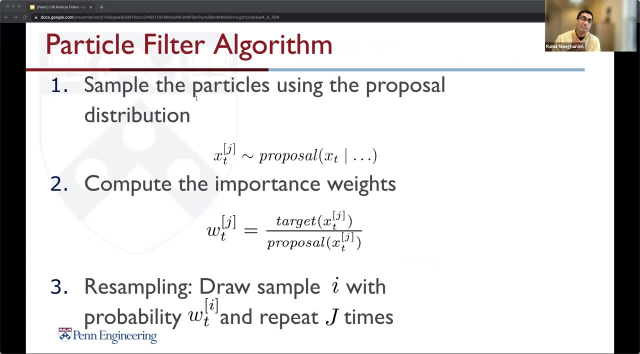 and then I take my observations for doing the correction. That's my LIDAR scan. Therefore, if we do this, we see the connection between the prediction and the correction step. The important thing is more samples, you know. obviously we have better estimate. The particle filter has three main steps now. First it samples the proposal distribution. 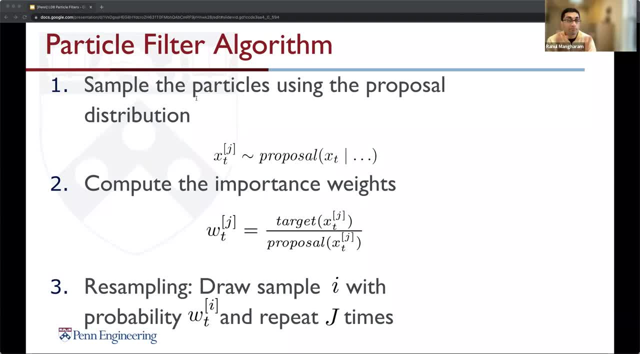 This is where it generates the samples from my proposal. This is a distribution which I choose as a designer and from which I can sample efficiently. and let's say, for the sake of argument: so I choose a Gaussian distribution here because that's efficient to sample from. 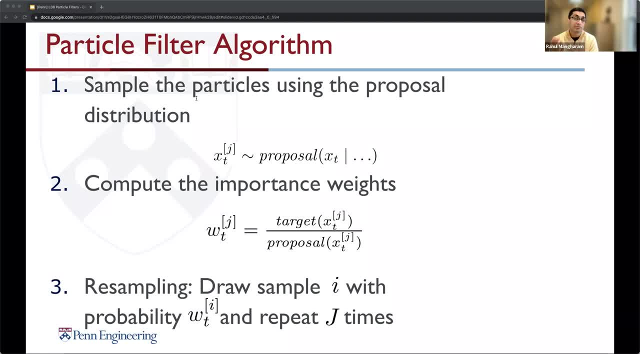 Then we compute the importance, weight, which takes into account the function that I actually want to approximate. the only thing I require here is that I can evaluate point to point wise, so for every point in space, I can evaluate this value and divide it by the proposal. This does the correction, telling me what's the difference between the. 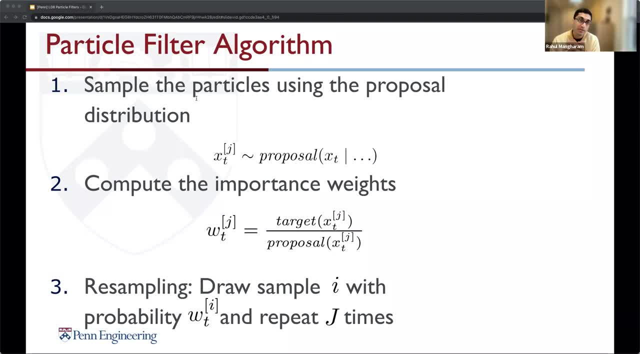 proposal that I chose to generate samples from and the function that I want to approximate of a correction for the fact that I actually sampled the wrong distribution right. The third step is a so-called resampling step and it's kind of sampling with replacement, So I have my weighted. 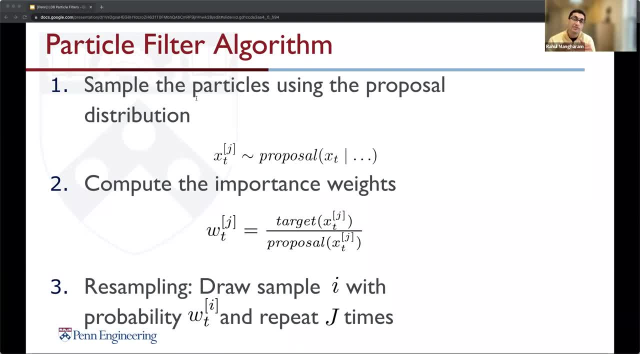 sample, step after step three, and then I just draw J samples out of that with replacement. The probability of drawing a sample is proportional to the importance- weight. You can see this, informally speaking, as a kind of survival of the fittest. It's quite likely to pick a sample with a high 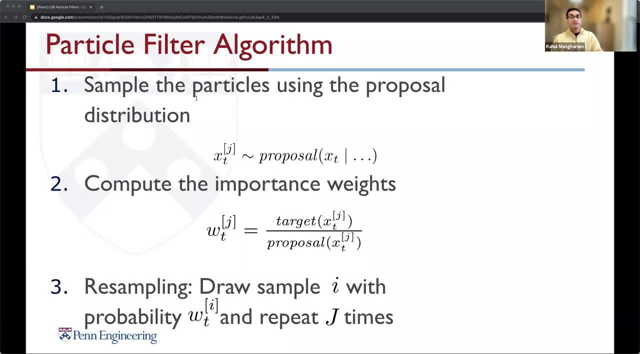 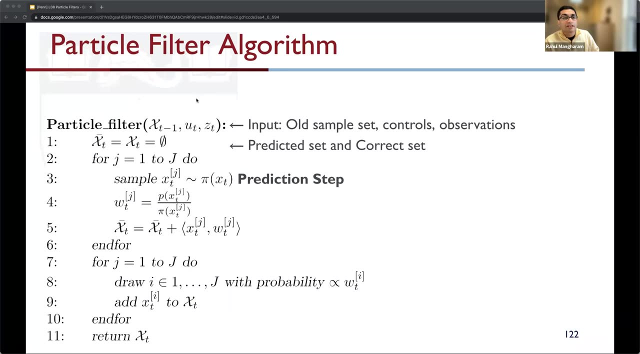 weight where the approximation was good, and I eliminate these samples which haven't been drawn, So those are more likely to have a small weight and they essentially just die out. This way I focus my sample set on the likely part of the state space. So let's look at how this is captured. 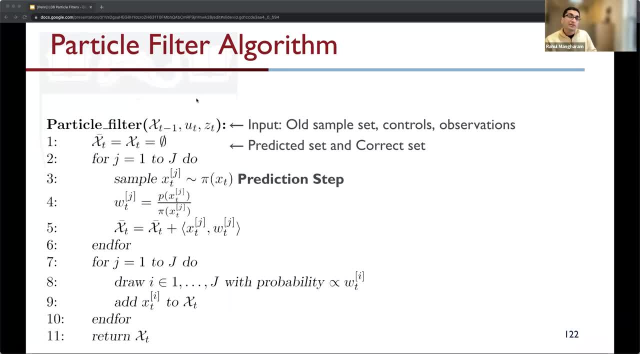 in the particle filter algorithm As inputs. you know, I have my old sample set- that is the previous belief over here- as XT and my controls and my observations right. So the same input as a base filter. Now we initialize two new sets: The predicted set, 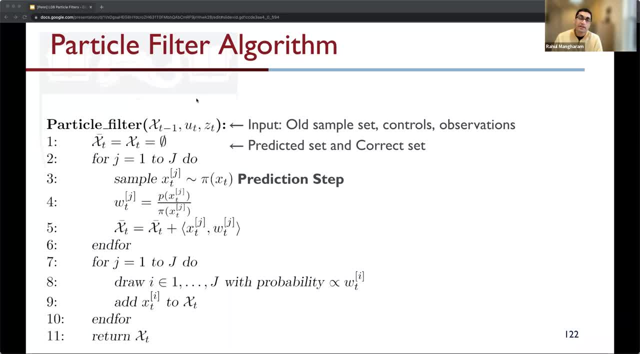 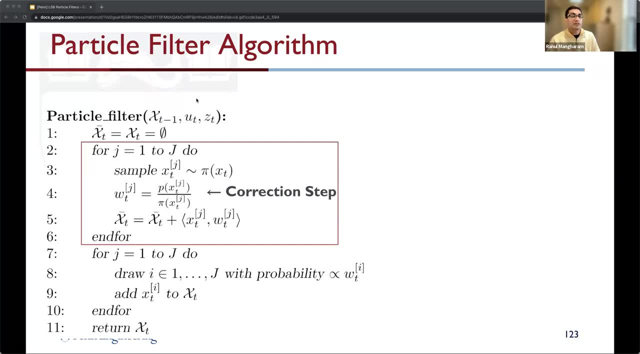 and the correction step, The two new sets over here and we initialize and they both start as empty sets. I iterate over all my samples in my previous belief and I obtain a new sample J by sampling from my proposal distribution In practice for localization. I take the sample. 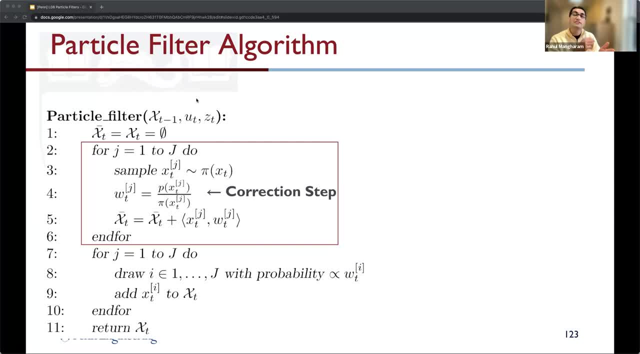 out of my previous belief, apply a motion forward and then sample around that area. For every sample, I compute the correction by taking the target distribution divided by the proposal and I add that to my predictive sample set. This is what I do for all the samples. 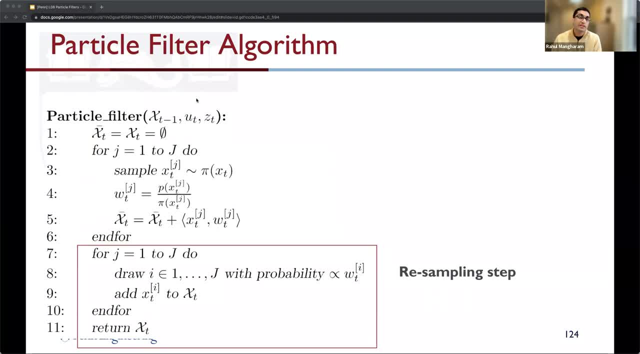 in this loop. Next, what we see down here as a resampling step. So we draw a particle that's the eye that's proportional to its weight, and I include it into my resulting sampling set. This is what we return. Let's look specifically into Monte Carlo localization, which is a specific 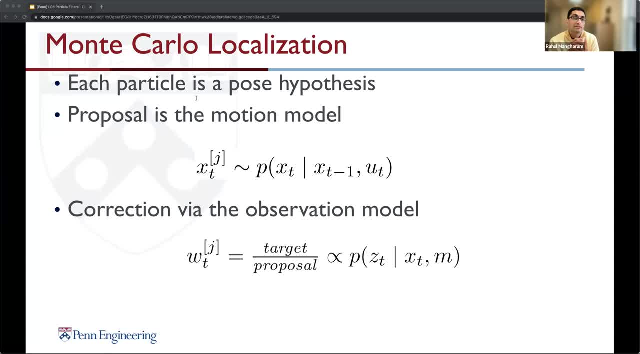 instance of particle filtering. So for each particle there is a pose hypothesis of the robot, So it has an x y theta state of the system that I may be in, Typically in Monte Carlo. localization for the proposal distribution: we choose the motion model. So 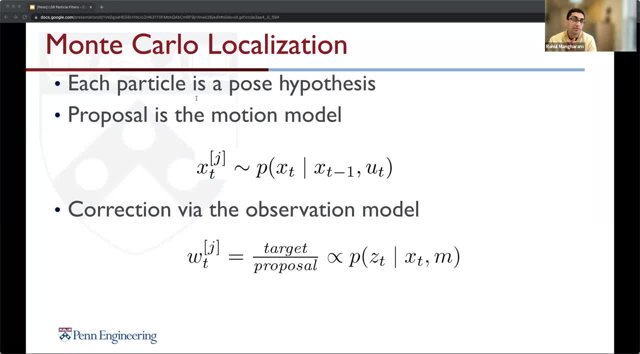 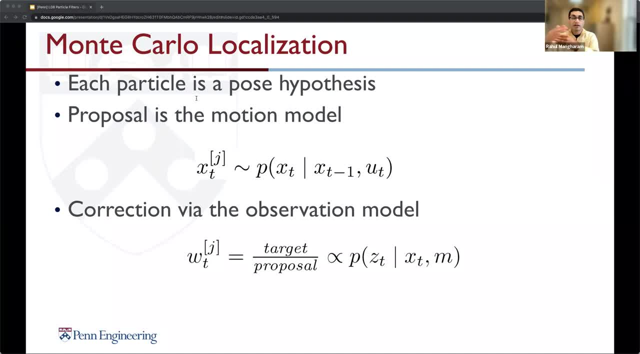 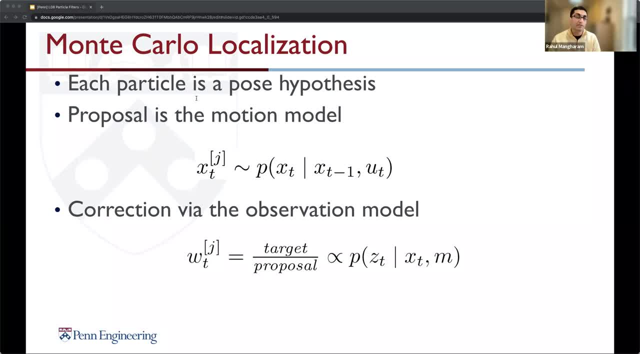 exactly my observation model And I'm getting a better and better fit now. So if you use the motion model as your proposal, that's your final observation model that you're going to obtain, So we can derive the particle filter algorithm for. 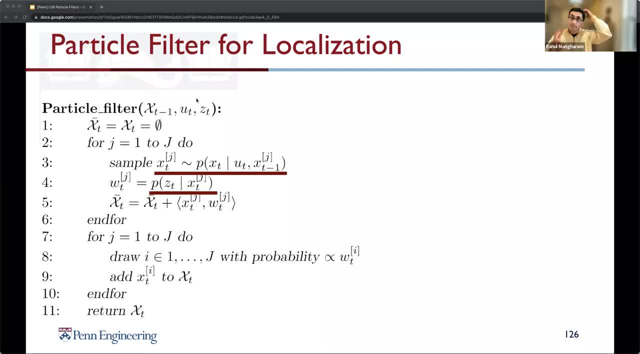 localization in exactly the same algorithm that we had before, Except we changed. you know, the two lines which are underlined in red, in which my odometry model, the motion model, odometry motion model as which I sample, and the observation model for 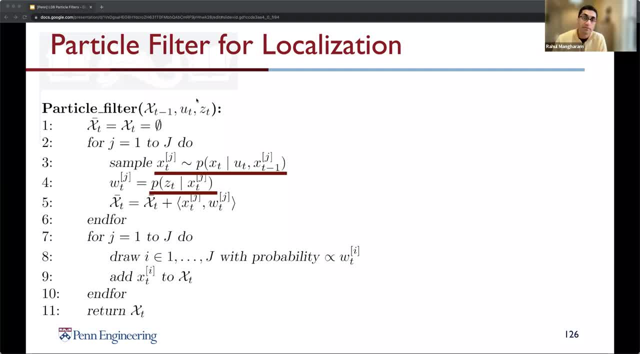 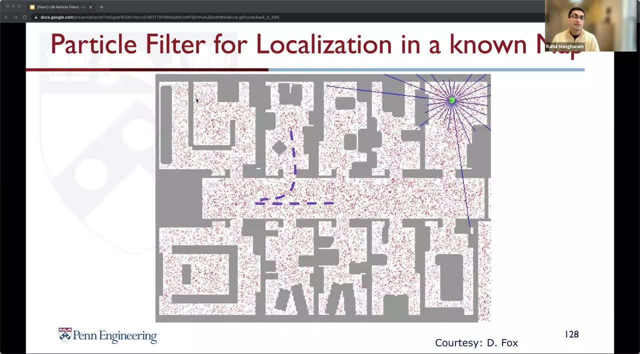 doing the correction Right. So I'm using my motion model and I'm using my observation model for the correction step. So what we see now in this example here are samples, you know, spread all over the place at the initial point in time. 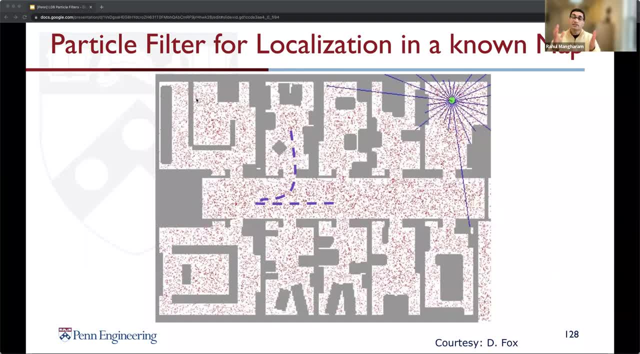 right, So all the red dots are samples, you know, as that's one possible pose where the robot may be at the moment. In reality, the robot was starting at the center, you know, in this purple dashed line that you see here, and moving across the corridor and then going to a room on the top. 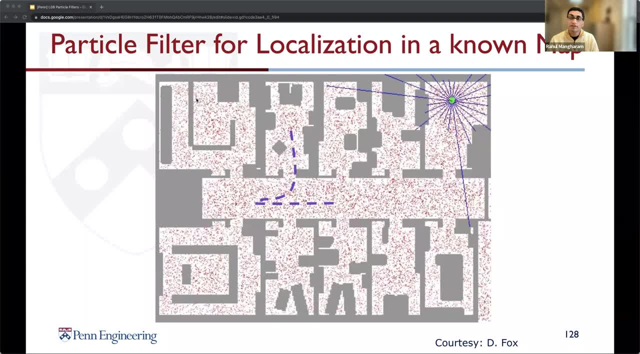 In the top right over here you see the green dot illustrates the initial best estimate. In the beginning the location is random because it's just one random particle. as you know, it might have some weight right. So these blue lines are kind of the sonar readings of the robot. 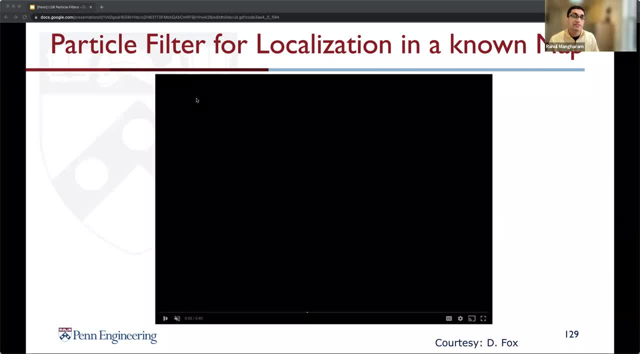 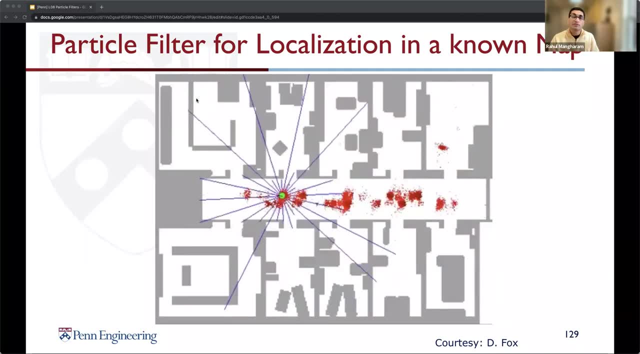 that actually is perceiving this world with the sonar scans, And what we see right now is a sequence of prediction and correction steps and resampling steps that evolve this state. So we propagate all samples forward according to the motion of the robot, we weigh them and then we 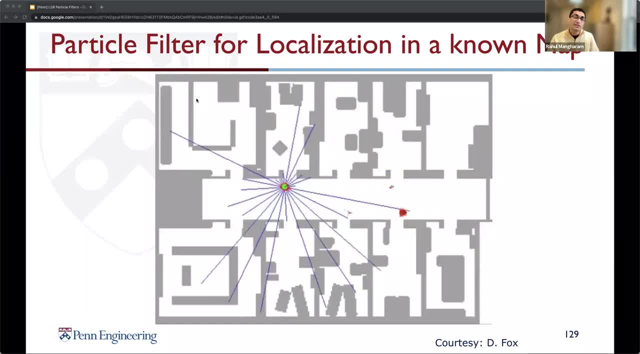 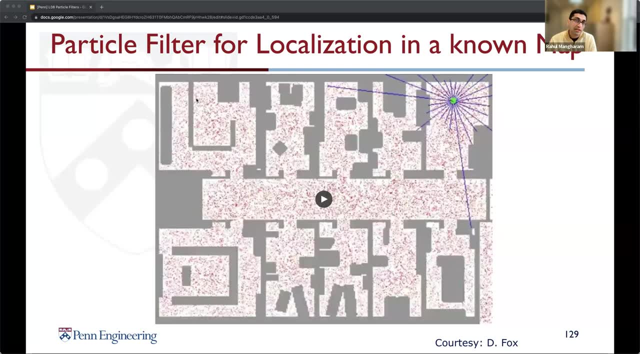 do the resampling step. With each resampling step, the bad prediction particles are more likely to die out and the good particles are more likely to survive. After a few steps, the system identifies a road you know must be the corridor, because that's the area which best aligns with the 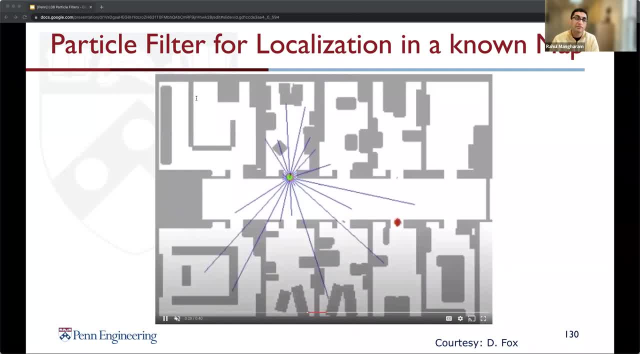 observation. Then we see something very interesting happening over here. We have two states because the corridor is quite symmetric, So there is no way to figure out which one is better until it goes into the room and you can say: okay, the observations for this room and not that room over. 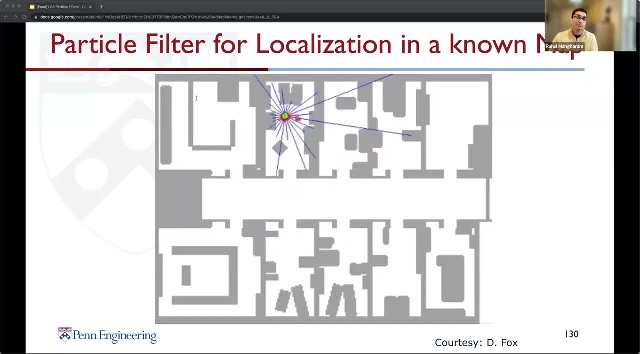 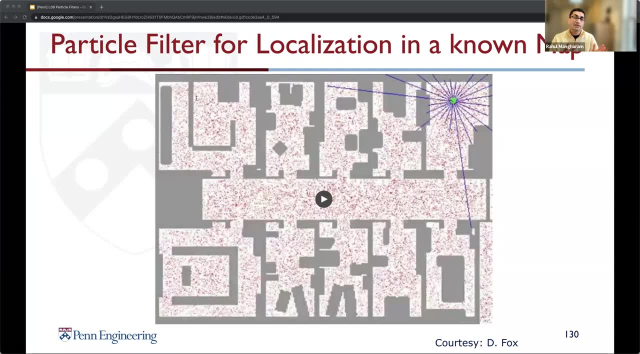 there, And so those samples die out from the room at the bottom and the other samples set from the room at the top survive. That's the kind of nice thing over here, because during the estimation position we can have multimodal distributions Right. I mean we could be in any of these rooms, or 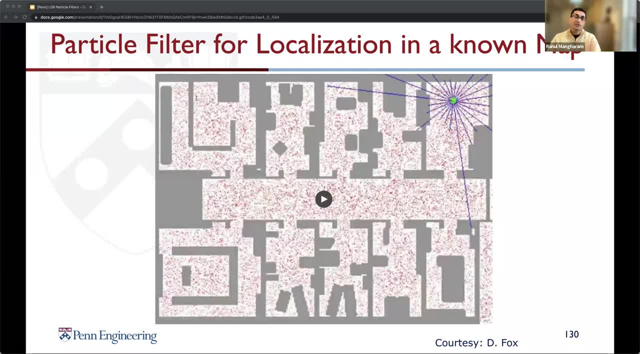 than either of these two rooms, Or we could be here or there. right, We can't be here and there, but we have to. we are trying to zone in on where we are, And only until you have seen enough information about. 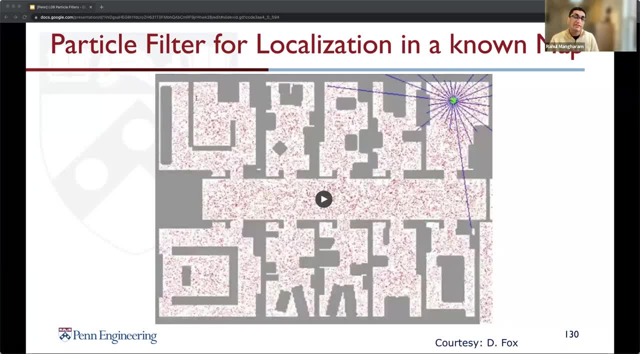 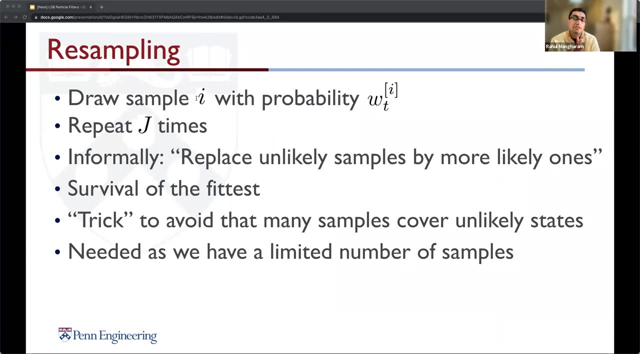 say that specific room, you can actually tell where you are in reality. That's a strong advantage of this particle filtering technique compared to things like Kalman filtering, which only has a single mode. In the resampling step we have our sample set with the weighted sample set. 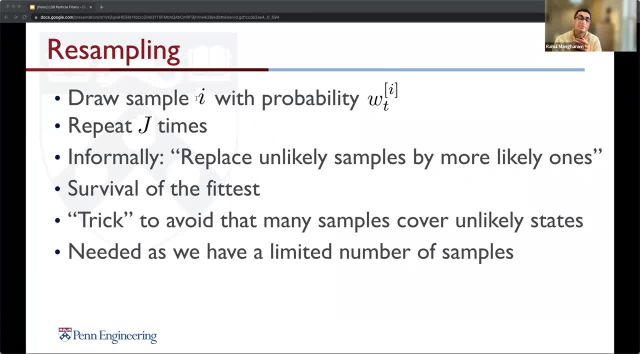 and then I just pick out n samples. I draw n samples with replacement, and the likelihood of drawing a sample is proportional to the weight. Why do I do a thing in the first place? Because I have a finite set of samples and with the finite set of samples you want to, 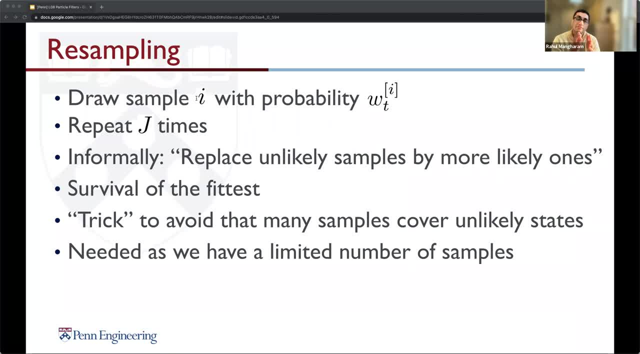 concentrate those samples in the region of the state space which substantially have a higher probability versus where they have a lower probability. If we happen to have an infinite number of samples, we don't care if a large number of samples is going to an unlikely region, as long as we have 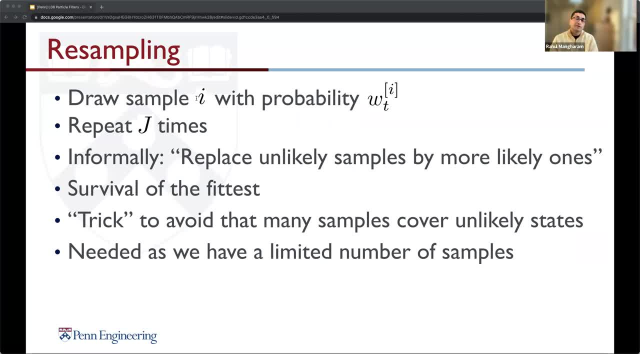 enough samples in the areas with high likelihood. But for all practical applications we only have a finite set of samples that we represent on our computer, and so we let the bad ones die out and use the samples to actually represent samples of the higher likelihood areas. So this kind of trick. 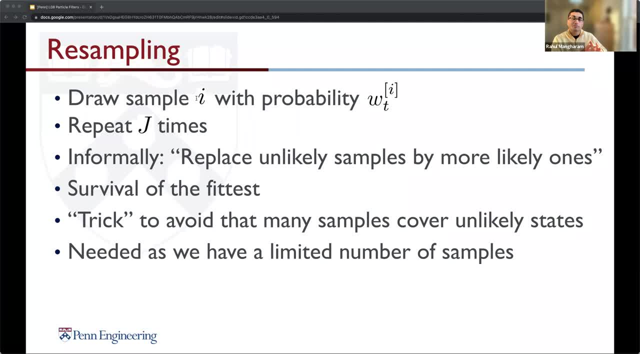 avoids what you have as a result of this trick. So this kind of trick avoids what you have as a lot of samples that are basically in zero probability areas. In practice, this resampling step is actually essential. So if you don't do this resampling step, you won't be able to track. 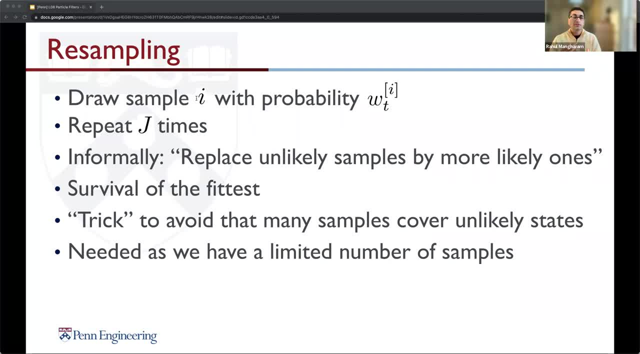 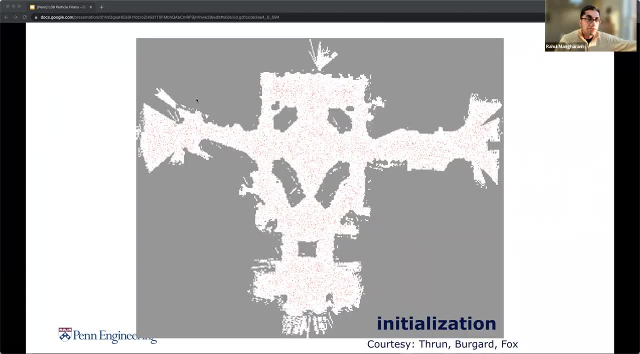 the pose of the system over long periods of time, because your filter will simply diverge. You won't have any samples, you know, which represent the likely areas. So here's a final example putting it all together: The demo actually is over 20 years old, from Carnegie Mellon. 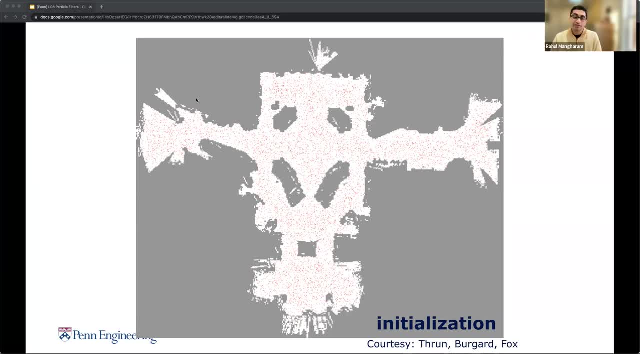 The demo actually is over 20 years old from Carnegie Mellon. The demo actually is over 20 years old from Carnegie Mellon, When the researchers were at Carnegie Mellon, and this is actually an example of when Monte Carlo localization was first developed. So this is a museum in Washington DC and what we see is the 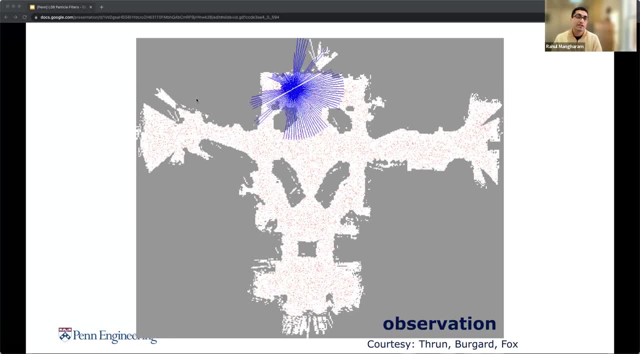 top view and we want to localize a robot in this world frame. The robot has two laser range scanners, one looking to the front and one looking to the back, and basically this gives us our first observation. I think there are over 10,000 particles. you know, at the initial stage, 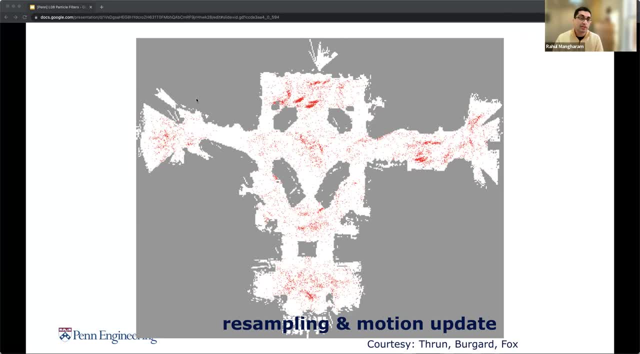 And then we do a resampling step and then a motion update, and then we take another measurement and then the weight is updated, The resampling is done, You can see how the particles have died out now and then the motion update is performed. So you can see from here that the motion update 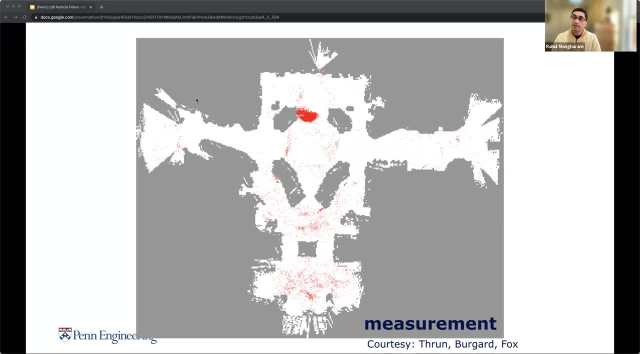 introduces some noise because there's some increased uncertainty and therefore the particles are spread out. and this comes from. you know the sampling procedure. And then again you take a measurement and do a weight update. So you see the samples you know are a lot darker in the areas of higher probability, where the robot is. And then you do. 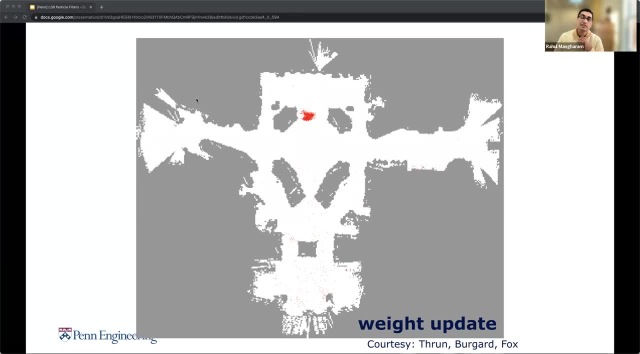 resampling and the unlikely- you know- states die out and it starts to concentrate. So in just a very few iterations we're able to get a really good, you know estimation of where our robot is, and you can actually continue this process and continue to localize the robot. 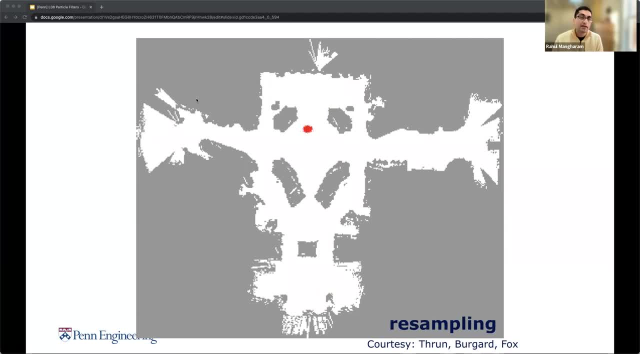 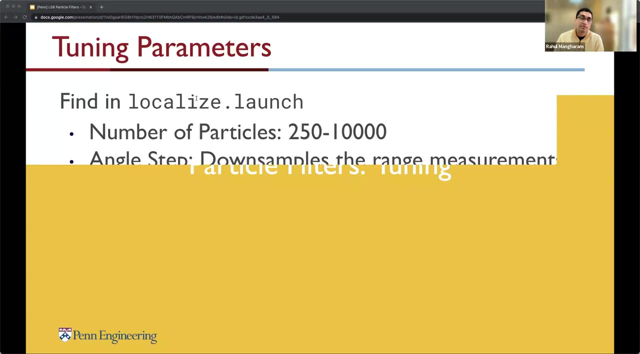 So this technique is called the Monte Carlo localization, and that's basically the gold standard for localization you know today. So we'll end with some practical ways of understanding the actual implementation of the particle filter. We tested on this briefly before, So obviously the one. 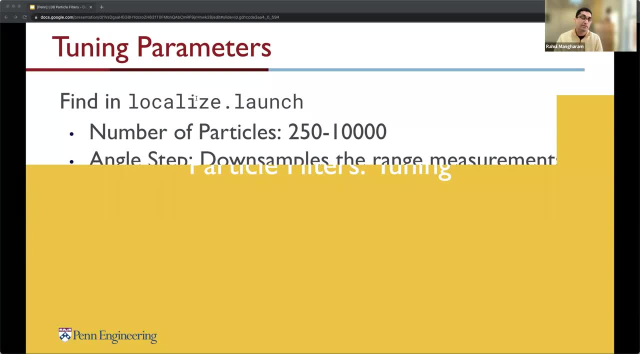 parameter that's really important is the number of particles. Now you can imagine if you have 10,000 particles. you would have to simulate in the possible range vectors of 10 000 times and then each of them would have thousands of rays. so it's heavy on computation. you also don't need to 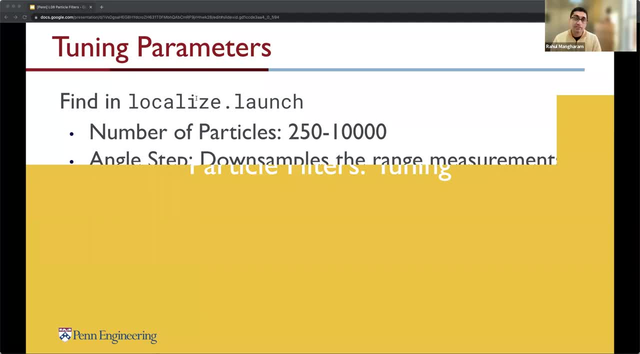 simulate all, like you know, 1080 lidar measurements from the dis, you know, from the discrete ray casting. perhaps you can down sample by a factor of four, or do the same for even the angle step. oh, the range of the lidar also influences your particle filter, because the longer you can see, the better shot you. 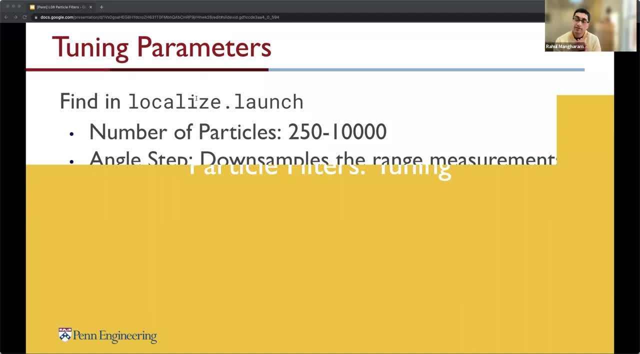 have about getting those unique correlations right. you know from the beginning, right? so if you have a 30 meter lidar, in general you know you start to localize much faster and and also uh, you maintain that estimate, uh, throughout. furthermore, you can get rid of the useless lidar measurements with. 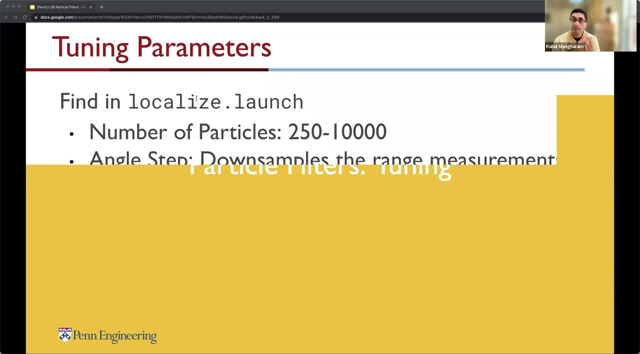 no returns or you know those hitting the floor that don't help you in the update step. so the particle filter can be set up actually to run in parallel on the gpu, as matrix multiplication is very compatible with running in parallel and that elevates. you know a good deal of the compute. 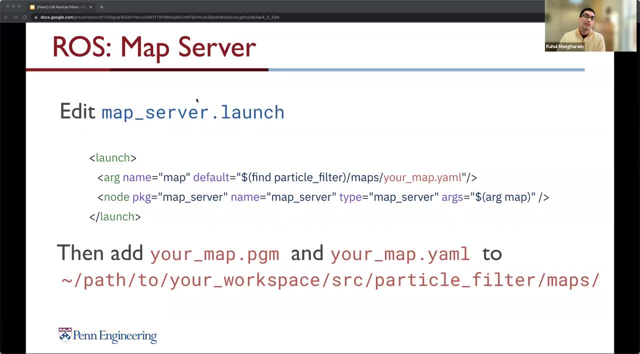 concerns using the particle filter. to run the particle filter or amcl, you have to give it a map file in our launch files so we send the parts through the map server and this map you know has to be a 2d cost map in the launch file of the particle filter algorithm. you need to 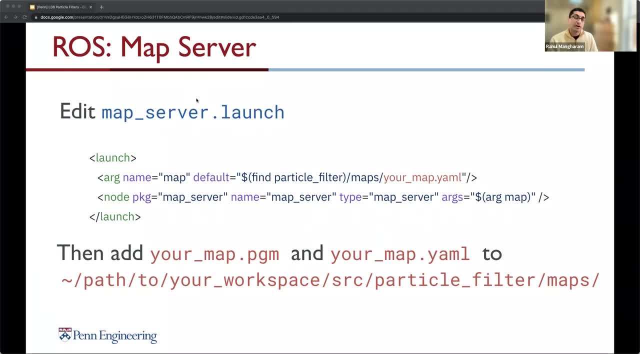 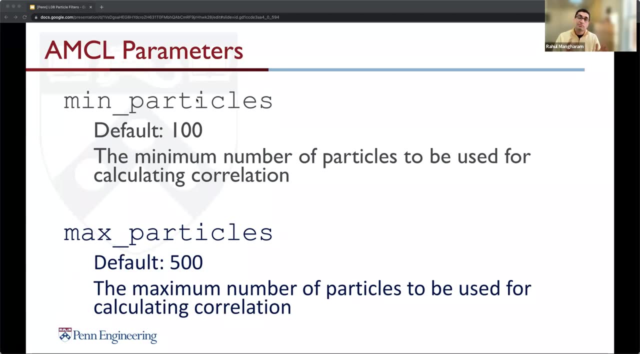 list where your map is, then this will open your rvis where you can specify your initial guess and then it will spawn the the filters to estimate the position of the robot in the map as it moves about some important parameters in the amcl package you know allows you to tune are the min: 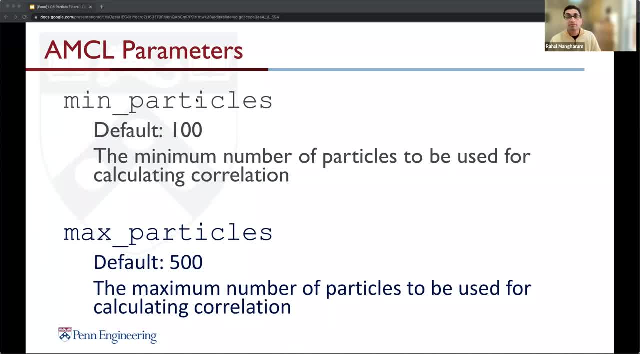 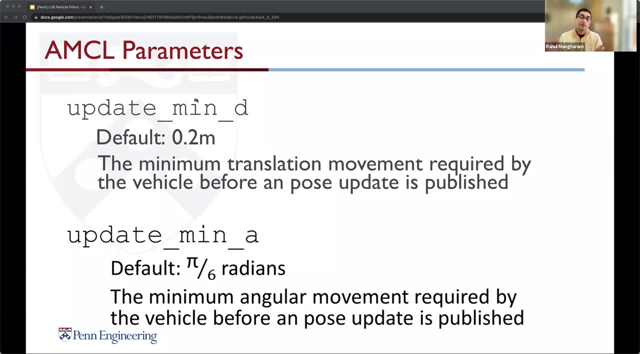 and max particle cloud size that kld sampling must adhere to. making it too high can reduce the update rate, and reducing it to few particles will affect the localization accuracy minimum distance and angle update parameters that we discussed before. you know decide how frequent you know to publish the corrected odometry drift. so, as you're moving, 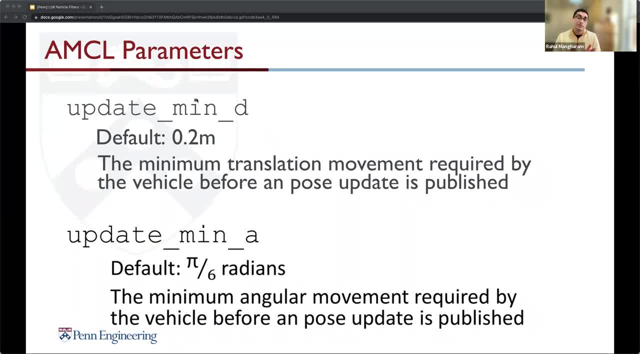 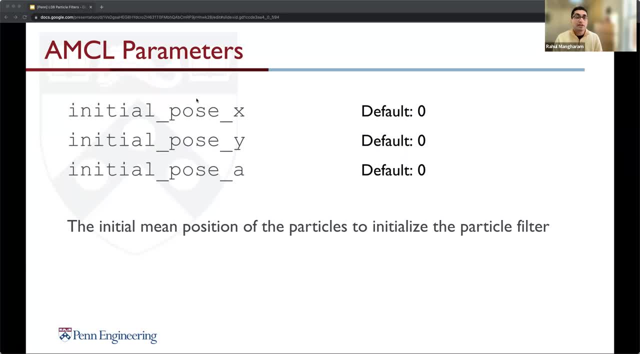 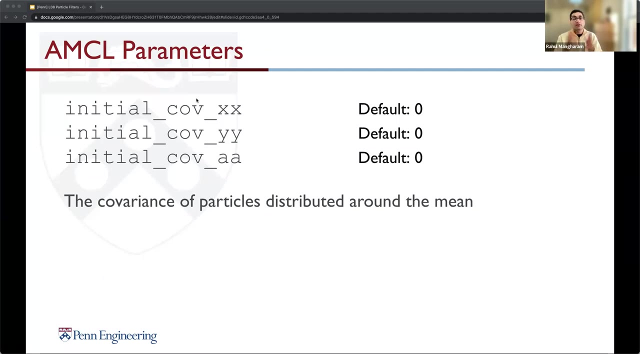 again, making it too small. uh, you know, provides bad localization due to insufficient samples. the initial pose gives the ability to programmatically define the starting position of the car and this can also be set manually, you know, through rvis. finally, the covariance of the gaussian distribution can also be set. this defines the spread of the particles around the mean. 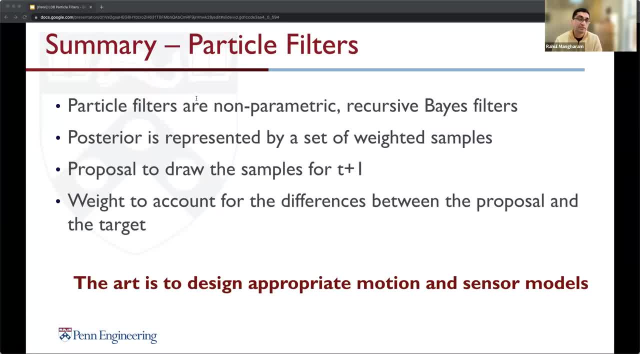 position. so, to sum up, particle filters. so what are particles? they are recursive, a base filter and especially a non-parametric variant. this means that we don't have a parametric distribution with which we can describe our posterior, but we use random samples to do that. we draw the samples. 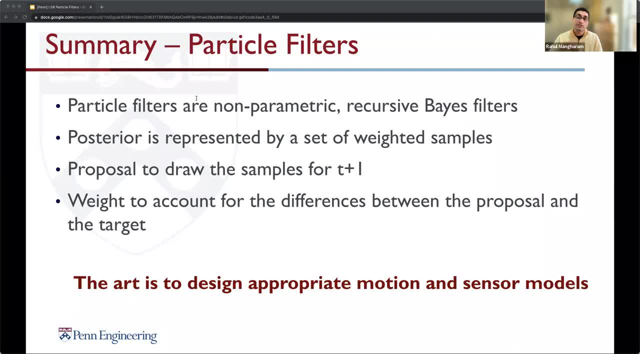 from a so-called proposal distribution in the next state, and then we do a correction in order to take into account the proposed distribution was not the target distribution that i'm trying to approximate- and then the final step is a resampling step and- and this is a technique which works very well, especially in